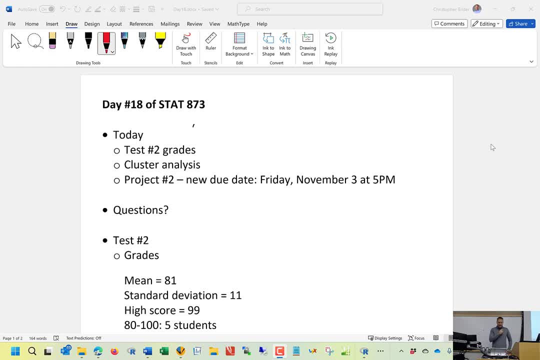 Let's get started here. So today we'll talk a little bit about test number two. We will continue with the cluster analysis section and, depending upon how far we get, we might talk a little bit more about project number two. Please note that I have changed the. 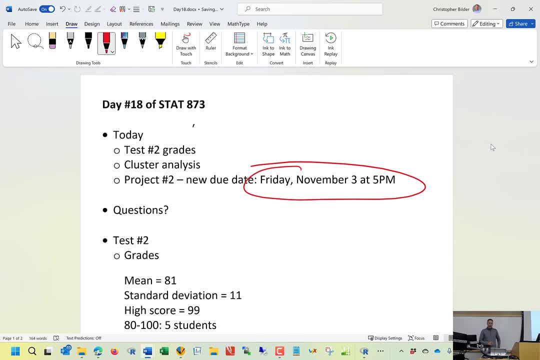 due date for project number two. So it's Friday, November 3rd at 5 pm. I was November 1st before. I'm not for sure if we'll get through as much material as I would like to in time for you to complete the project, so that's why I decided to move back. 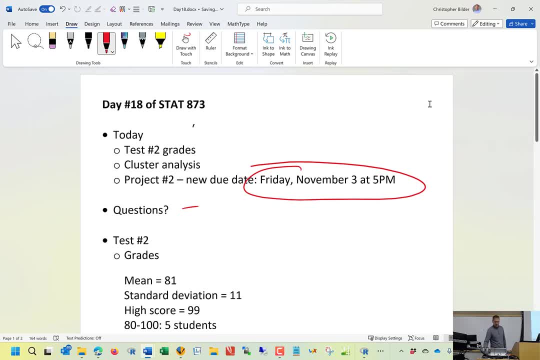 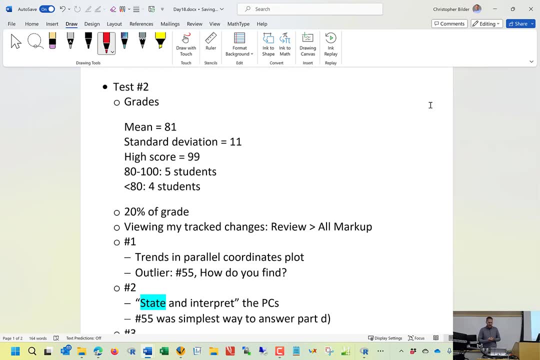 So are there any questions before we get going here? Okay, so test number two. Here's a grade distribution that I posted to the course website for the discussion board. Average score was 81.. Five students with a grade of above 80 percent or below. Now obviously there are some students here that probably are not. 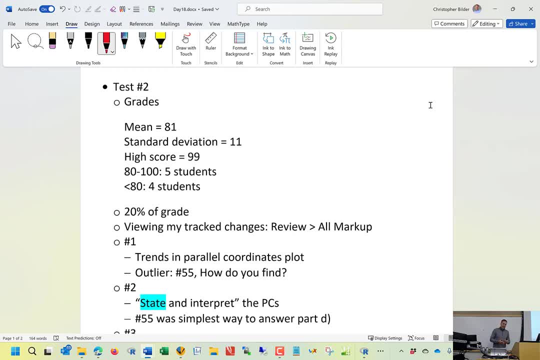 satisfied with their grades. Just realize that this test is 20 percent of your overall grade, That's not 100 percent. So you know there's still a lot of other grades that are out there that you can get to improve on your overall course grade. So please take that into account when you think. 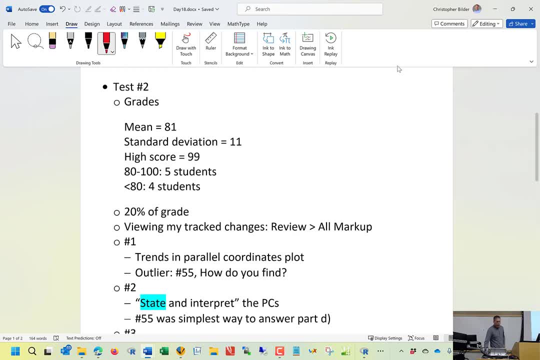 about your, your test grade. Hopefully, though, that this test- if you're not satisfied with your grade, this test- will give you an opportunity to think about: okay, am I preparing well enough for this class? You know what could I do better? And if you want to talk to me about it, 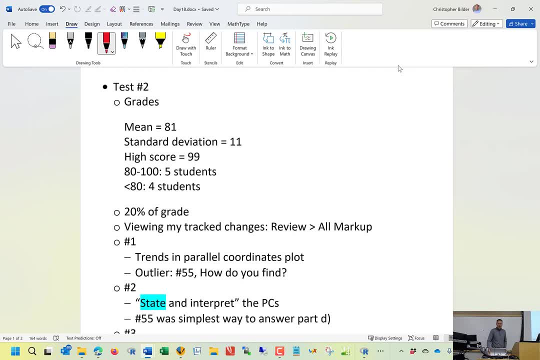 I'd be happy to give you some suggestions as well. So when you take a look at your test, please make sure that you have under review you have all markup checks So you can better see my comments that are on the test. 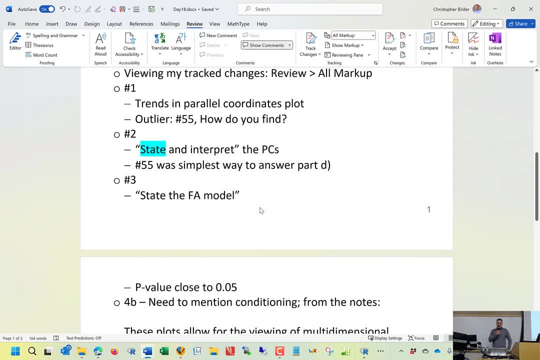 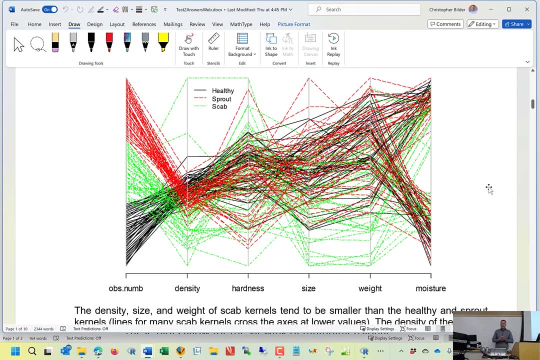 Let's go over some of the problems on the test. So number one: we had this parallel coordinates plot for the different kinds of weak kernels. Most students were able to get the get the plot right. Sometimes there was problems with the interpretation. Now, when I look at this plot, I immediately see that the 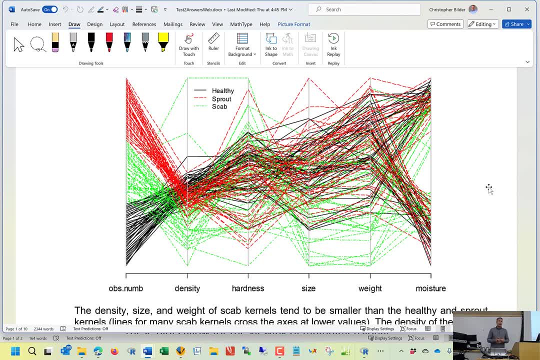 that there's a lot of green on the bottom of the plot, and so that's what i would immediately focus on: that it seems that these scab kernels tend to have low density, low size, low weight. but don't just focus necessarily on just, let's say, one of the variables. you know what we can see, one of the 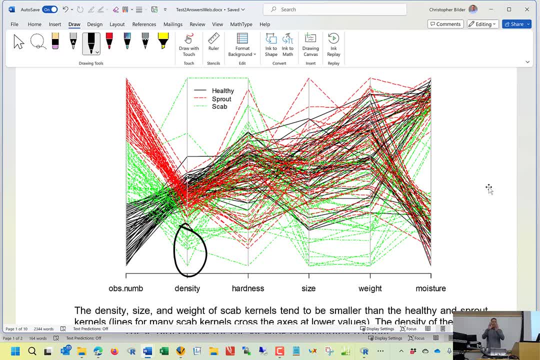 beautiful things about these parallel coordinate spots is that we can see trends across the variables. so, for example, we can easily see for size and weight that if i have a low size, i tend to have a low weight as well. so those are trends that i would focus on here. yeah, i might also talk. 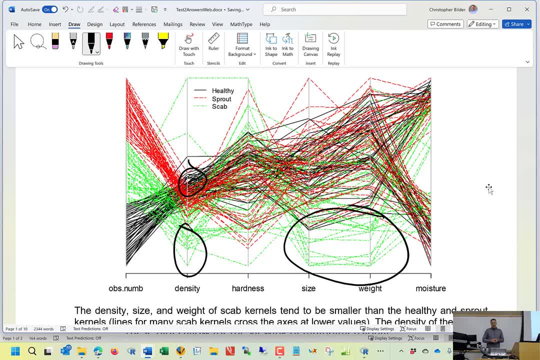 about how, uh, it seems like uh the healthy, uh kernels can tend to have a higher weight than uh the rest. that doesn't mean every single kernel is always, for healthy is always above sprout scab, but we're seeing these trends that it's. there's more of them that seem to be above. 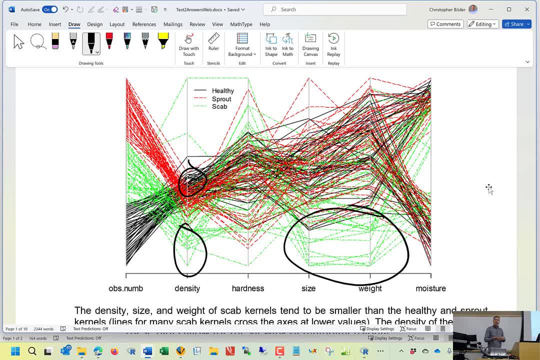 that, and so that's what i would talk about in this plot regarding trends now also later, then we need to start talking about outliers and the. the thing that i think that sticks out the most regarding an outlier is what i just circled there. you know by far. 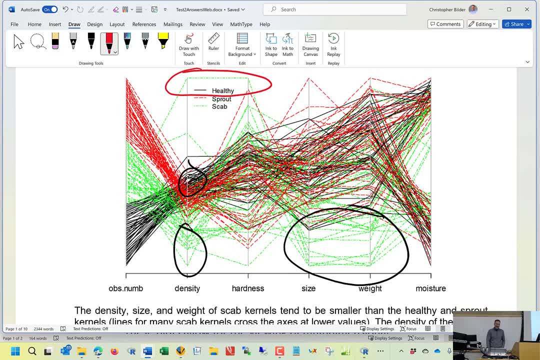 this one scab kernel has probably at least 25 percent higher um density than all the other curves and also tend to have the high. it also has the highest hardness as well, and so that's where i would focus on for outliers. now there are other possible outliers, you know we 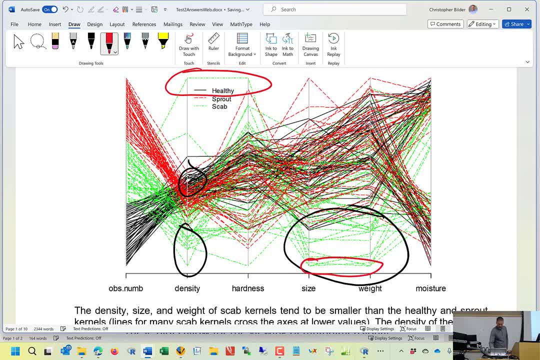 maybe these down here, this here, as well, as potential allies. we have this up here as well, and so there's multiple ways to answer the question, but you have to also justify your answer. in this particular problem, though, i let me just make sure i got the problem right. 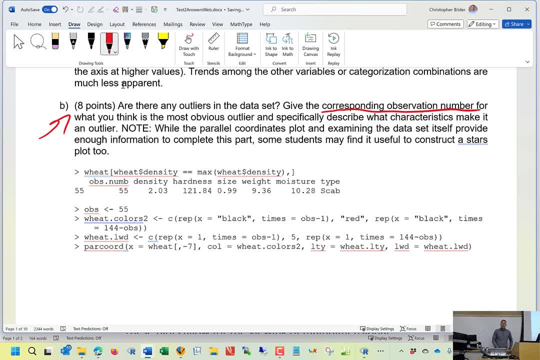 you need to give the corresponding observation number when you're talking about these outlets, and that's important because you want to determine well, which, which kernel in this case, is an actually an outlier? you know, it's nice to say, yeah, there's an outlier. well, what? what is the actual observation? 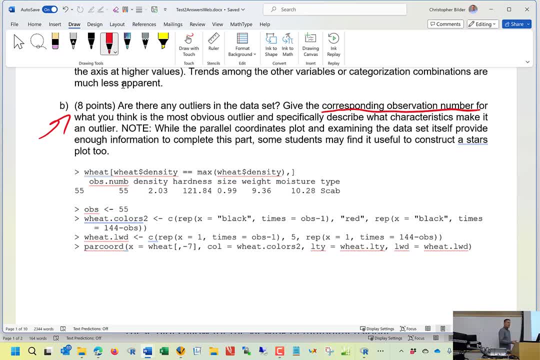 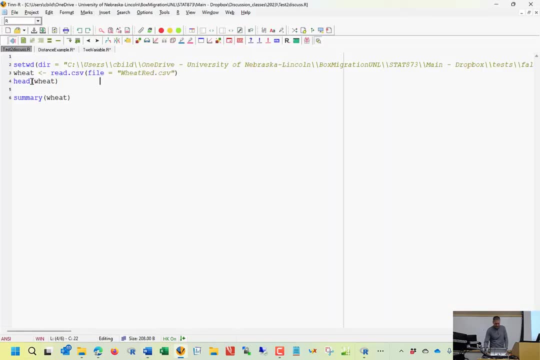 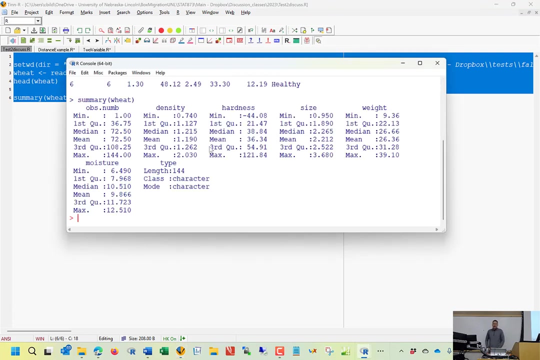 and so you need to actually identify that corresponding observation, and there's a number of different ways to do it. i show one particular way in the in the answer key here. another way that one could approach it is, let's say, you know, you're reading your data and you do a summary of the data. 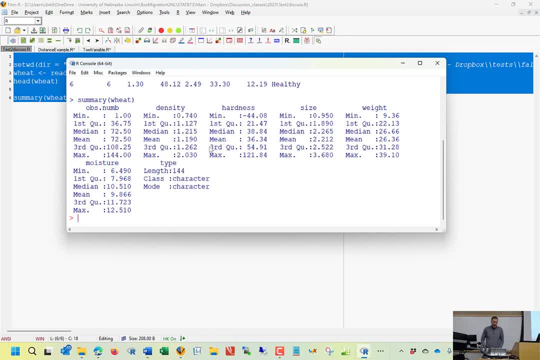 and you see, for density, the highest density is 2.03. so whatever observation number that corresponds to that's, that's the max, okay, so there's the 2.03 right there. so how would i again find then that particular observation number? well, how about we just simply look at all the density values? 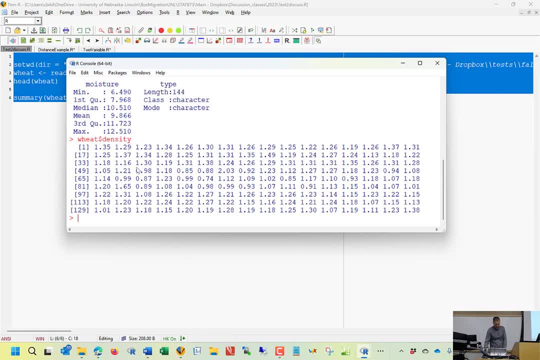 we find 2.03, and right here that corresponds to, if you count, number 55.. so that will be one way, probably the easiest way, to find well, what corresponds to that number. so that's the way to find your observation and where that is. and you know what i show, then you know i go a little bit farther. 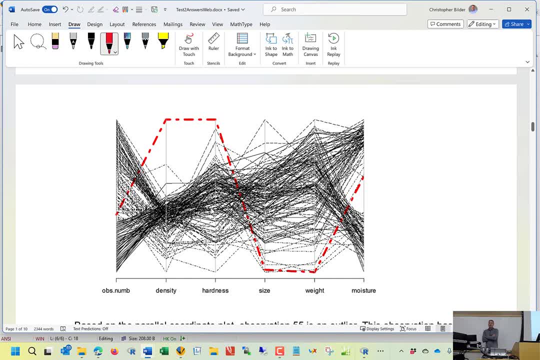 you know what i show then on this plot, then well, let's take a look at observation number 55. you're going to have to do this additional plot. it's helpful to do something like this in actual practice and we can see: not only is it the highest density and hardness, but it has about the small size. 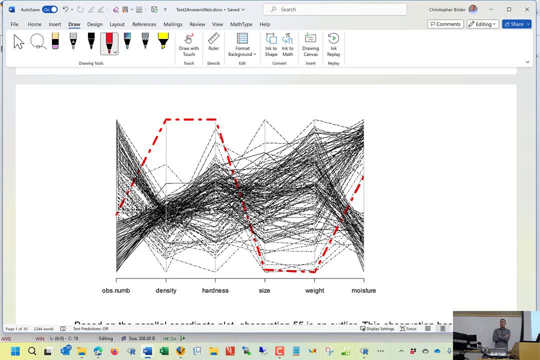 it has the smallest weight. so you know, this is multivariate, this is a multivariate course, multiple variables. we can see that definitely this particular observation is sticking out from all the rest. that's the definition of an outlet. now you could have, you know, again mentioned some of the other observations as outliers too. 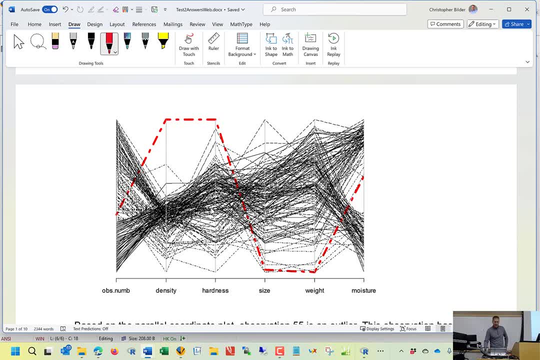 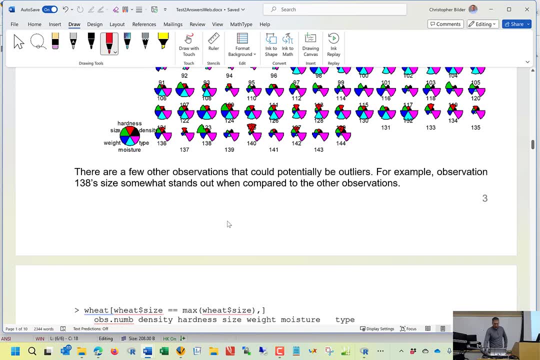 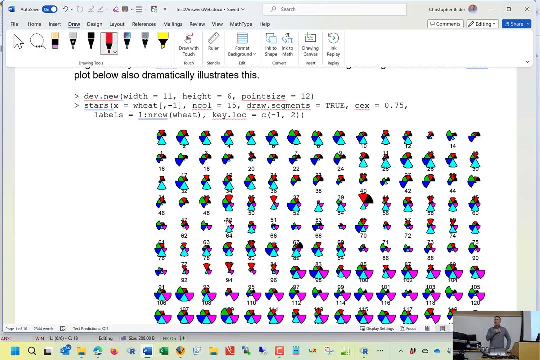 i wouldn't take all the points, but this is the one that really stuck out to me that i was hoping that you would see. alternatively, you know i mentioned in the in the problem description. well, you could also take a look at a star spot, and you know, if i just look through these star spot, 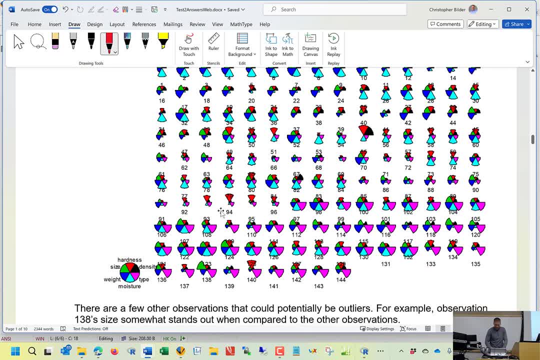 the one thing that just really sticks out is this one right here now, something that you have to be a little bit careful about in terms of how this labeling is done. this is actually for number 55, but unfortunately it's not going to be the same for all of them, so i'm going to go ahead and do that. 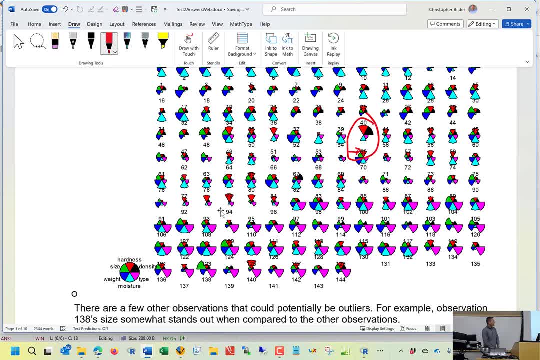 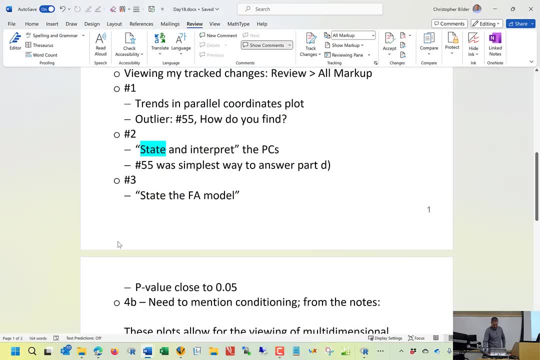 and i'm going to go ahead and do that, and it's going to be a little bit harder to see that number there because it's actually printed on the star spot right below it. okay, so number two. i think this is an example of sometimes, but we actually just saw one of these. 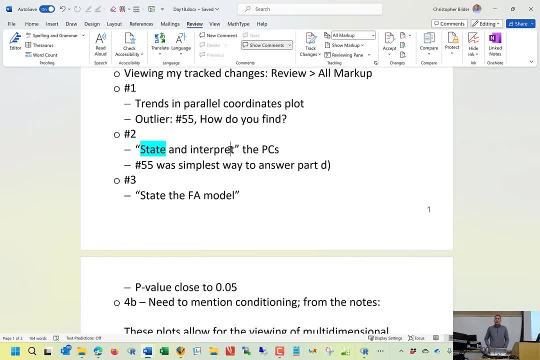 this is an example where you got to be careful you make sure you read the entire problem and look what the problem passed so you know previously for the outlier- sometimes students were missing- actually identifying what was the actual observation number in number two. the first part said: state and interpret the corresponding principal components. 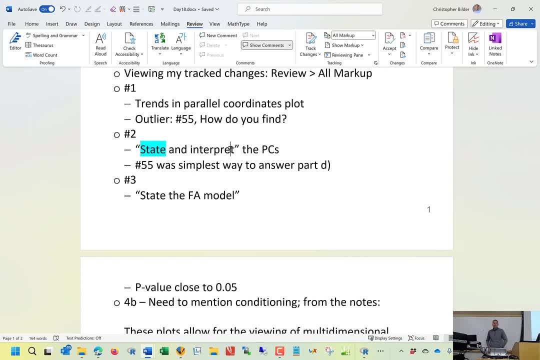 sometimes students would miss the state part. sometimes a few, maybe one or two students missed the interpret part. they got stated meaning an actual state part sometimes, sometimes nervous and for the most part as long thinking heavily in all of the information asks you what we sure thought it. might score for this problem. but talking in practice was a good start to figure out that i was missing out. but there's a colloquial pricing for the relation from student hands at, or students headings and size set and i'm probably not that discretenced… and later i gotzen necessary produce in sense of how these 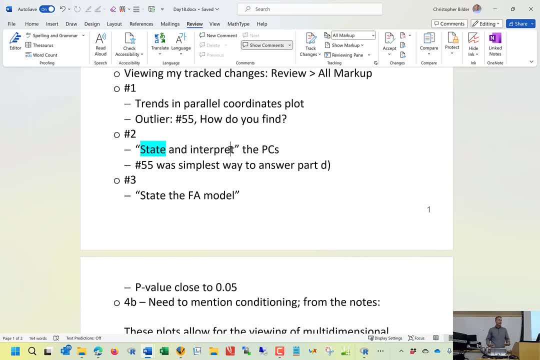 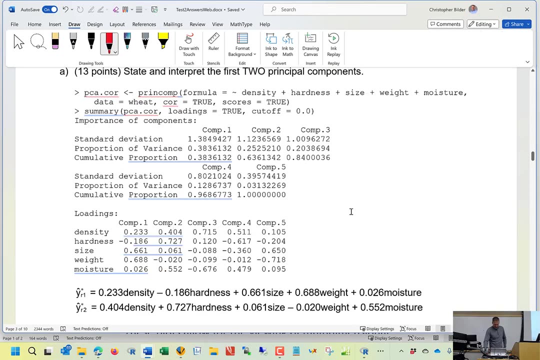 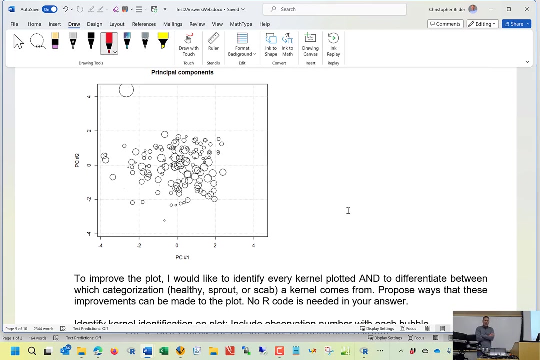 write out the equation and then interpret, and so unfortunately then some easy points were missed there, because the whole problem wasn't wasn't answered, but in number two. here see, so I had this plot of the principal components that I gave it. obviously one thing really sticks out compared to everything else. 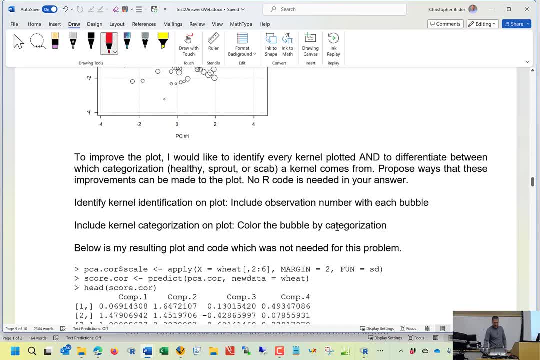 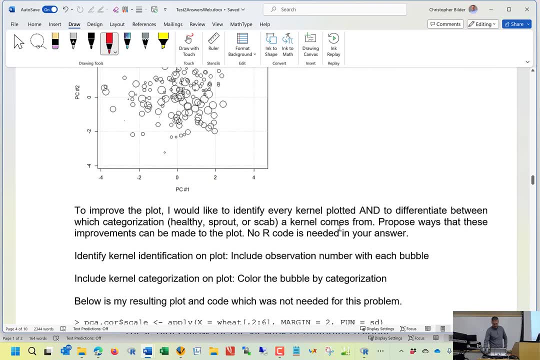 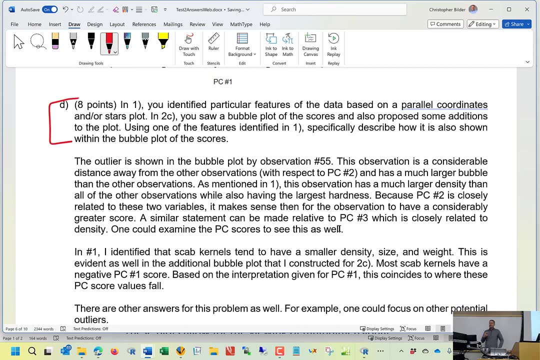 and in this particular problem I ask: basically identify a feature of this plot that can also be seen in a parallelogram, coordinates plot in number one, and I really, really like this problem because it helps you make connections between the different kinds of plots that we've. 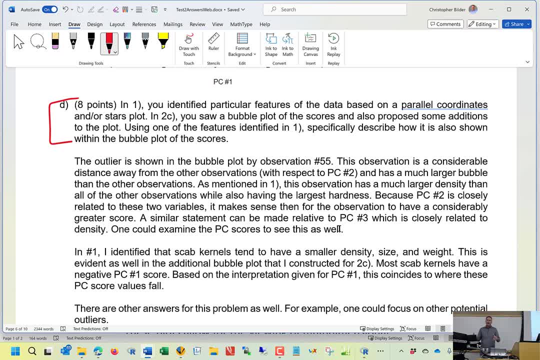 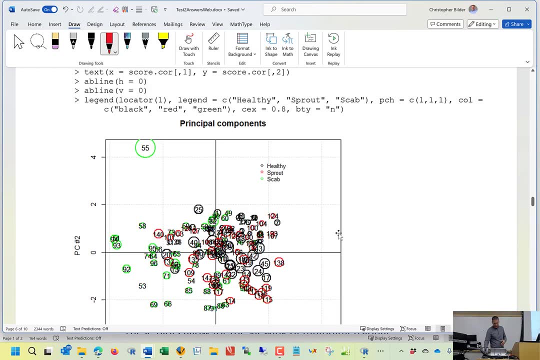 talked about- I mean, even when we talked about the group in the graphic section- the connections of between plots and eventually then the principal component section. we try to make those connections, and so that's what I was trying to assess there, if you can make those kind of connections. and so with this plot, 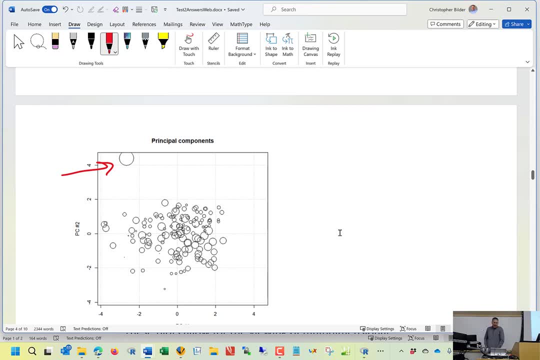 here again, that feature that I have arrow pointed to really stands out, and so you might be thinking: okay, well, how? how? if something stands out that much, how can that be represented in the parallel coordinates plot? well then, that gets into understanding. this has a large um Principal component, number two value: 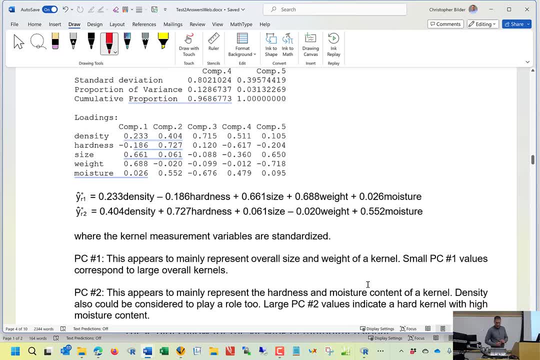 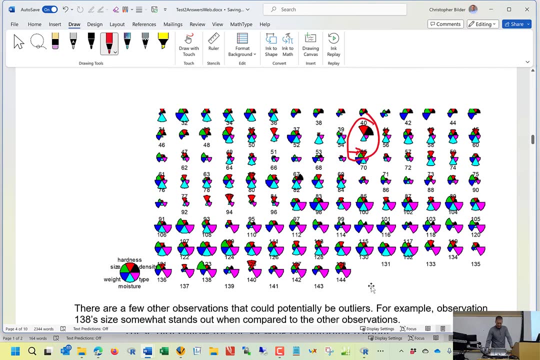 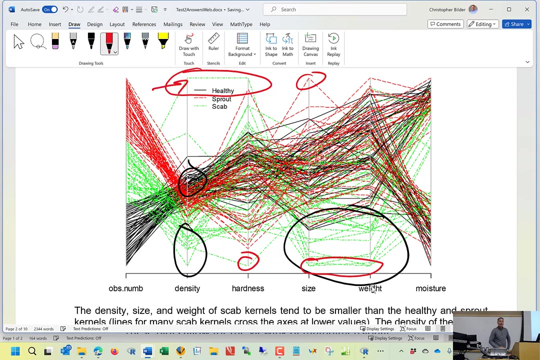 So, principal component number two, In order for it to have a large value, we need to have a large density. I need to have a large hardness. Okay, This particular value has a large density, has a large hardness, And so that's what you could have focused on. 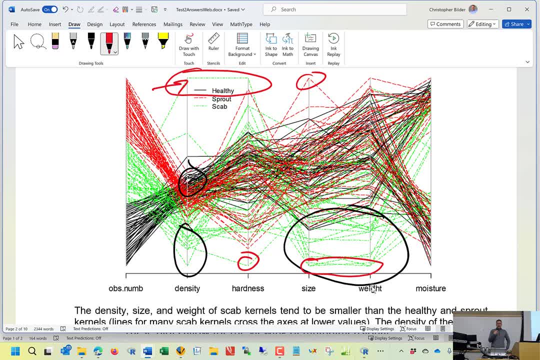 in this particular plot to talk about. I saw them, it was an outline, it was a density, Hard, very large density, very large hardness, And I see it in this principal component, number two. So that would have been the easiest way. 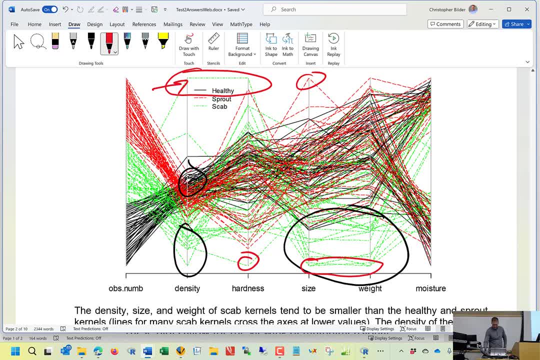 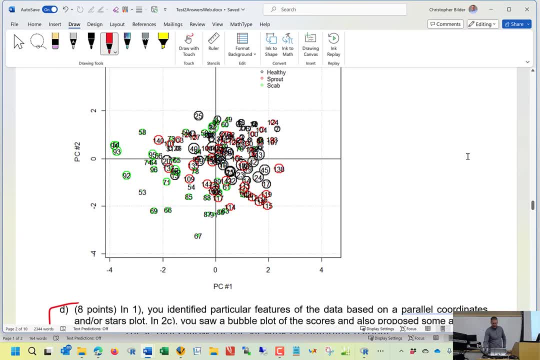 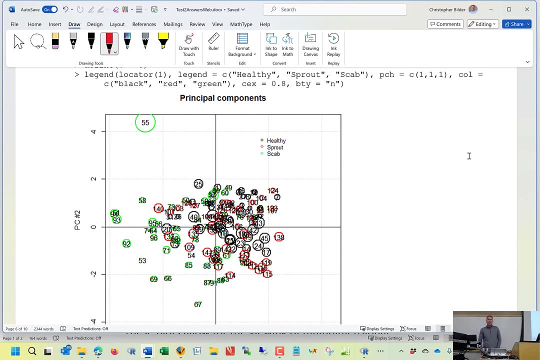 to answer that problem, And while it wasn't needed, some students decided to go ahead and do one of these plots as well, And one thing that you can talk about in this particular plot is that notice the green there for the scab. 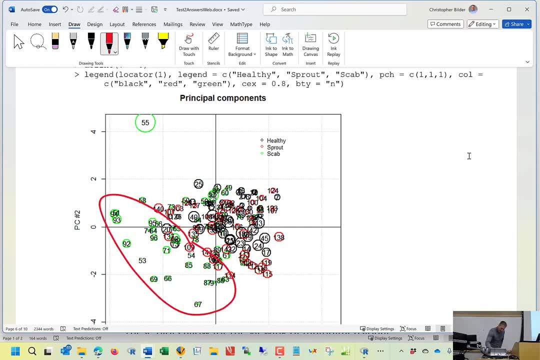 Notice how that kind of is separated to some respect from the rest. Well, that corresponds to what we saw for the parallel hardness plot with respect to the density- density and two of the other variables as well, And so you could have talked about that. 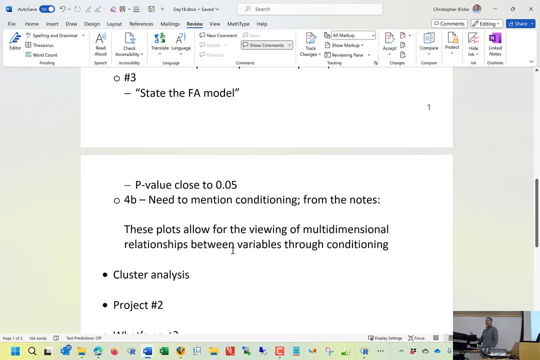 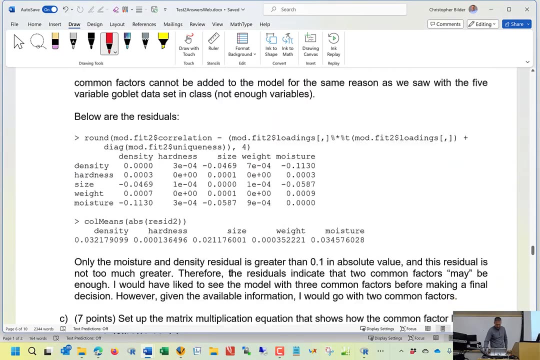 Number three was the factor analysis problem. Again, you gotta state the factor analysis model, And some students do not do that. But let's talk about how to decide on the number of principal components. So are two common factors appropriate to use with this data? 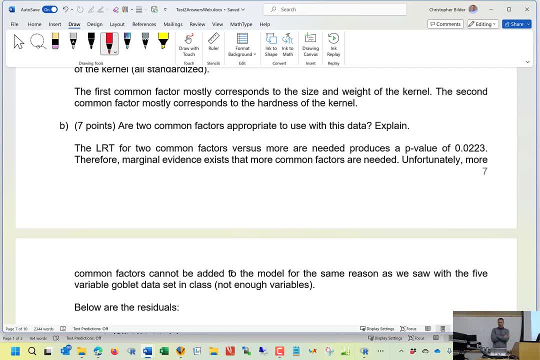 Some students- and this is what I would start off with as well, but some students chose to start off with the likelihood ratio test. Some students chose not even to do a likelihood ratio test, But start off with the likelihood ratio test. That's a great place to start. 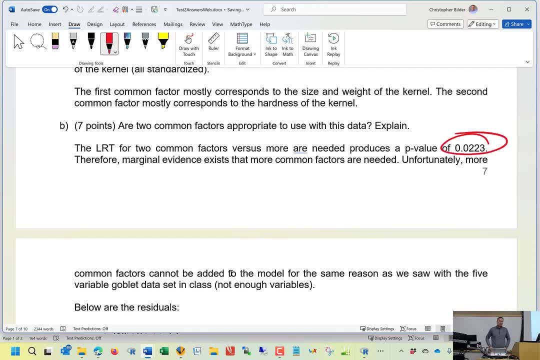 Let's take a look at this p-value. So the null hypothesis is that two common factors are sufficient. The alternative hypothesis is that you need more And that's kind of a low p-value. And so from that you would say, well, I'm a little worried. 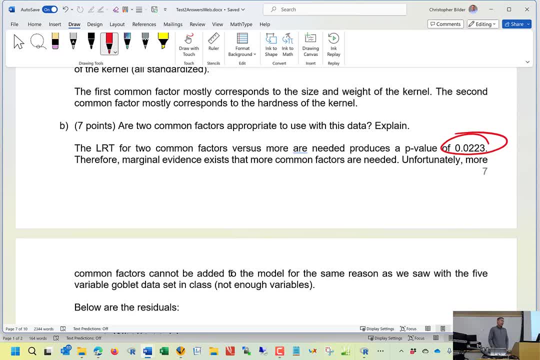 that maybe two factors are not sufficient. I mean, it's a borderline. You know, if I had .05 as my alpha, two would not be sufficient. If I had alpha .01, then you know you would say, don't reject HO. and perhaps two are okay. 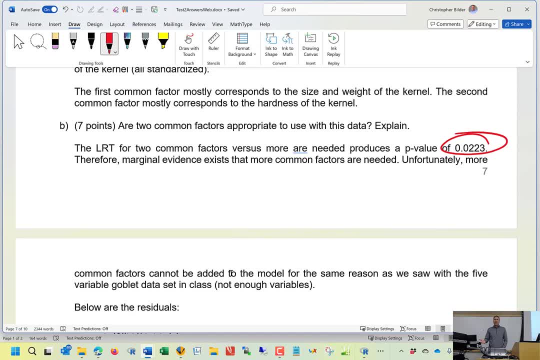 But you at least have to go through that logic. And if you immediately say two factors are sufficient because the p-value is .02, and leave it at that, you did get full credit, Because someone again could use alpha .05.. 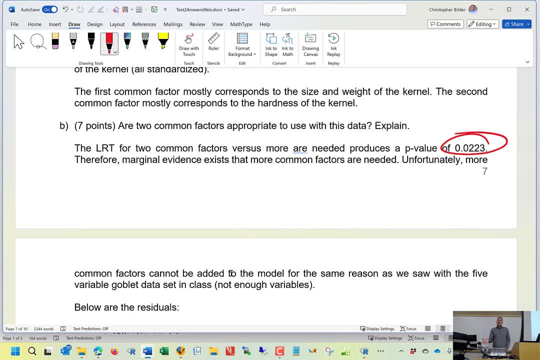 And you would reject HO. Now, if you talk to, let me start talking about. you know that there's marginal evidence that helped you get more credit, But you know we have other tools available to us to make a judgment. 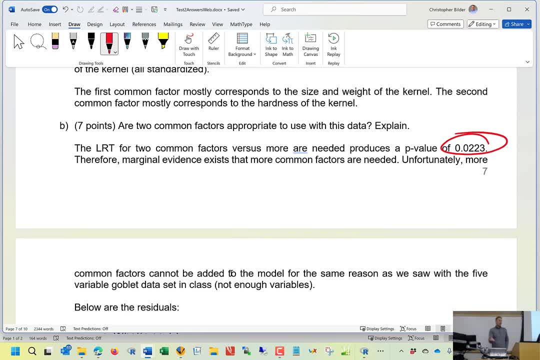 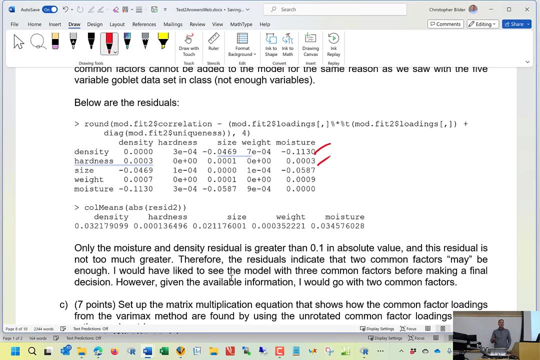 And so since I have kind of a borderline decision here with this like the ratio test, I definitely would want to look at something else: The residuals. And if you look at the residuals you know we have just two that are a little bit larger. 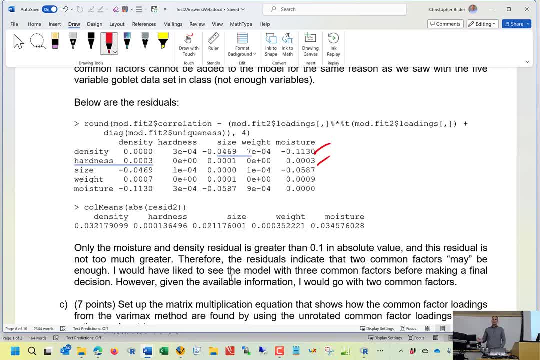 in absolute value than what we would like, But they're not too much larger, And so with that I could probably, or I could justify: yeah, okay, two factors, two common factors, probably will work fine, It's not perfect though. 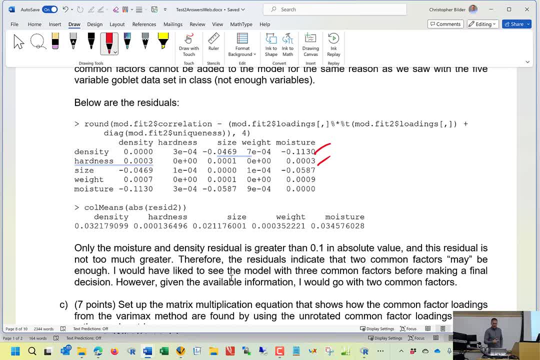 And so that you know that's. you know that's a little bit of a. you know that's a little bit of a. you know that's a little bit of a. you know that's what I was looking for in that particular problem. 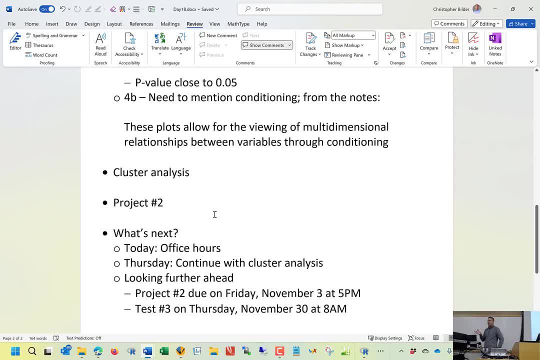 And then, lastly, 4b, Let's talk about trellis plots. What about trellis plots? allows us to have to plot multivariate data, And the answer actually came from essentially the right, when trellis plots were introduced in the notes. 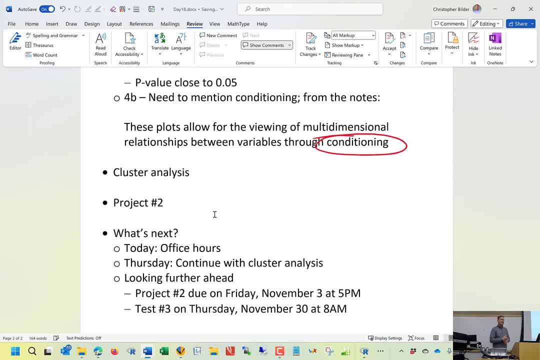 And the key is: you need to say something about conditioning. Trellis plots allow you to condition on particular values of our variables so that then we can look at the relationships between some of the other variables. That's the key with these trellis plots. 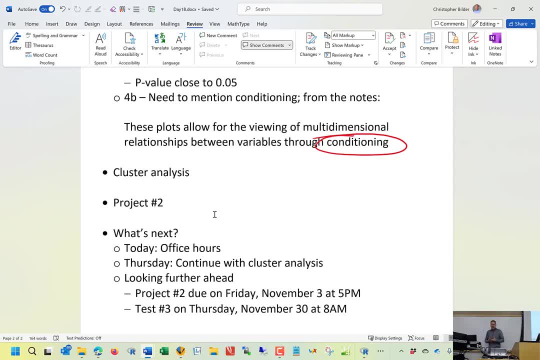 the conditioning aspect. Okay, So that's all I had to say specifically about the tests. Now, if you have a question, you know, about why I took off a certain number of points on your test. you know that's okay. 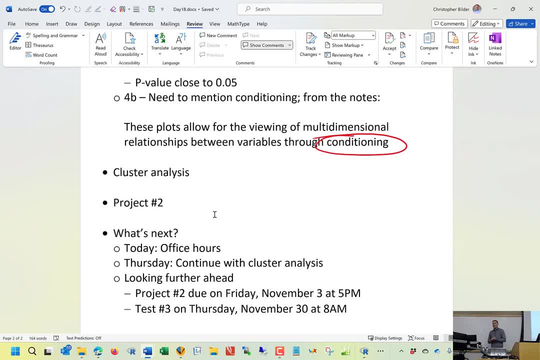 Please ask me that individually after class. I'd be happy to talk to you about it. If you have a question, though, about how to do a particular problem on the test, after you, take a look at the answer key if you still have a question about it. 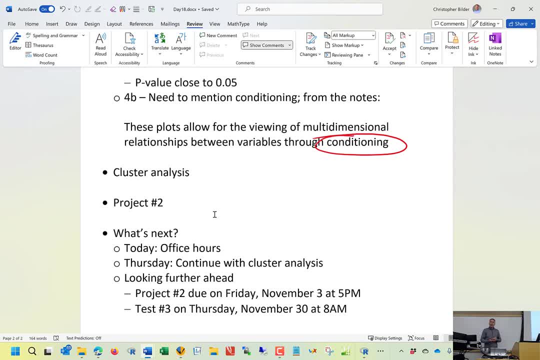 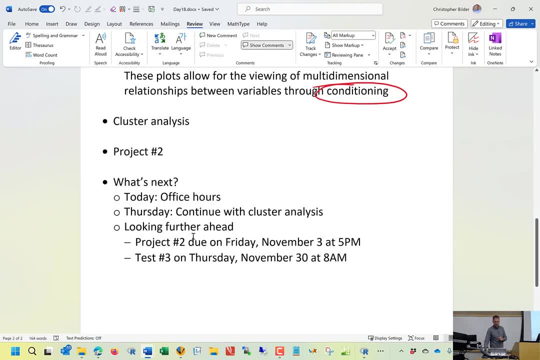 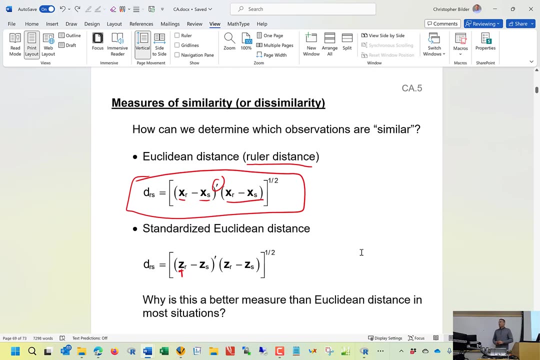 please feel free to ask at this time. Were there any questions about how to do particular problems on the test? Okay, Let's move on to cluster analysis again. So the purpose of the cluster analysis is to basically have a formal way to group observations. 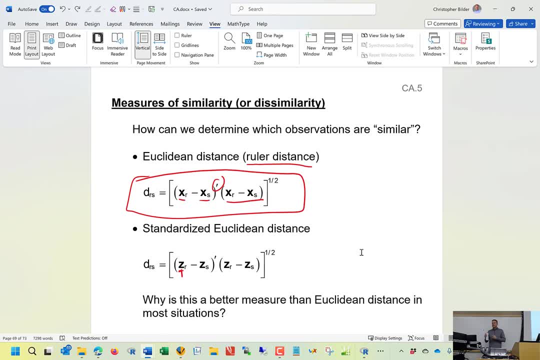 And these observations aren't grouped in any previous way that you know about. So, for example, like with the goblet data, We don't have a based upon the information that we've collected, we don't have a grouping, But, as you will see eventually, 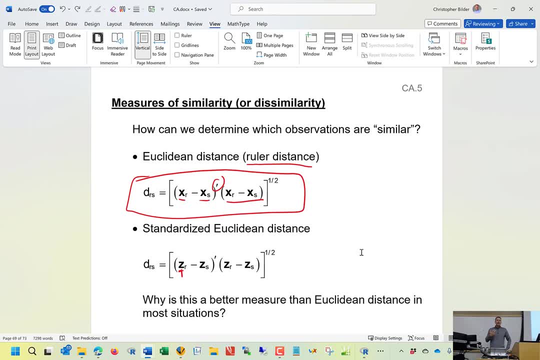 we want to come up with some kind of grouping. This grouping is called a cluster, So a group is a cluster. It's just a name that has developed over time, And so you know how do we make decisions about what observations to put in the same cluster. 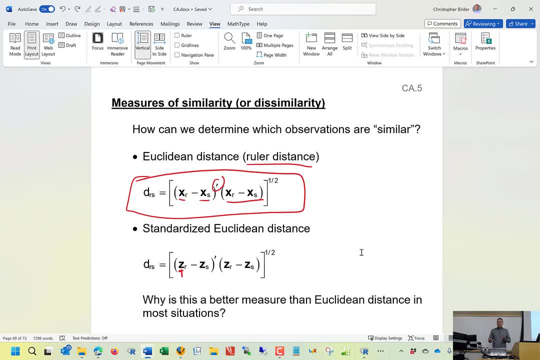 And so you would think that, well, it has something to do with some observations being, let's say, similar to one another, Okay, Or dissimilar. You know, the ones that are similar you're going to put together in the same cluster. 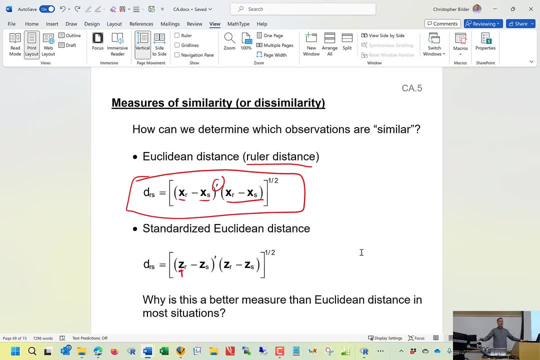 The ones that are dissimilar. you're going to keep them the same. So how do we measure similarity? There's actually a number of different measures. We're going to talk about just the most widely used ones, And that is Euclidean distance. 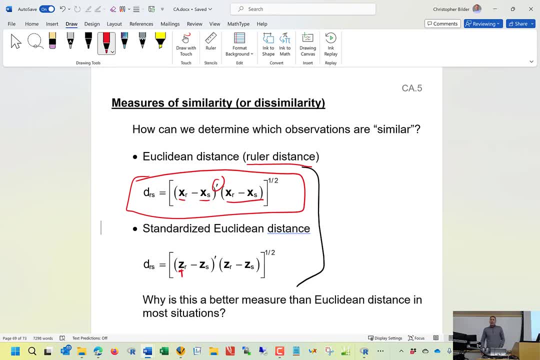 So you can think of this. you know, if we have just simply two variables, And that's Euclidean distance, And we plot data in a scatter plot, If we just actually put a ruler down on the plot, Essentially that's the Euclidean distance. 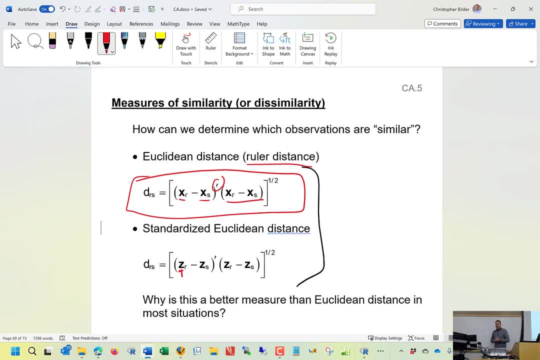 if the ruler is properly scaled And so we can do the Euclidean distance just with the regular data or with the standardized data, And almost every application people will be using the standardized data. The reason why? Because it's just the Fen freezing. 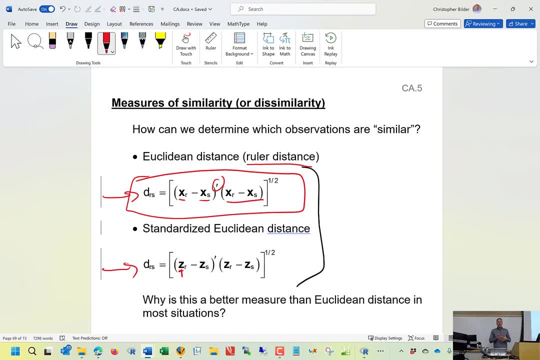 The reason being is because you don't want, let's say, some variables that are measured in a different numerical scale than other variables to have an actual effect on what you say is similar or not. There are some special cases where you still want to use just plain old Euclidean distance. 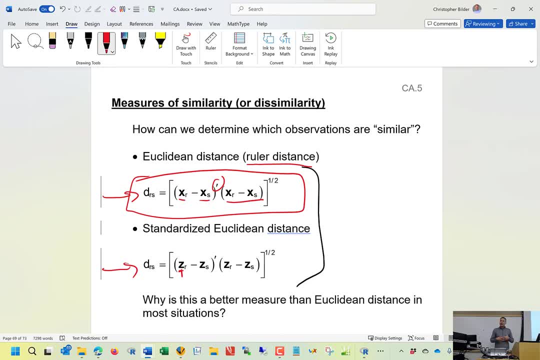 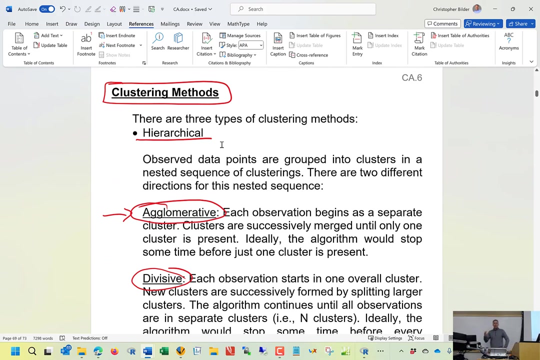 but generally speaking, most people use standardized Euclidean distance to take out the fact that some variables are measured on different scales. Once we have this way of measuring how similar observations are, then we can use one of a wide variety of different cluster analysis methods to put the observations into groups. 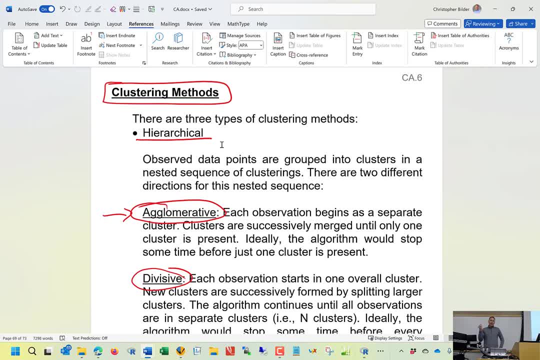 into the clusters. There are three main different, let's say, categorizations of cluster analysis methods. Today we are going to focus on what's called hierarchical, and hierarchical is split up into two different parts. Today we are going to focus on agglomerative, where the basic idea is this: 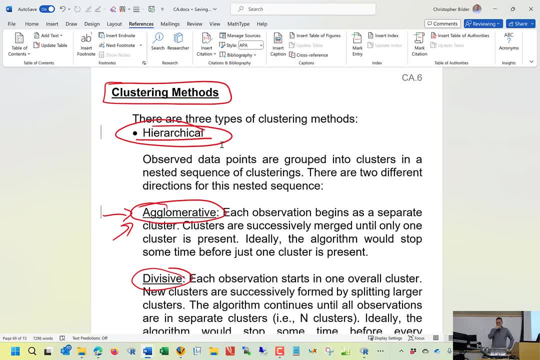 Every observation. the process to find these clusters is hierarchical, meaning that there is a number of steps involved to determine what observation goes into what cluster In an agglomerative method. what we do is we assume, let's say, if I have ten observations, 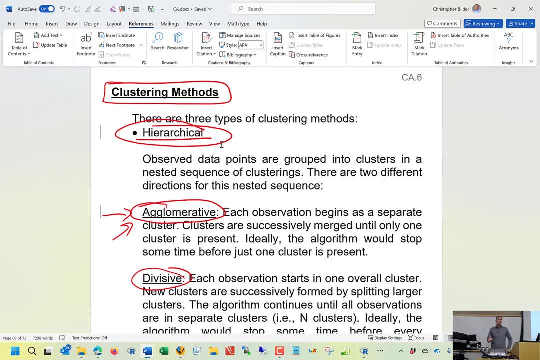 I'm going to start off with ten clusters- Every observation is its own cluster- And then what I'm going to do is I'm going to look for the two, let's say, clusters that are most similar, and then I'm going to merge those two clusters together to form a new. 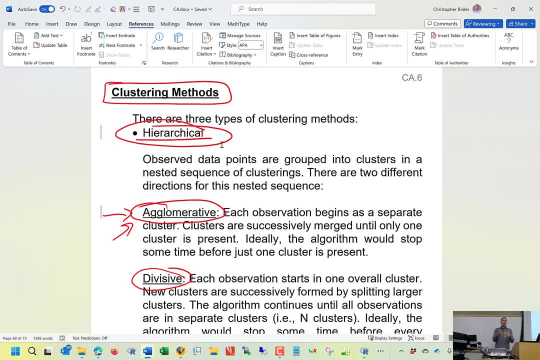 cluster. So now I have- if I start off with ten observations- ten clusters. now I'm going to have nine clusters. Then what I'm going to do is based upon these nine clusters. look at the number of clusters that I have. 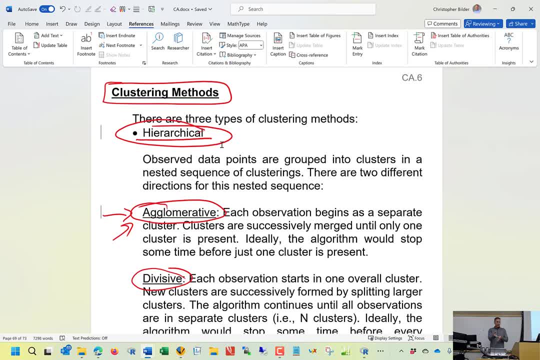 I'm going to start off with the ones that are most similar to one another, using some kind of measure like a variation, actually, of the Euclidean distance, And I'm going to put those two clusters together to form a new cluster. so now I could have. 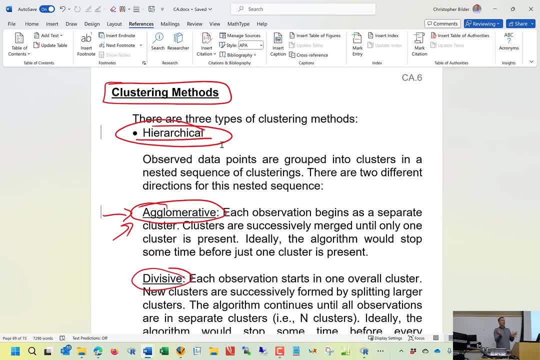 just eight clusters. Now I'm going to keep on going in this process until all the observations are in just one overall cluster. You might be thinking: wait a second, why would we want to have just one cluster? Well, one of the big things that we're going to be considering is that we're going to have 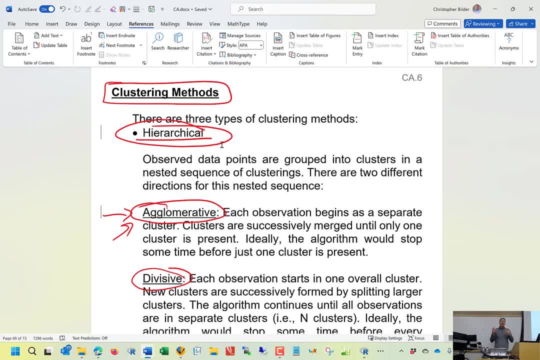 to keep on going. One of the big things that we're going to be talking about is: how do I make a decision about where to stop the clustering process. Maybe once I get to three clusters, I want to stop. Maybe I get to five, I want to stop. 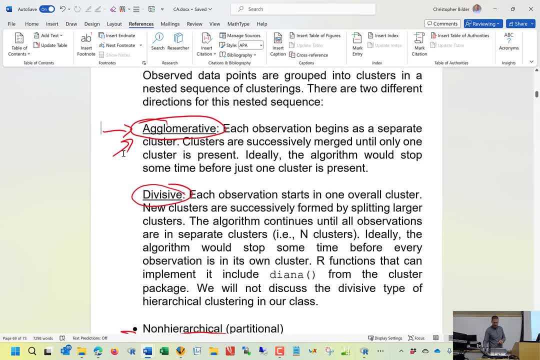 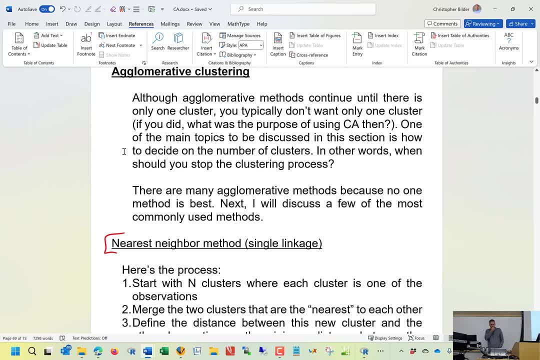 How do I make that decision? That's what we're going to be talking about. So now we're going to get to new materials. Let's create a new material. Let's create a new material. Let's create a new element. Let's create a new element. 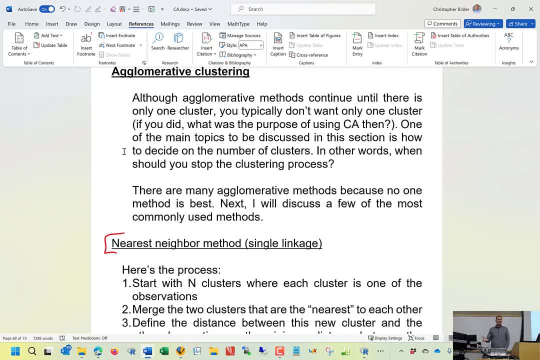 Let's create a new element: the agglomerative clustering. there's actually a number of different ways to actually implement it. we're going to talk about a few of them. why are we talking about a few rather than just focusing on the best? because there is no. 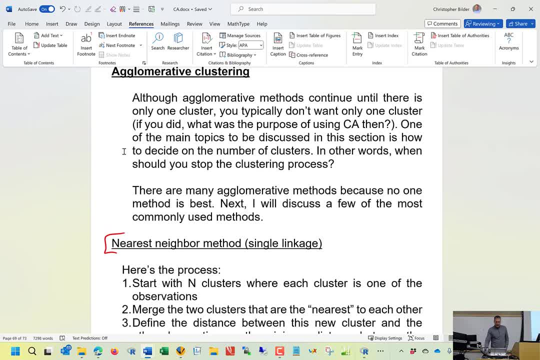 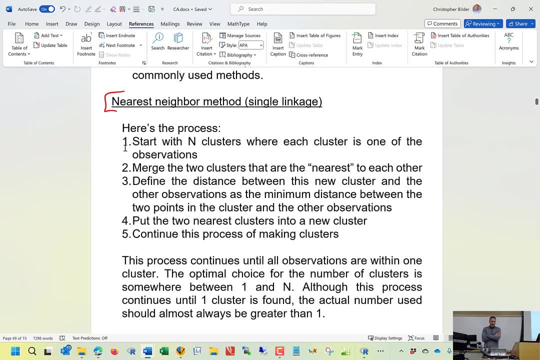 best method, and so we're going to begin with what's called the nearest neighbor method, also referred to as single linkage by some people. and here's the process, kind of similar to what I just described. let's say, I have n observations. every observation is going to be a cluster, so clusters of size 1. 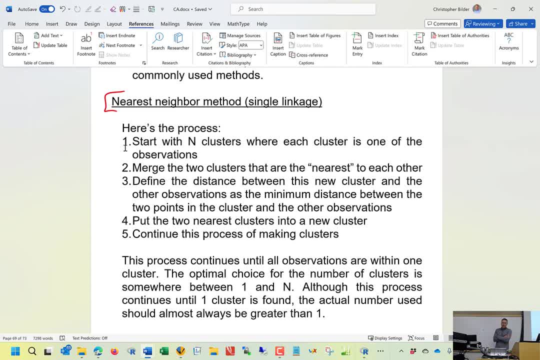 then I'm going to merge the two clusters together that are the nearest to one another- good, and in the end it's just simply well, which have the smallest standardized Euclidean distance then. so I have two observations that are in a cluster. then I'm going to need to somehow then make a decision about, well, what's going to be. 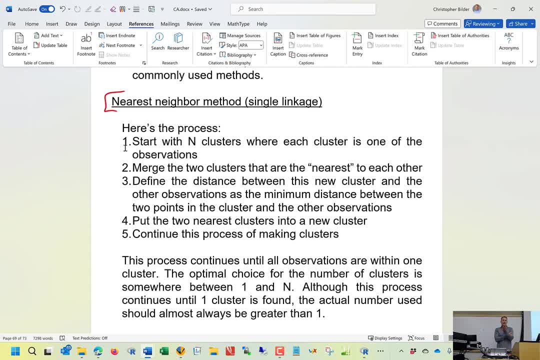 merged next, and the key is that: how do you make a decision about? how do I measure, then, the distance between this cluster that has two observations? how do I measure that distance that cluster is from the other observations? how do I do that? in the way that this is done- and we'll go through a 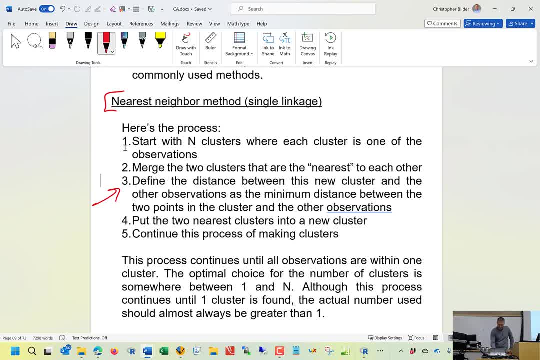 simple example shortly define the distance between this new cluster in the other observations is the minimum distance between the two points and the the cluster and the other observations. So now I have all these distances again and I need to decide. okay, well, I need to now merge a set of 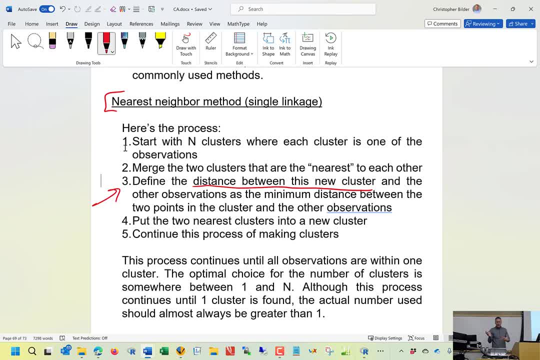 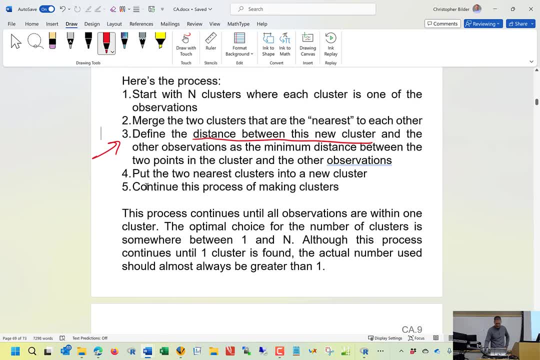 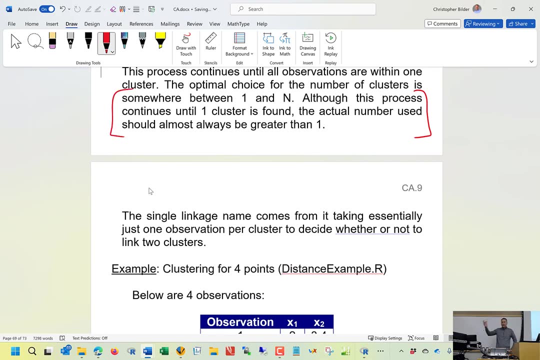 clusters again, And so I put the two nearest clusters now into a new cluster And I continue this process until everything is in one cluster. But the key is at some point and we'll get to it eventually. today I'm going to need to. 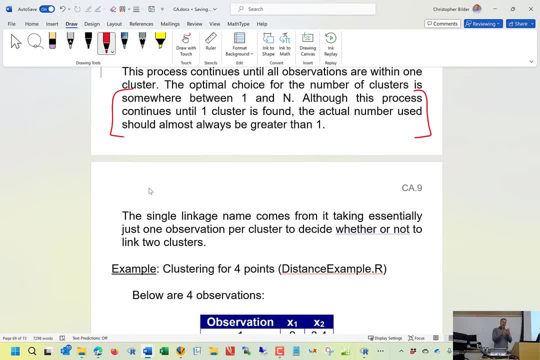 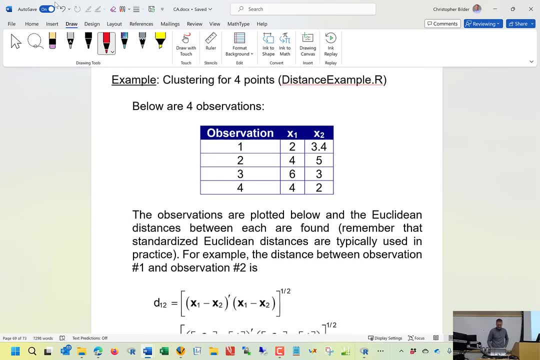 figure out. okay, I don't actually want to go to just one cluster, I want to stop somewhere before that. So here's the example. I have simply four observations and only two variables. It's an easy example to help illustrate this. And we're just going to use regular old Euclidean distance. We're not going to. 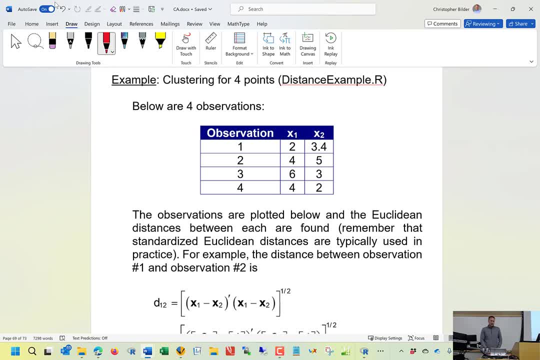 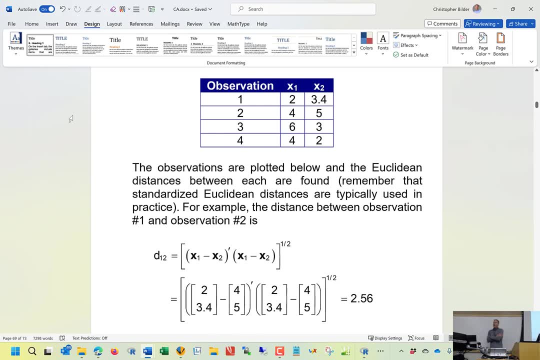 use standardized Euclidean distance here. So what I need to do to begin with is find all possible distances between each of the observations. So, for example, if I want to do observation one and observation two, which equivalently we can think of as, at least right now, cluster one, cluster two, I can find my 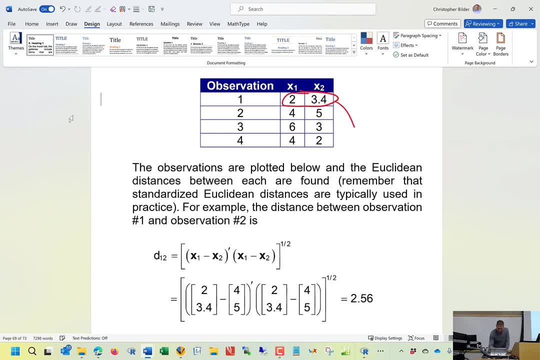 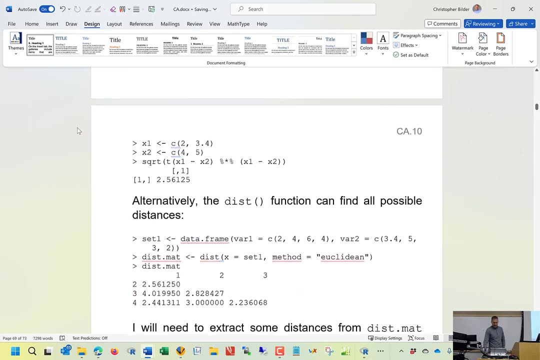 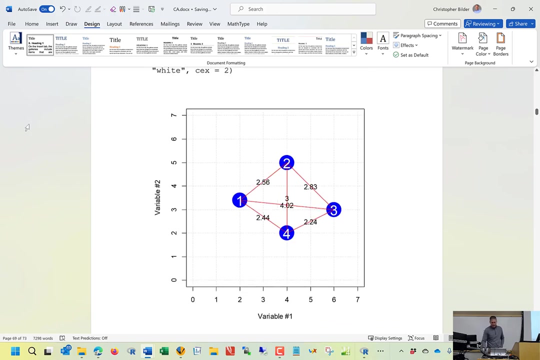 Euclidean distance by taking the 2 to the 3.4.. I'm going to put that into my x1 vector And I take the 4 and the 5, put that in my x2 vector, do the matrix multiplication and I get 2.56.. Here's a nice plot that helps illustrate this. So I 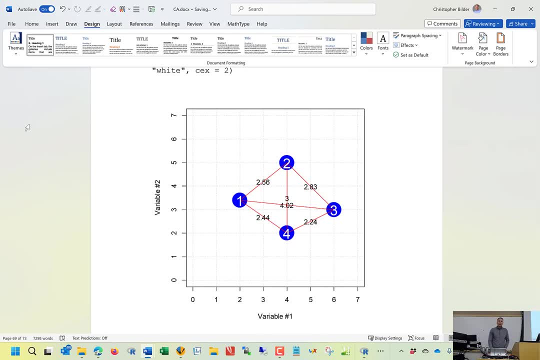 have the, you know, variable one and variable two. Variable one is on the x axis, variable two is on the y axis. I have the actual variable numbers, nicely labeled there as one, two, three and four, And so we had just found the distance. 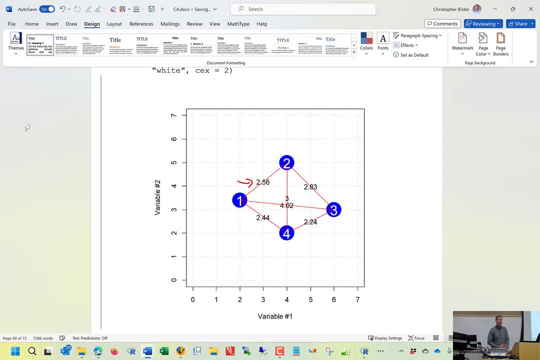 between observation one and two, which was 2.56.. So I drew a line there to say, hey, I'm going to find a distance and I put the actual distance type in here. So these are all my distances between the observations And the way then that we 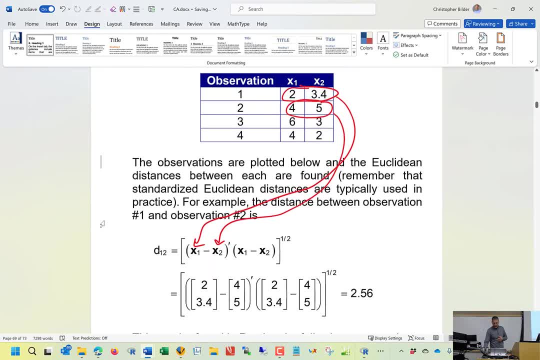 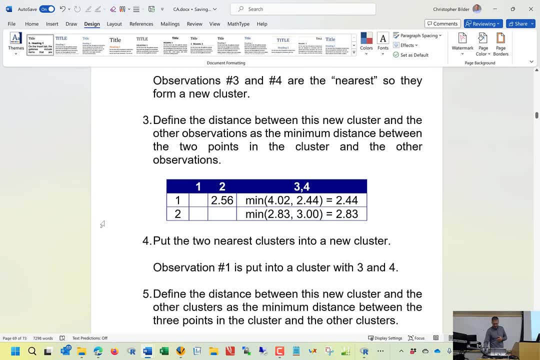 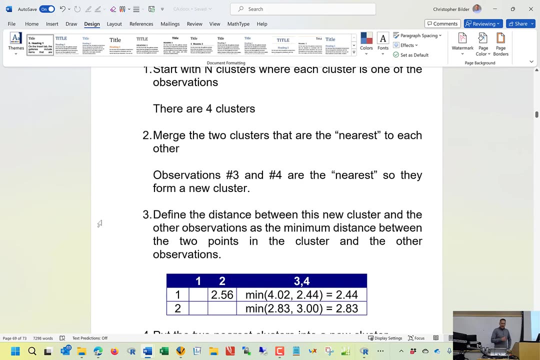 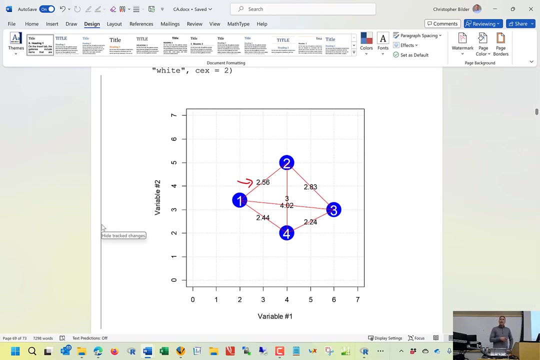 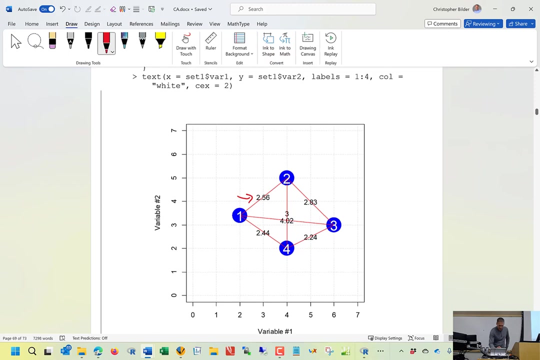 start the clustering process. Sorry, I am jumping ahead here. I need to find the observations that are closest to one, In other words, again, the clusters that are closest to one another. I'm going to join them together. So you look at all those distances that you see there. Well, what's the 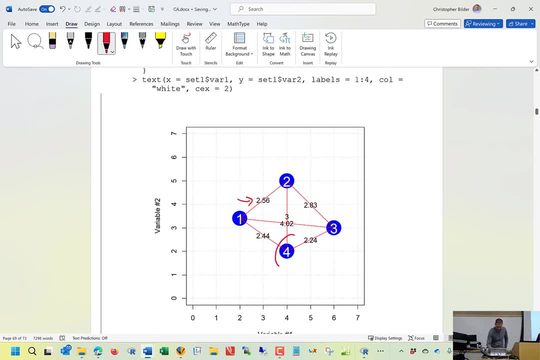 smallest distance. Well, it's the distance between three and four, Distance of 2.24.. So that's my new cluster. So now I have three clusters: A cluster with just observation one, a cluster with just observation two and now a cluster with 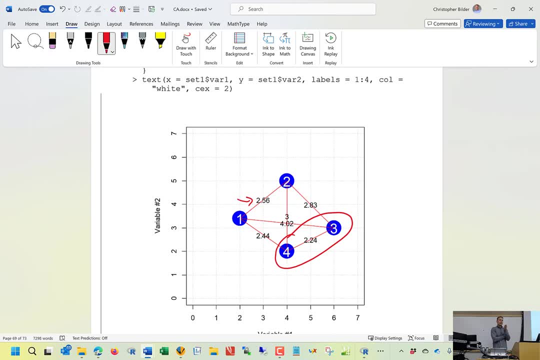 three and four. Now the clustering process continues. I need to decide, well, which clusters am I going to merge next? What the nearest neighbor method says is find all the distances between the clusters, And that's what I've done on page 12.. Right, 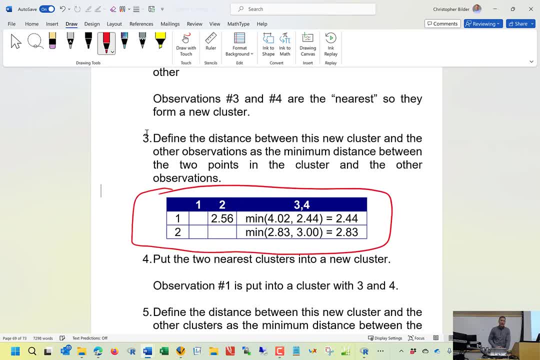 here. So the distance between the cluster that has just one in it and the cluster that has just two in it is, well, it's just the distance between 2.56.. But what's the distance now between the cluster that has just observation one in it and the cluster has three and four? What the 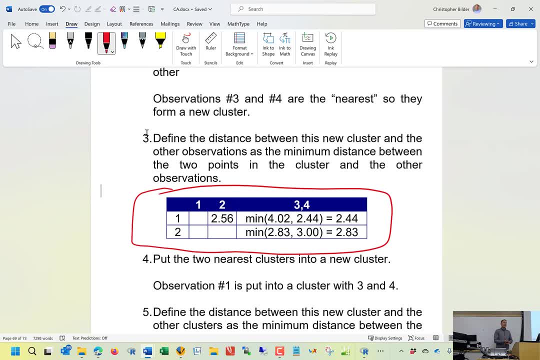 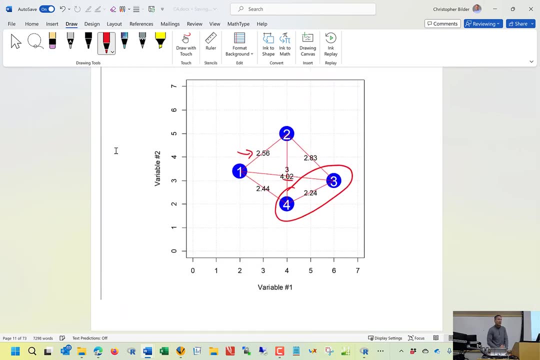 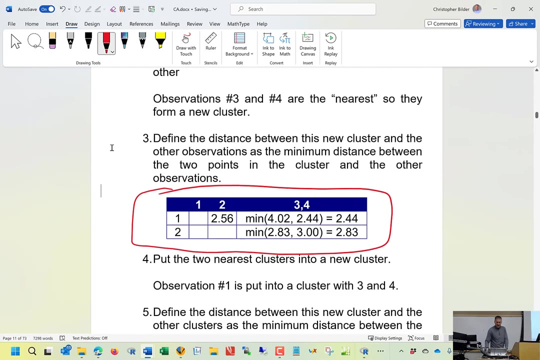 nearest neighbor method says is look at all the distances and find what that minimum distance is. So the distance between one and three come up here. the distance between one and three is 4.02.. The distance between one and four is 2.44. So the distance then that cluster one is to the. 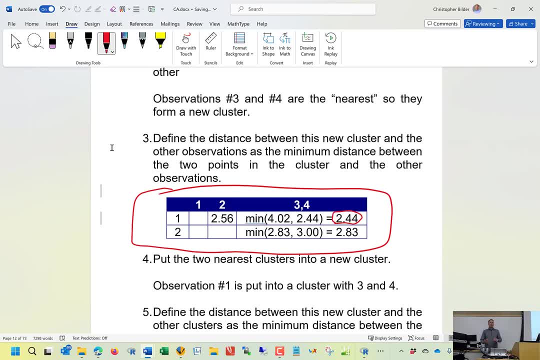 cluster that has three and four in it is 2.44.. Nearest neighbor: Observation: three is the nearest neighbor to one When I compare one to a cluster that has three and four in it. That's where the name comes from. Now, what about? 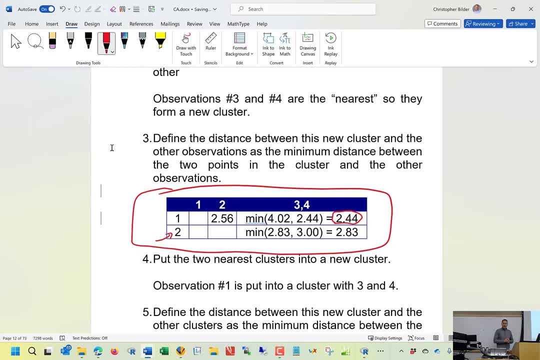 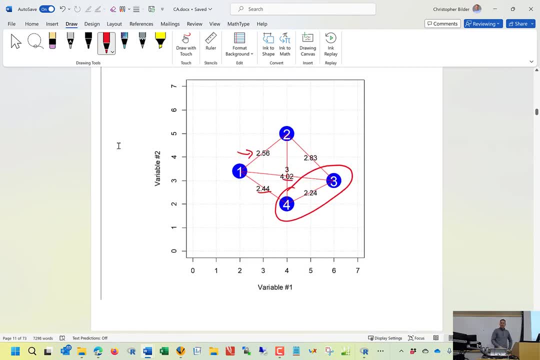 the cluster. that has just observation two it. Well, let's look back at the plot again. The distance between two and three has a distance. uh sorry, the distance between two and three is 2.43.. The distance between two and four is three, So the 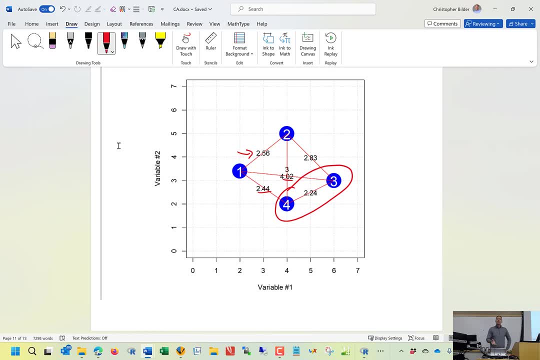 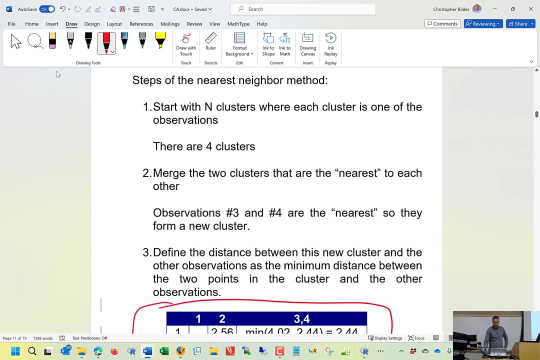 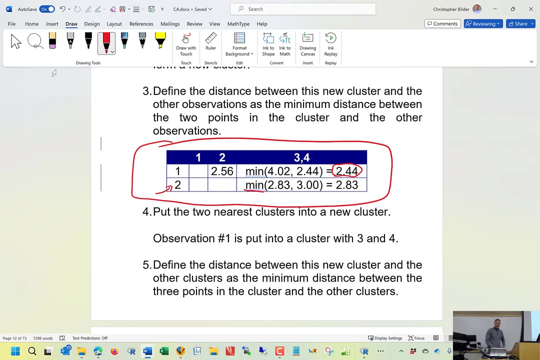 nearest neighbor to two is observation three, And so the distance between two and the cluster has three and four in it is 2.4.. is 2.83. so, based upon what I see here, then well, what is now going to be the next cluster form? it's still the minimum value in terms of the distances between. 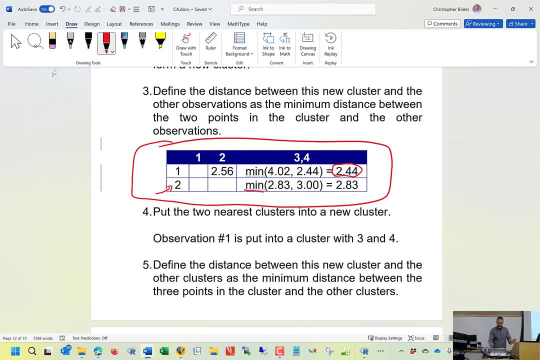 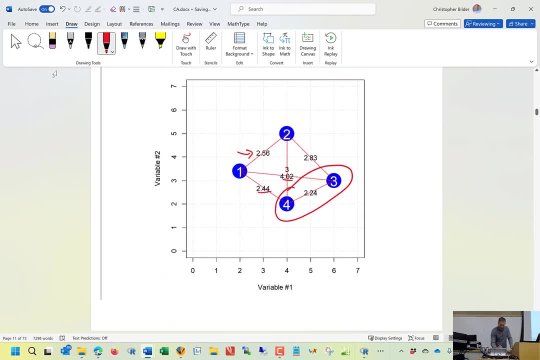 the clusters. and that smallest distance is right there: two point four, four. so now get a new one here. now for my second stage of my clustering process. I have a cluster that has just two in it, and then a cluster that has one, three, four. okay, now the next step is to get rid of the clusters and then the next step is to 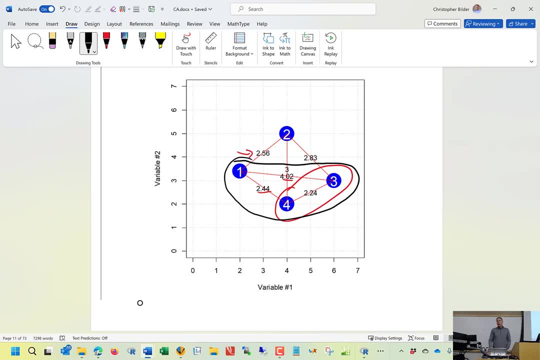 get rid of the clusters. and then the next step. I need to decide. well, what am I going to merge next? well, it's going to have to be two with one, three, four. but let's think about the distances. what would be then the distance between the cluster that has two and the cluster that has one, three and four in it? what? 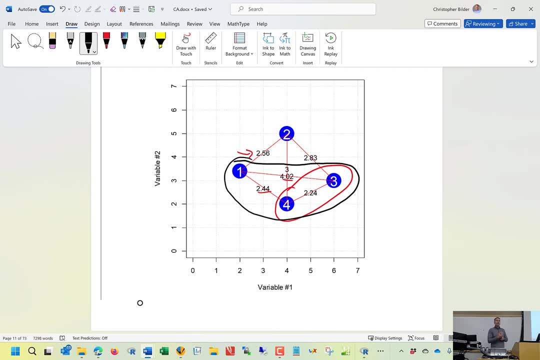 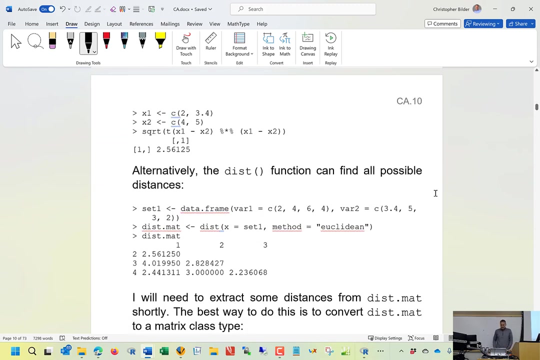 will be the distance two point five, six, because that's the minimum distance. one is the nearest neighbor to the cluster that has just two. okay, so that's how it works. let me come back up here. so sorry that I skipped around a little bit. so, top of page ten, I just show you in R how to do the actual. 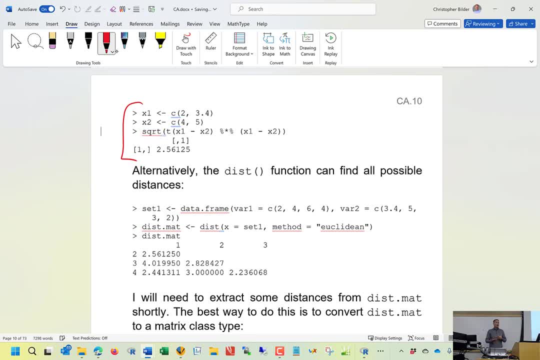 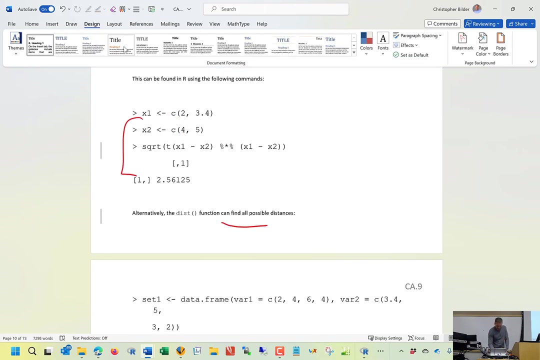 map if you were to find then the actual distance between observation one and observation two. Fortunately there's a nice function in R called dist that will find all distances between your observations. So how did I use it? Suppose I create oops, suppose I let me remove the grammar check here. that's kind. 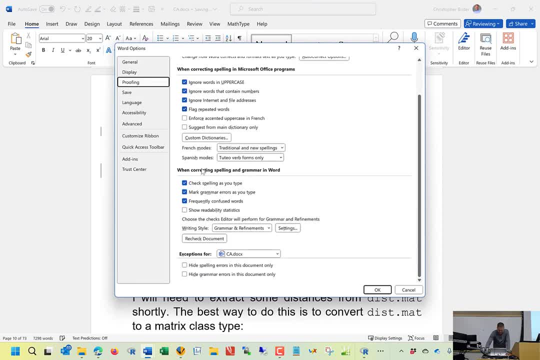 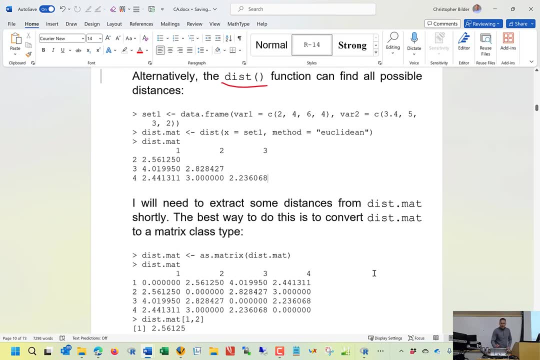 of annoying. okay, so I create a data frame called set one, where the first column is going to be for bar one. I just put in all the variable one values. second column is going to be bar two. put in all the variable two values. that's going to go into a data frame called set one. 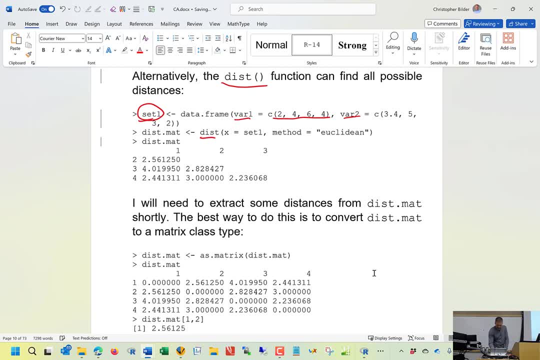 for the lack of a better name. And then I say dist First argument: x equals, set one. What kinds of distances do I want Here? I just want Euclidean distance. So I put that into an object called distmat for distance matrix. I actually have formally. 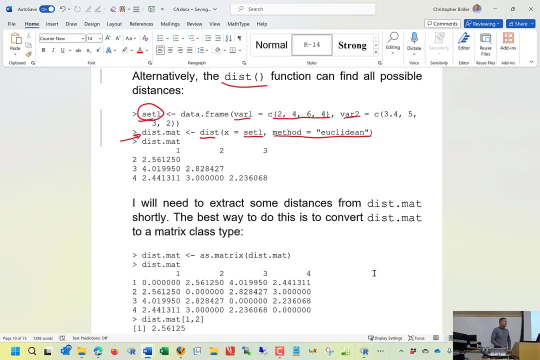 a matrix, but it just made sense to do that and this is what I get for all those distances. Some people refer to this as a lower triangular matrix, Even though it's not a lower triangular matrix, Even though R is actually not recognizing this as a matrix class. 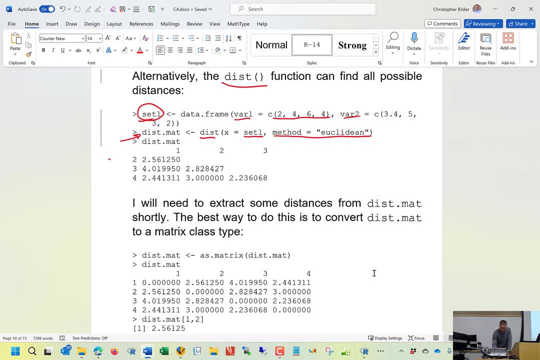 And so to make sure you understand how to read this, so the distance between observation two and one is 2.56.. Notice, we do not have a. well, let me skip that. The distance between three and two is 2.82.. 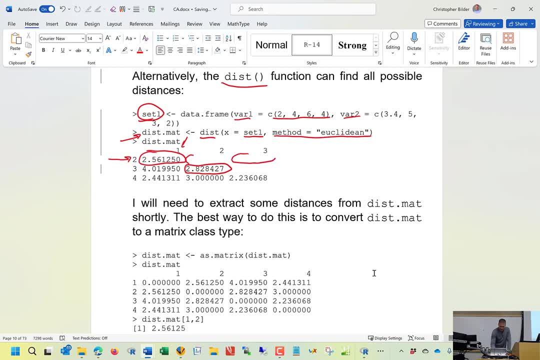 Now notice: I do not have a distance between two and three. Okay, Why? Well, because it would be exactly the same Whether I'm looking at observation two versus three or observation three versus two. it doesn't matter, It's still the same distance. 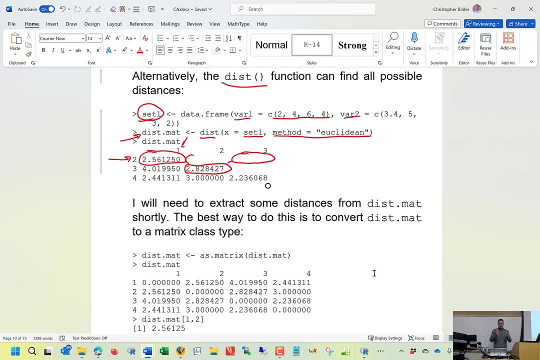 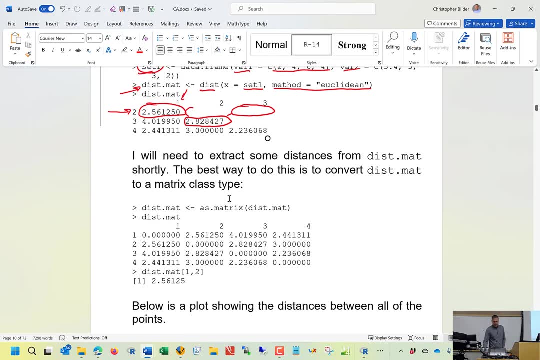 So that's why you see those empty spots in that structure. Now, to actually to do my plot coming up, I need to transform this into something that R actually recognizes as a matrix. And the way to do that there's a function called asmatrix, meaning treat it as a matrix. 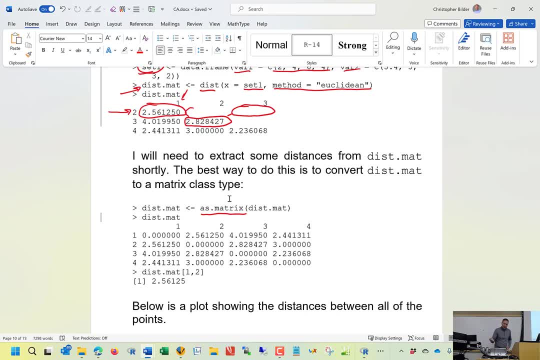 So if I do asmatrix of dismat and I just put it back into an object with exactly the same name, Now I do have an actual matrix, and the reason why that's important is because I can actually access a row Okay, And a column to pull out the different distances. 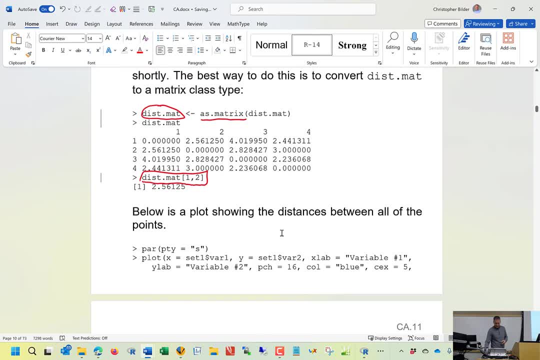 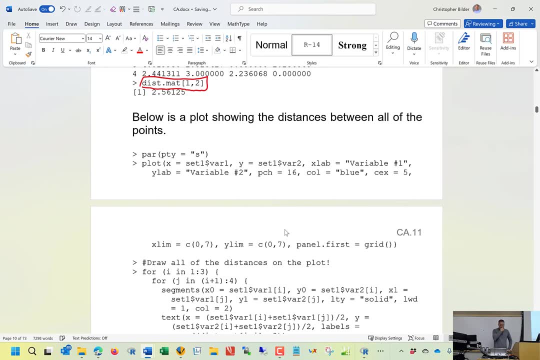 Okay, Now how did I do that plot? Depending upon your interest in knowing understanding this code, I will go into more or less detail. So what I do here is I first use the plot function, where on my x-axis I put variable one, y-axis, variable two. 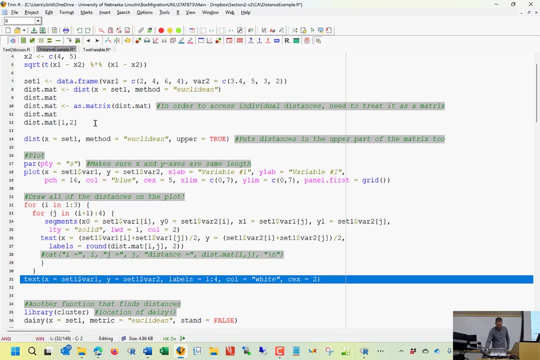 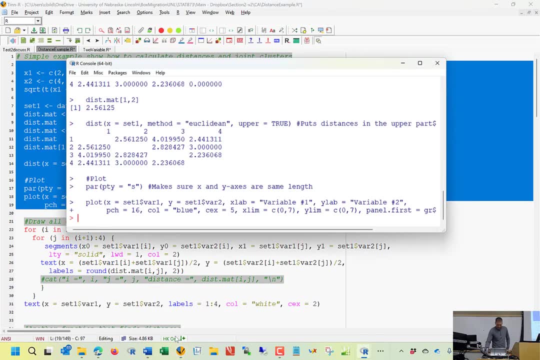 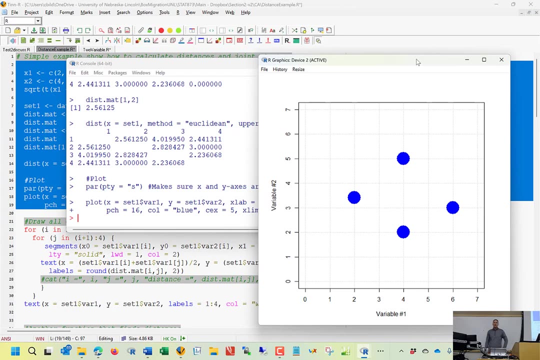 Let me actually just come over here. There it is. So I begin with by plotting the simple points. I have a big blue circle there. How do I get the blue circle? Well, I say: color equal blue. Plotting, character equals 16.. 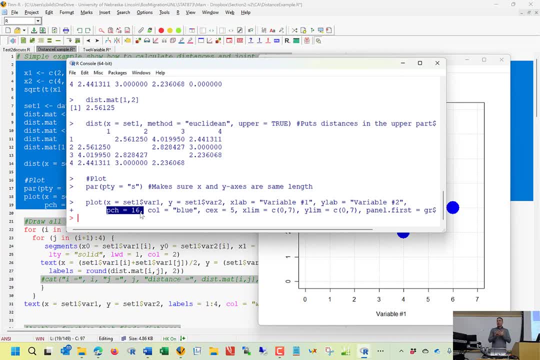 If you go back to the intro to R notes, you'll see that what's often called a filled circle or closed circle is plotting character number 16.. And then I use cex equal five, meaning make the plotting point five times larger than the default. 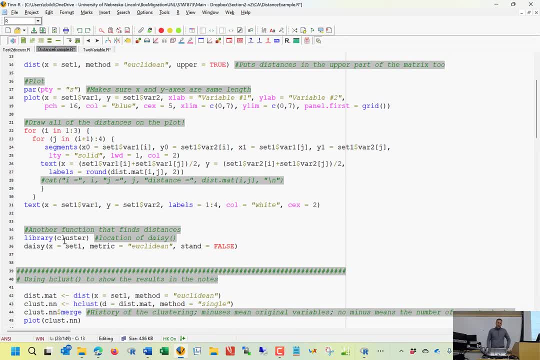 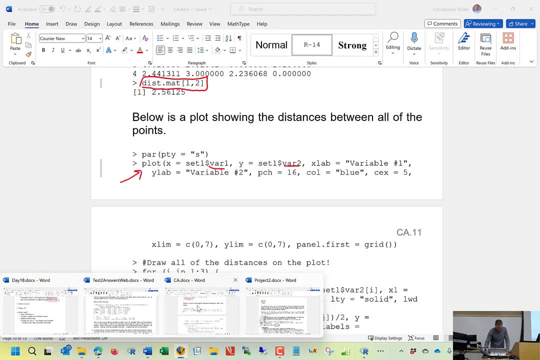 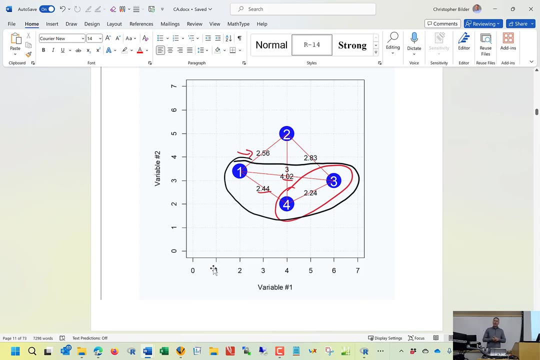 Okay, Now To get the actual lines And the distances actually shown on the plot- So the red lines- and to actually plot the distances there that you're seeing, I need to use some for loops. Now, in many programming languages there are like for looping structures. do looping structures. 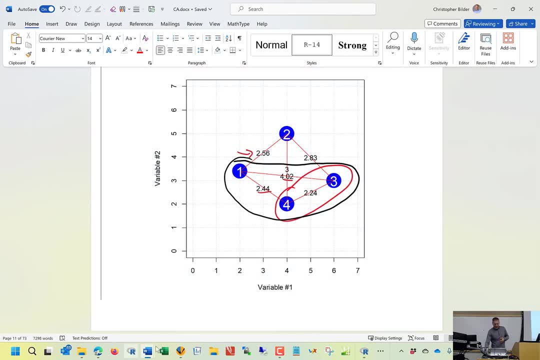 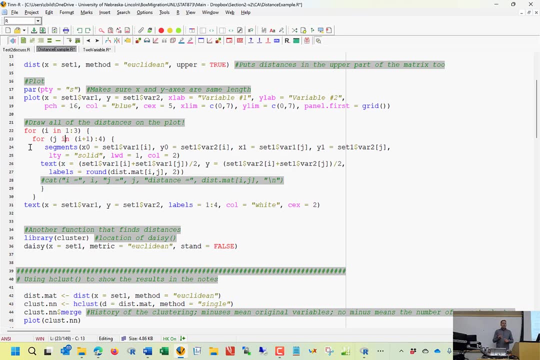 R uses a for looping structure here, And so what I do? Okay, So for each possible, let's say for each pairwise combination of the variables, Let's say variable one, I'm sorry- For each pairwise combination of the observations. 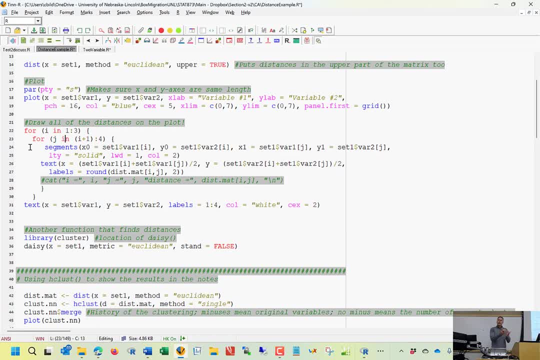 Let's say observation one and observation two, Observation one and observation three, Observation two and observation three. What I'm going to do is use the segments function To draw a line Between the two blue dots representing those observations And then right in the middle of that red line. 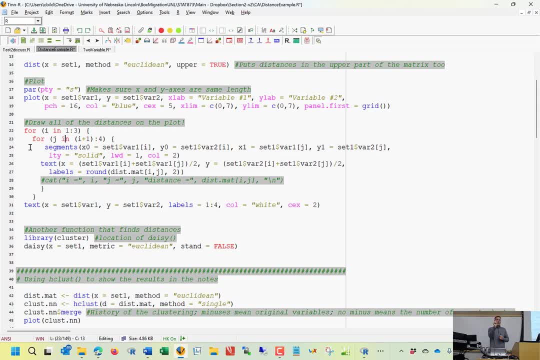 Meaning kind of like a halfway point. I'm going to plot the actual distance, I'm going to actually plot the numerical value of the distance, And I do that through two for loops, And so this is what I'm going to ask you here. 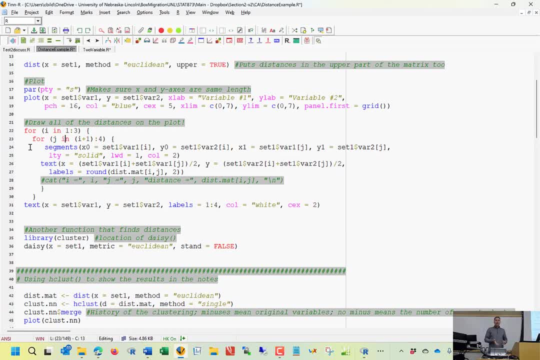 Would you like me to go through this for looping structure here, Or Are you comfortable enough with for loops that I can skip it? It's up to you. I'm happy to go over it some more. Okay, Okay, Let's. 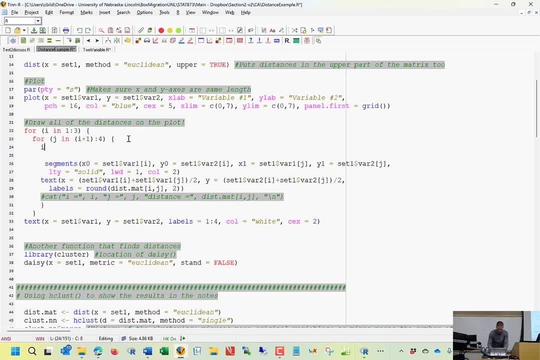 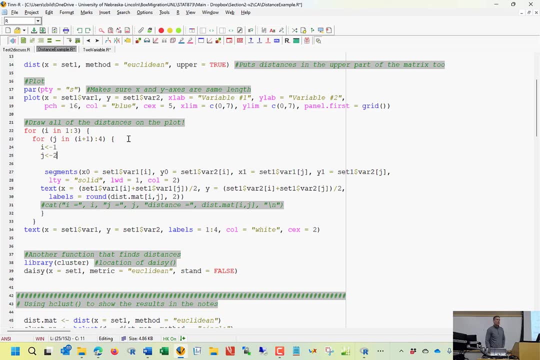 So I have two indices here, I and J. Is this big enough or do you need me to make it bigger? Big enough? Okay, Two indices, I and J, And what this is going to correspond to first is that I is going to be for observation one. 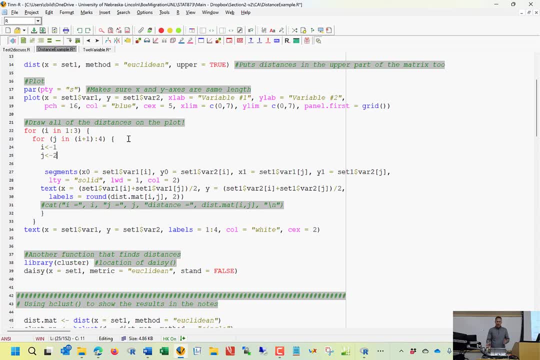 J is going to be observation two And so if I just highlight this code, Okay. So for example, Here's I, I is equal to one, And then I'm going to use the segments function To draw a red line Between observation one and observation two. 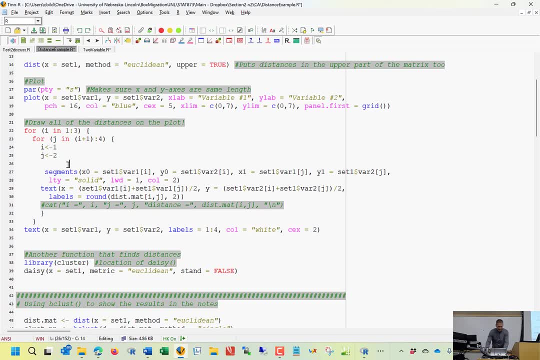 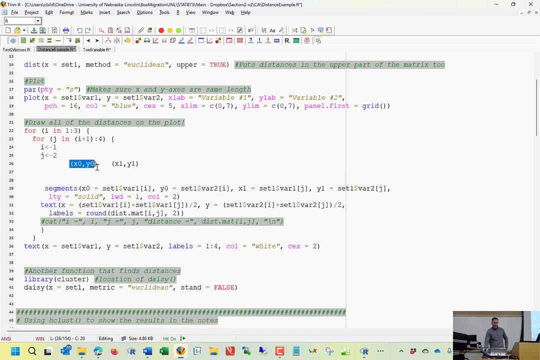 The way that the segments function works. is that? Imagine you have. Oops. I have two points on my plot. One is going to be at, Let's say, X sub zero, Y sub zero In terms of the X axis, The Y axis. 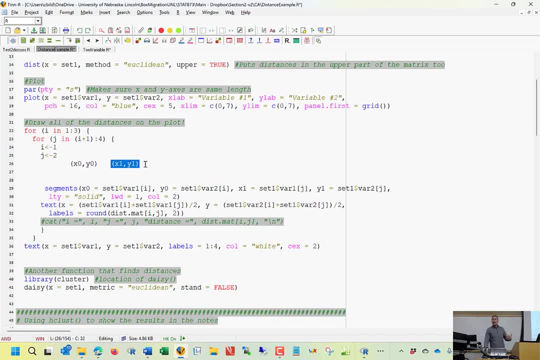 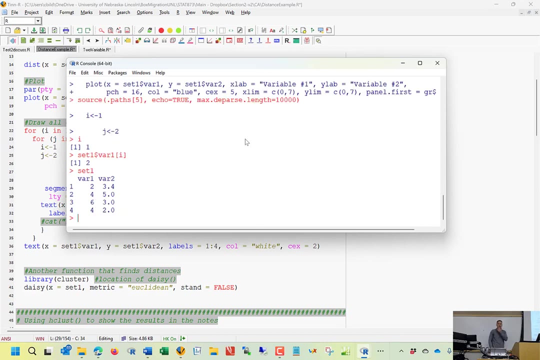 Another point is going to be at X one and Y one, And so in the segments function I specify X, zero, And so what that's going to be is the first variable value for observation one. Okay, That's, It's equal to two. 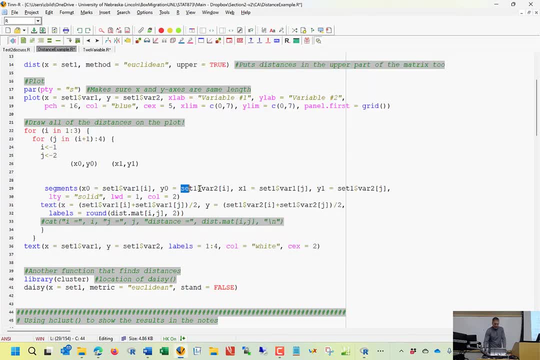 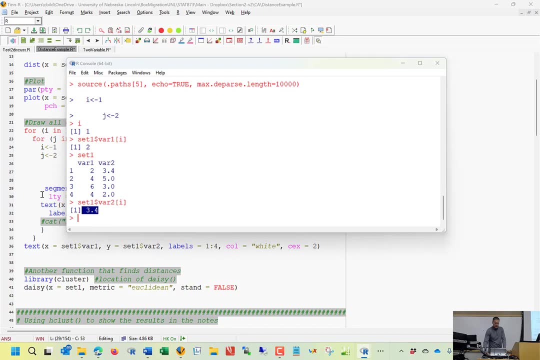 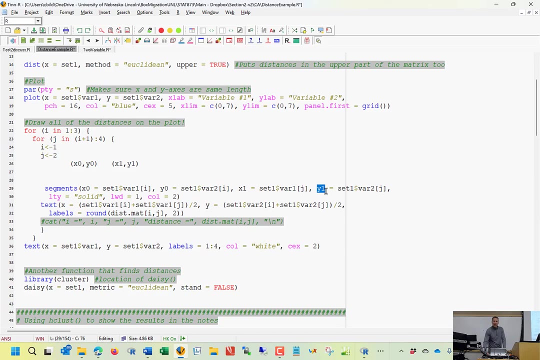 The Y zero component is going to be for the second variable value for observation one. Three point four, X one, Y one is now going to be for that second variable. I'm sorry, The second observation- Excuse me The line type- is going to be a solid line. 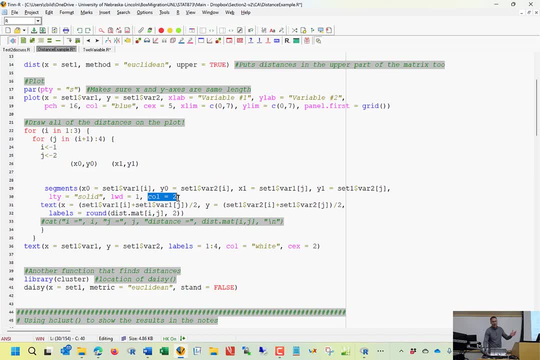 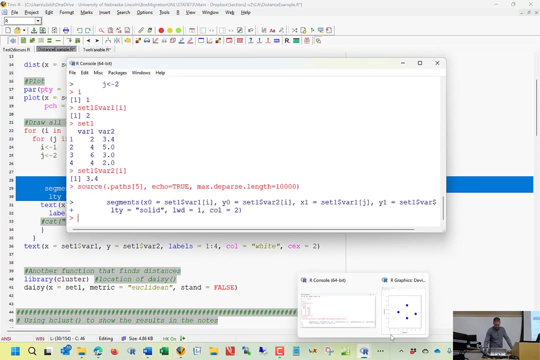 It's going to have a color of two, Which R translates into red, And the line width is just one Meaning. It's just a default. I didn't actually need to put that. If I run this segment of code, What you're going to see on the plot- 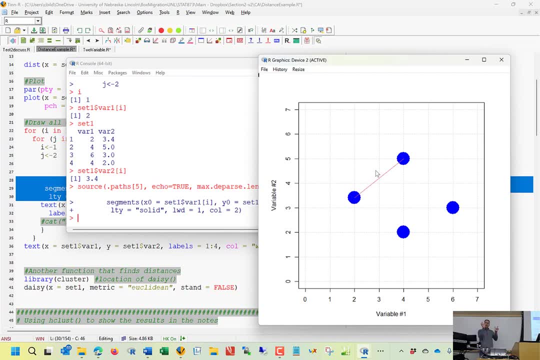 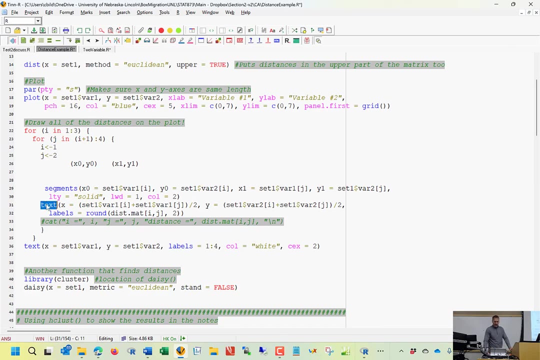 Is the red line. So I took the two points In our two dimensional space, Drew a line between them. Now I'd like to actually put in Here what the actual numerical value of the distance is, And so I can do that using a function that we've seen before called text. 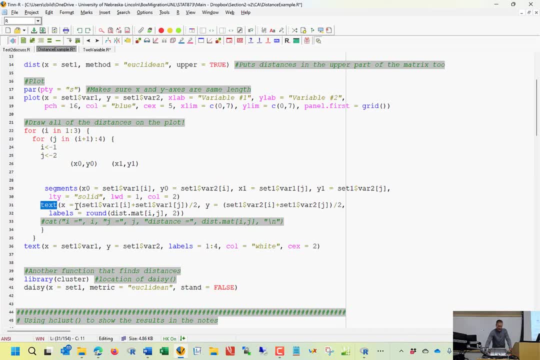 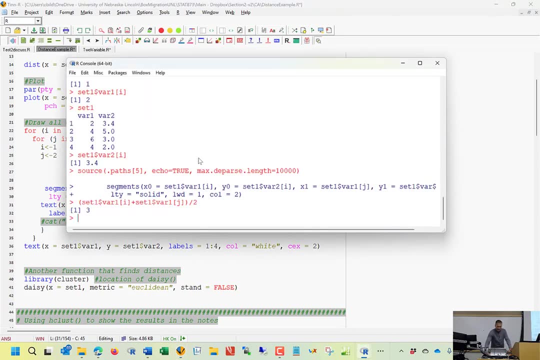 Where do I want to plot the actual numerical value? Well, What I'm going to do is find the average Between Variable ones: The value for variable one for observation one. The value for variable one for observation two That values three. 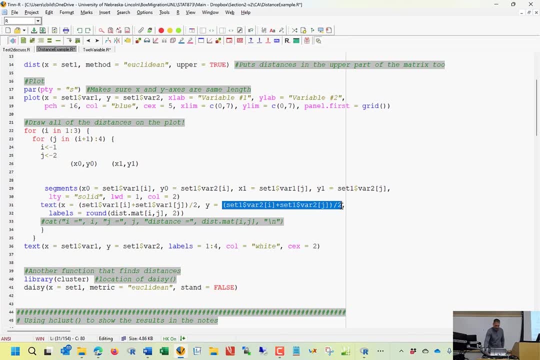 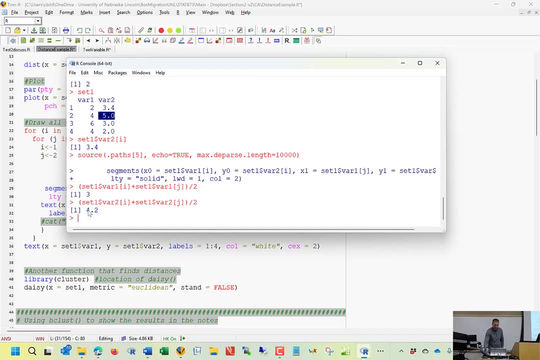 That's going to be on my X axis. My Y axis is going to be the average Between three point four And five. So Four point two. Why am I doing this? Well, If you look at the plot, That should mean then. 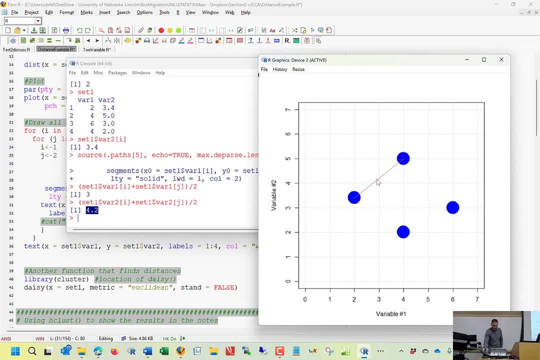 I should be like: If you see where my mouse is, I should be right about here Where I draw my text. What's the actual text? I want the actual numerical value, And so that's where I go into my Dis. 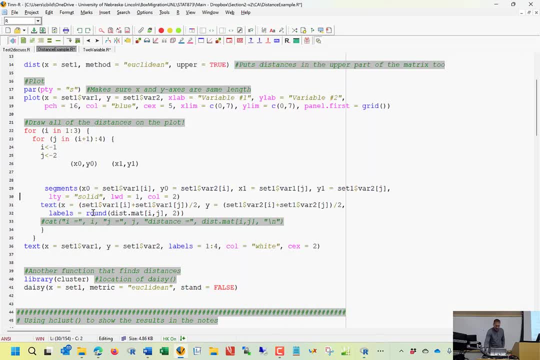 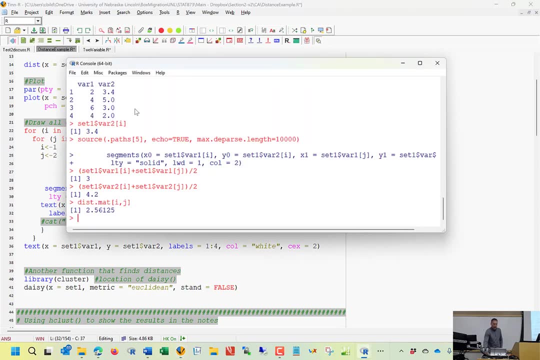 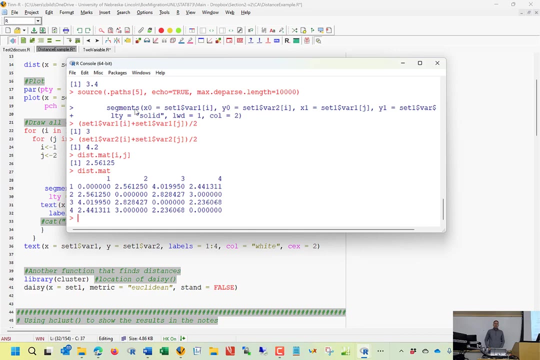 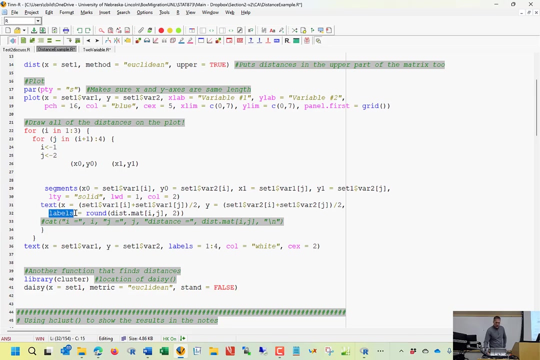 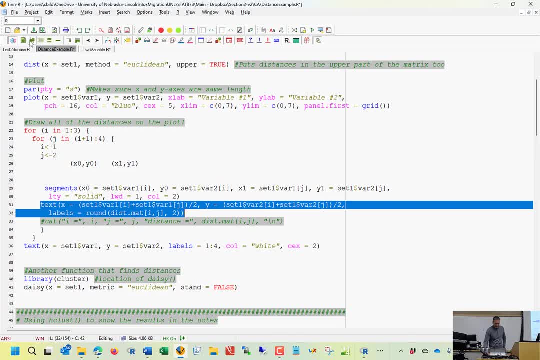 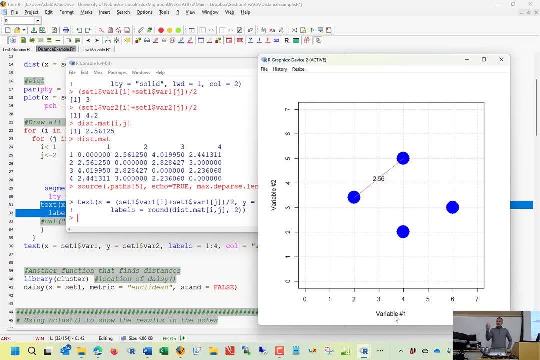 For the text function, And I rounded Two decimal places So that It just looks nice, And so, When I draw that out, There we go. Now I would like to be able to Repeat this process For now. 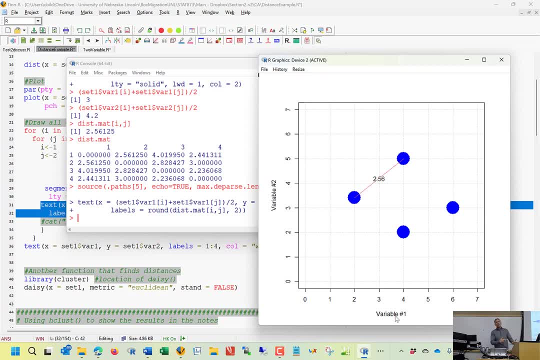 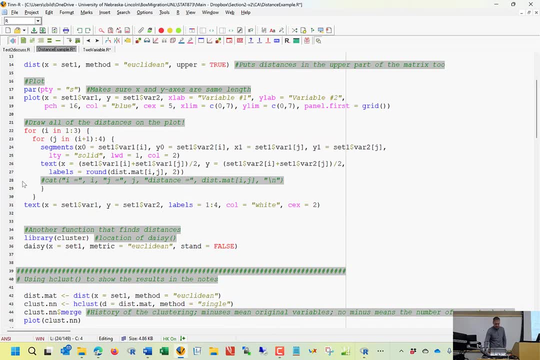 Observation one And three, Observation one And four, Observation two And three And so on. in where I say for I in 1 to 3, I use a curly bracket. you can see what's highlighted there in red. everything inside those two curly brackets is. 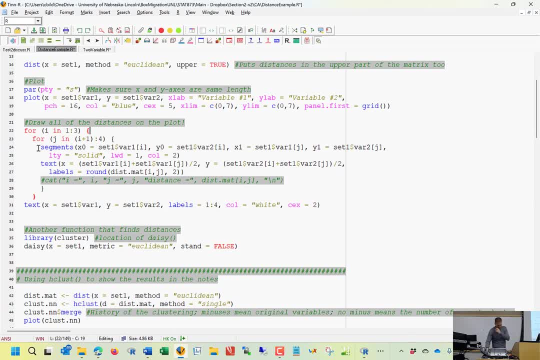 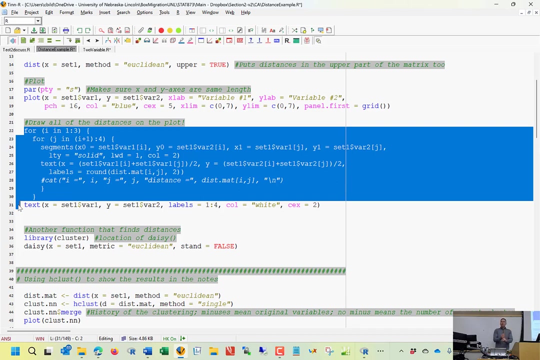 within that for loop. then I say for J in I plus 1 to 4. everything inside the curly bracket is within that for loop. so I have nested four loops, and so the first time that I run this segment of code I is going to be 1, what's J? 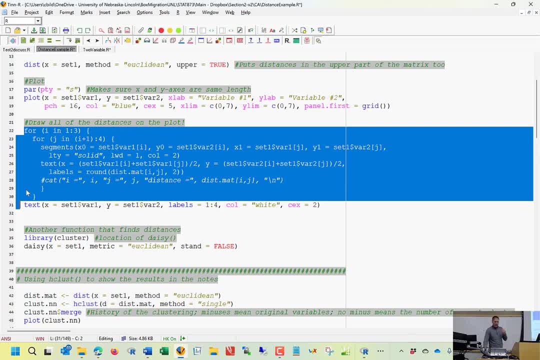 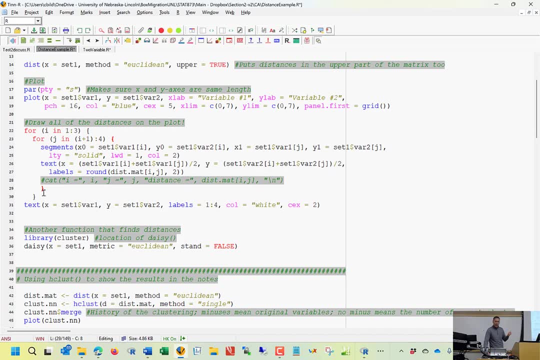 2, 3. okay, and so I is 1, J is equal to 2 and I'm going to get exactly what I had just drawn before. then you get to the bottom of the for loop. then it's going to come back up here and say: okay, well, now I need to go. J equal to 3, so it's going to 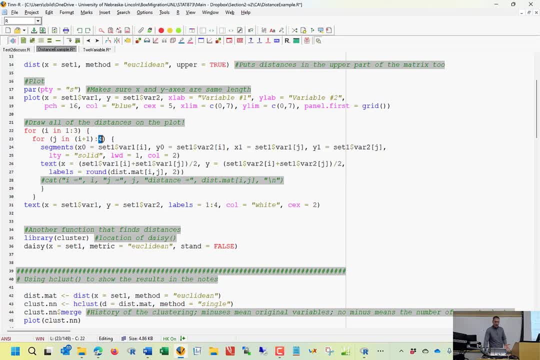 do for I equal 1, J equal 3. then it's going to come up here and sees: okay, I still have J equal 4 to deal with. so now I have I equal 1, J equal 4. and then it gets down to here and says, okay, I guess I'm done with that for loop, now I'm going to go. 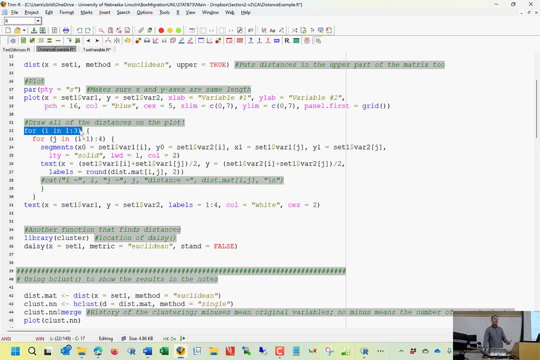 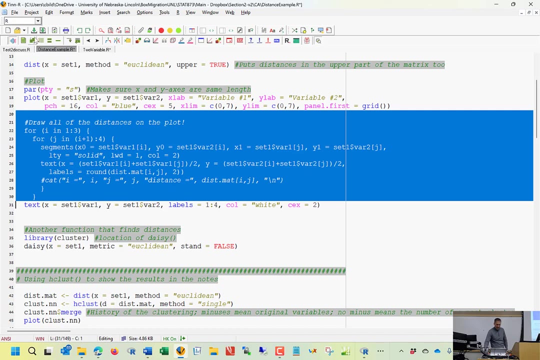 back up to my original for loop, and now I is going to be incremented to 2. so now I'm going to do this from: for I equal 2, J will be 3, and I keep on doing this process over and over again until I went through the entire for loop, and now I 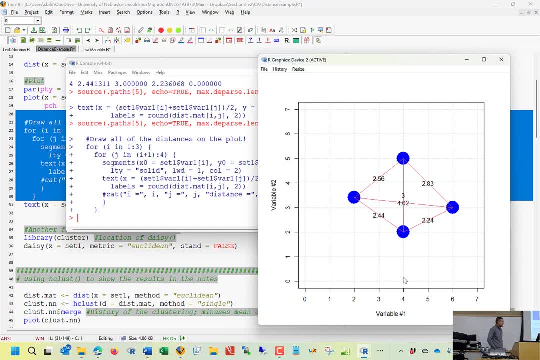 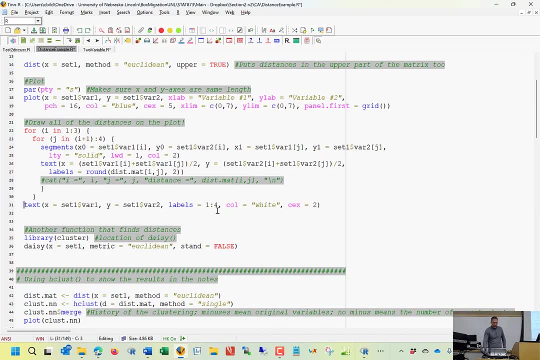 get all my red lines. I have all my distances. last thing I need to do is I need to plot the actual observation numbers, and I use the text function to allow me to do that. the labels argument is just simply: well, the numbers 1, 2, 3 and 4, color is white. C, X equal 2, meaning we're going to 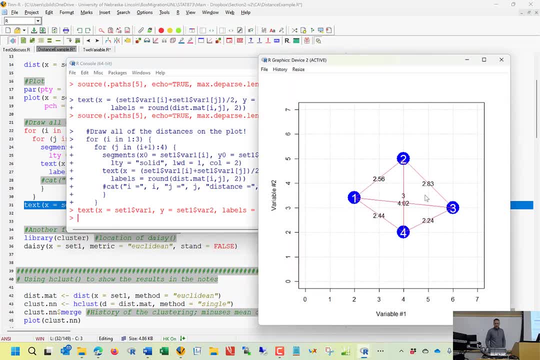 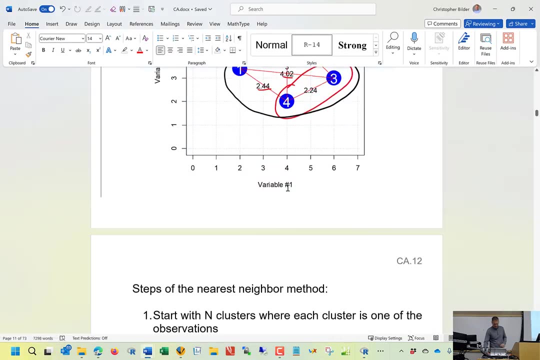 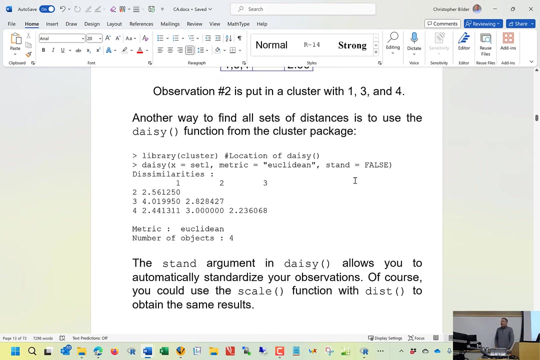 make it twice. this the default in terms of size, and there's my clock. any questions? okay, now there is another way that you can find these distances: the the function that I just showed you. the dysfunctions within size step package. there's also a package called cluster, and sometimes people will use this. there's a function. 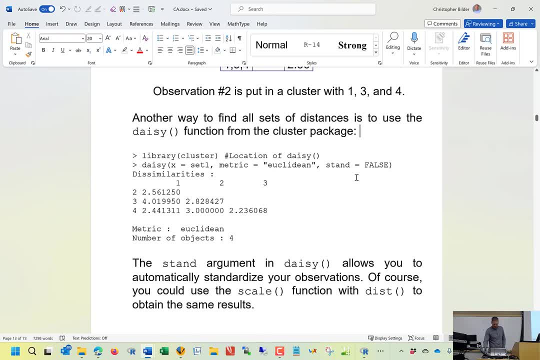 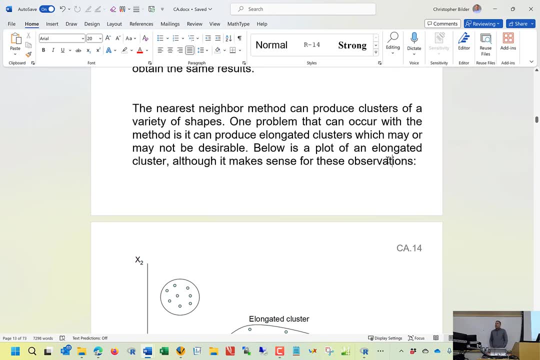 called cluster, and then sometimes people will use this. there's a function called Daisy that will find those distances as well. Okay, Now, as I told you, there's many different augmentative methods out there. Nearest neighbor, also called single linkage, is just one of them, And again, there's multiple ways to do this. 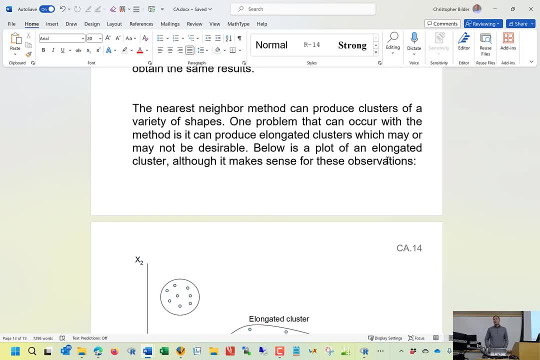 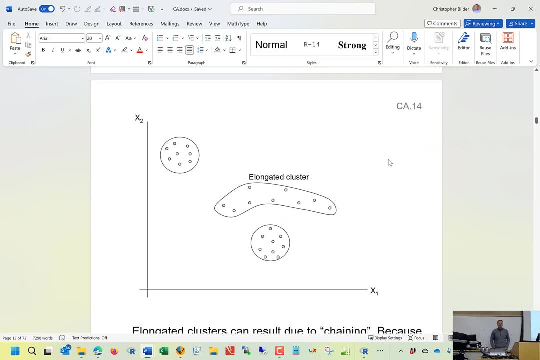 because none are perfect Or none is the best, I should say. The problem that nearest neighbor can have is it can have what are called. it can form in the end what are called elongated clusters. So maybe during the clustering process you get to a point where you have these three clusters and for some reason you 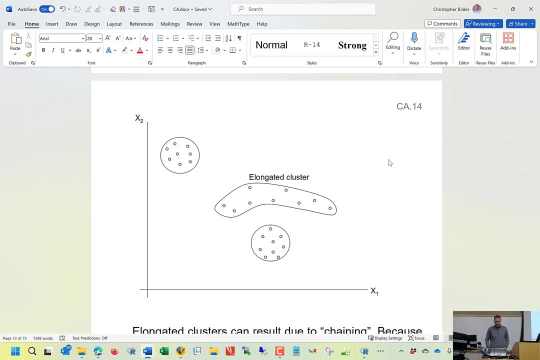 decided to stop, And we'll talk about how to make that decision later- And so what we have there is labeled one elongated cluster. Now, in this particular case, that, that elongated cluster seems fine. You know, again we're trying to find similar. 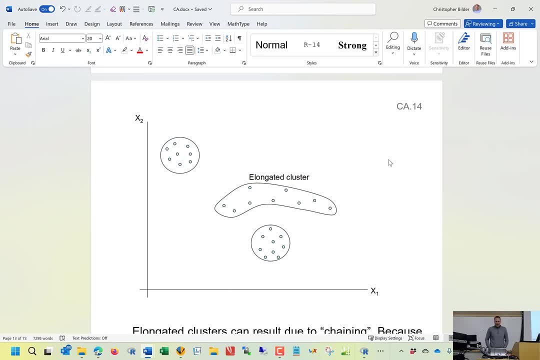 observations, put them into groups, clusters, and indeed it looks like we have three distinct groups there. I just wanted to show you what an elongated cluster looks like. Now, in another situation, you know, maybe you might have something like this. 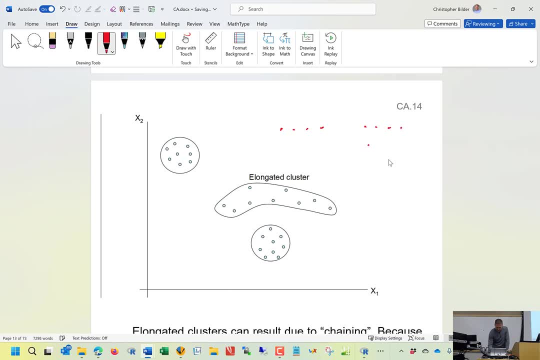 Let's say we have these observations. What can happen is is this- And this isn't necessarily drawn to scale the best, But we have two clusters here. They're elongated as you can see. They're kind of stretched out When that's what nearest. 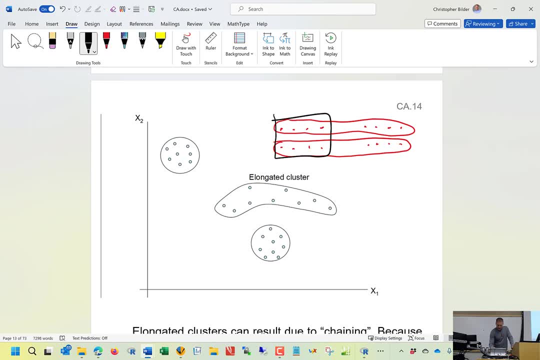 neighbor might conclude. But you know, if we look at this another way, maybe we should have this instead. Well, why does this happen? Why does nearest neighbor perhaps result in those red clusters there? Well, it's because of how nearest neighbor works, You know, through this hierarchical process. observations: 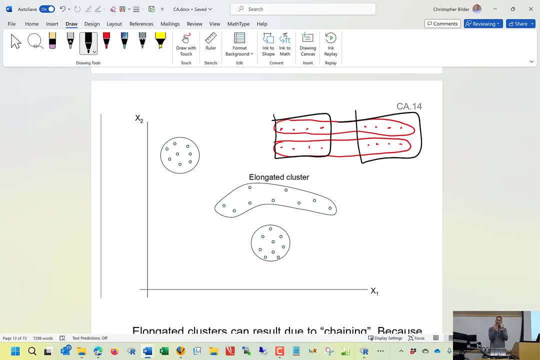 are joined to particular clusters And the distances between the clusters is always the shortest distance between, let's say, this cluster and this cluster, And that's what it's almost like: a like, you know, like a chain link, If you think of. 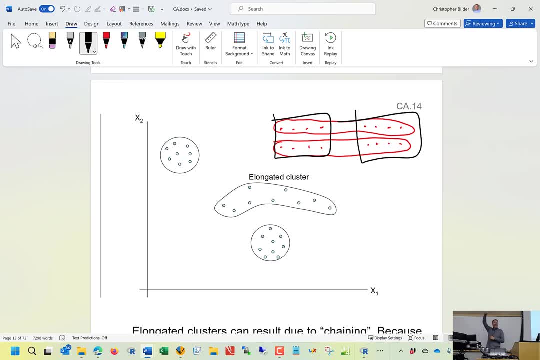 like a chain holding up a chain. if you can imagine a chain here, you know where you have different links together. You know it only takes, let's say, one close observation to link different, in this case clusters, And so because of that, you 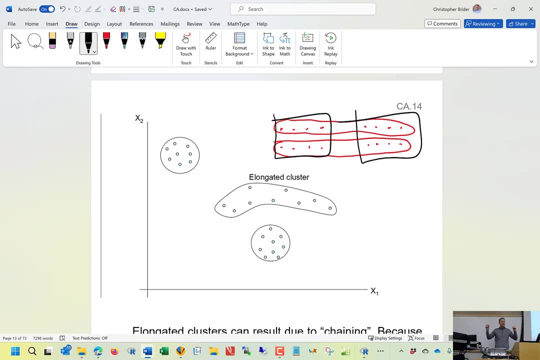 can end up having these elongated clusters like this. You know it doesn't look at the whole necessarily. it's not like one overall measure of distance between, let's say, a cluster that has five observations here and five observations here. Rather instead. 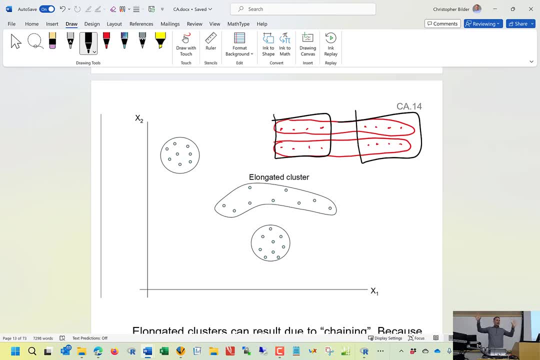 you're looking at the closest one here. you're looking at the closest one here to make that judgment about how you deciding what's the distance between the cluster and how you decide what to join, And so, because of that, you can have these. 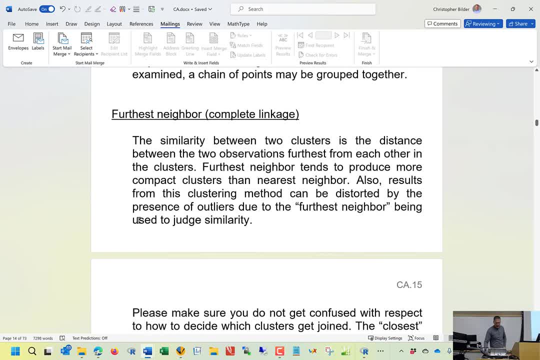 elongated clusters. So you might be thinking, okay, well, rather than looking at the nearest neighbor, how about we look at the furthest neighbor? You know the observations in two clusters that are farthest apart. we're going to define that as the distance between two. 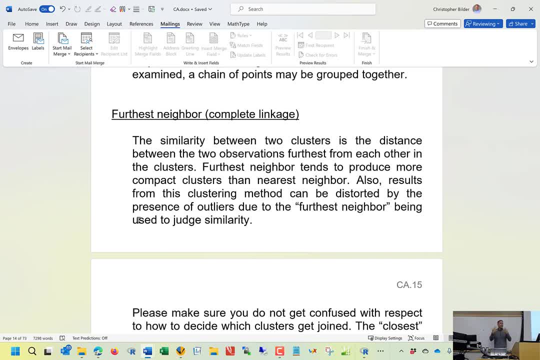 clusters And you could do that. That's called the furthest neighbor method, also known as complete linkage. So before we had single linkage, that name comes about that you know. it just takes two close observations to make that decision complete. 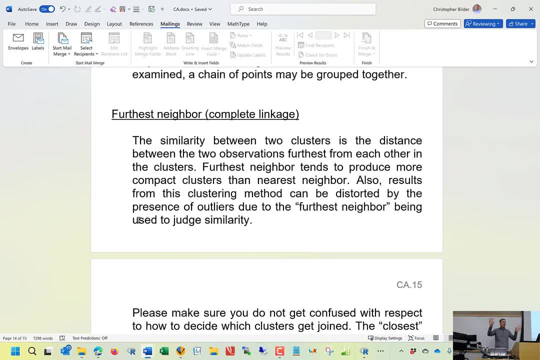 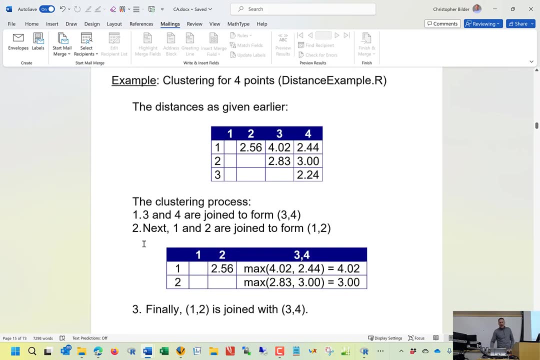 Basically now you have to look at all your observations in each cluster and then pick the two observations that are farthest apart to make that. So you're looking at all the observations, you're looking at the complete cluster to make this judgment. So let's talk about how this works. So we're going to, you know, look at this example again. 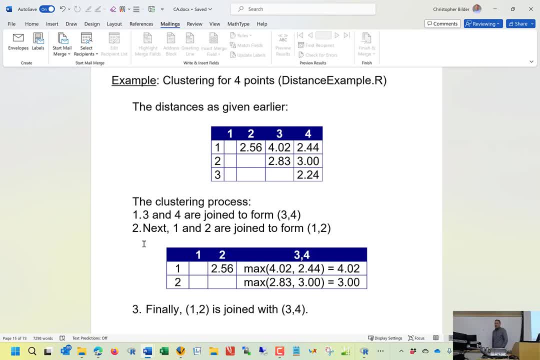 where we have these four observations. Here are the four distances. Now, this is we're aware. things can get confusing for students at times when they first see this. The measure of similarity here is equating distance, And I'm always deciding between which clusters. 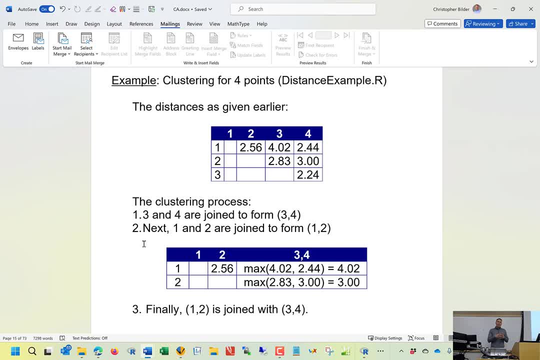 to put together by looking at the smallest distance between the clusters. So in this particular case, if I start off with four clusters, observations three and four are joined together. Now where this name of furthest neighbor comes into play is next when I decide which clusters. 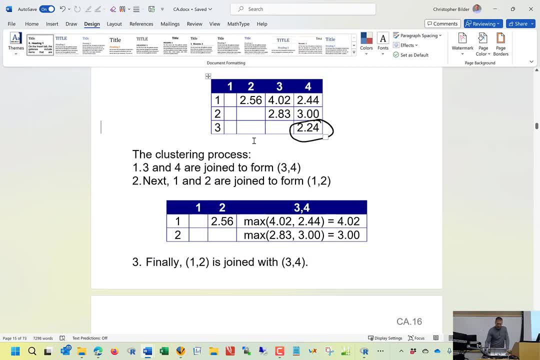 to join. So the distance between one and two is still 2.56.. But now what's the distance between one and this cluster? 2.56.. This is a cluster that has three and four in it. This is where furthest neighbor comes. 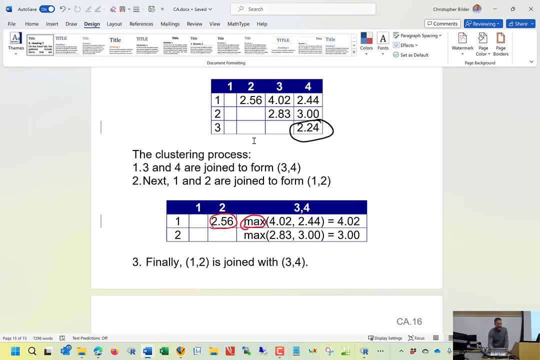 into play. Before with nearest neighbor I had min there. Now I'm going to use max. So the distance between observation- I'm sorry the cluster that has just one in it and the cluster that has three and four in it- is the maximum distance between one and three one. 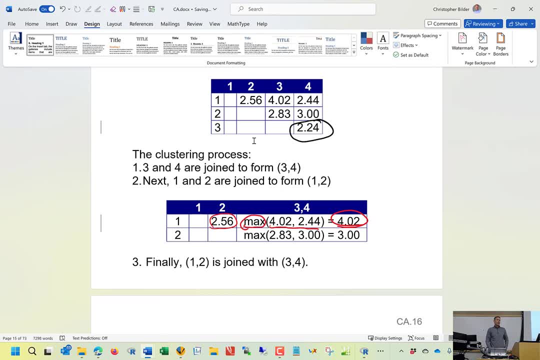 and four, That maximum distance is 4.02.. When I compare two to three and four, that maximum distance is three. So now I have this table of all these distances. How do I make the decision about which clusters to join? Well, again, we're looking for the most similar, The smallest distance. now that we see here. 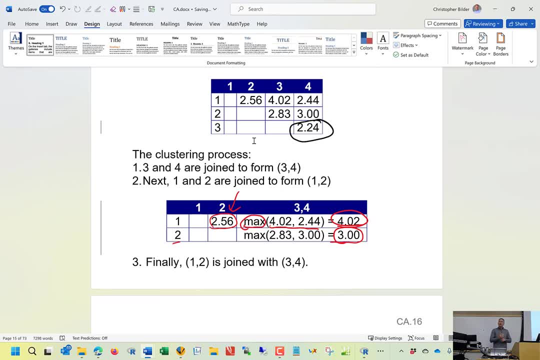 is 2.56. So observations one and two now have just one in a cluster Where students get confused then at this step is they say, oh, I'm using furthest neighbor. So that means observation one and the cluster that has three and four in it should be joined. 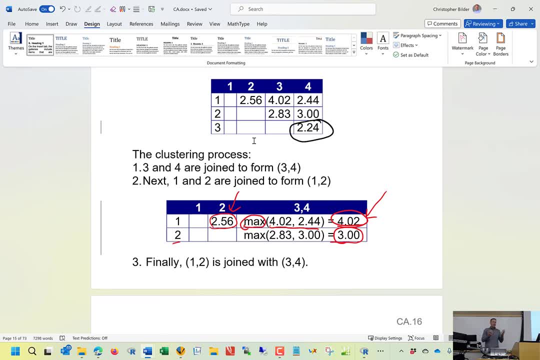 No, Where this name single. I'm sorry. where this name nearest neighbor and furthest neighbor come into play is when you make a decision. how do I measure the distance between the clusters? You always still join the clusters that are the closest together. It's just how. 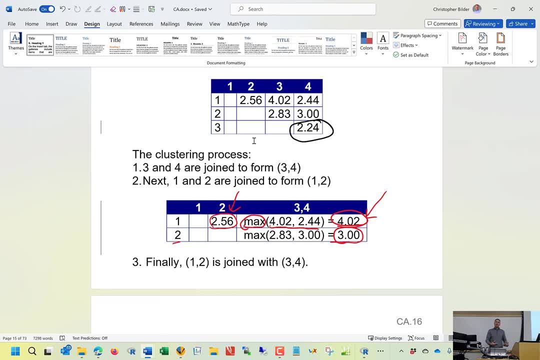 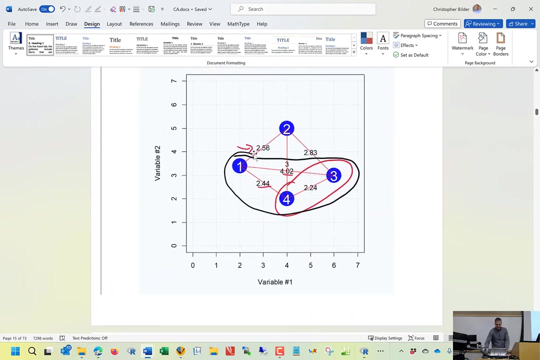 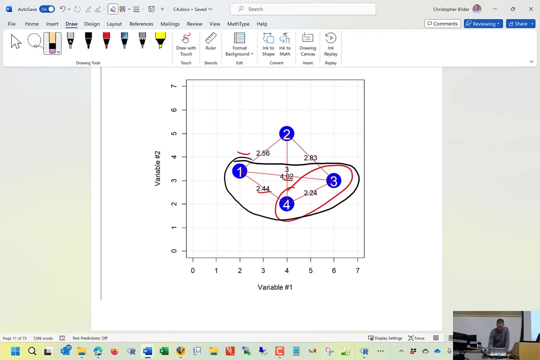 do you define distance? Any questions about that? This is a critical thing for students to understand. Any questions about that? So I'm happy to re-explain. Can you repeat that part again? Yeah, Sure, OK, Let's actually go back to our plot here. Let's see here, Because these are simple concepts. 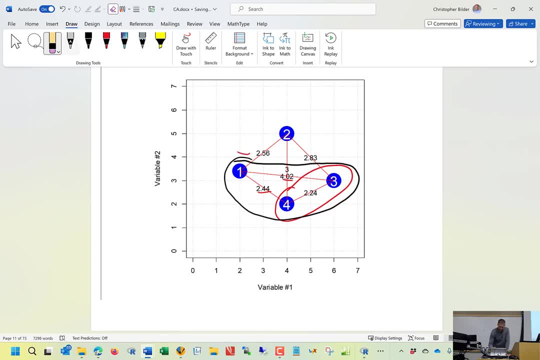 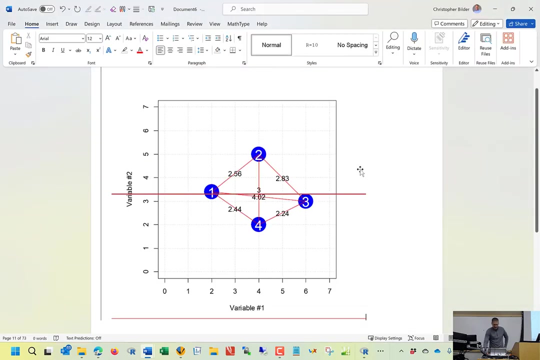 you know, nearest furthest, But it can be, just come on, my eraser's not working here. I'll just do it a different way And we'll try this. There we go. We'll try this one more time. 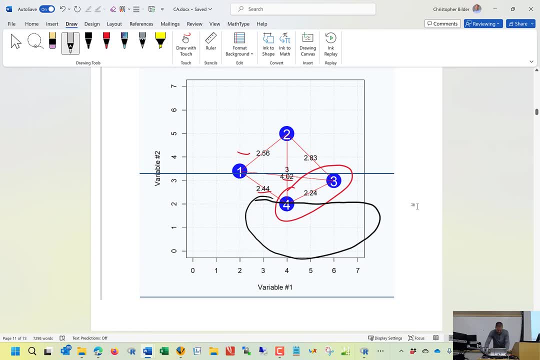 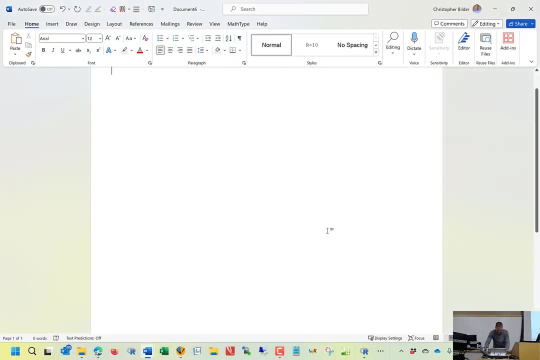 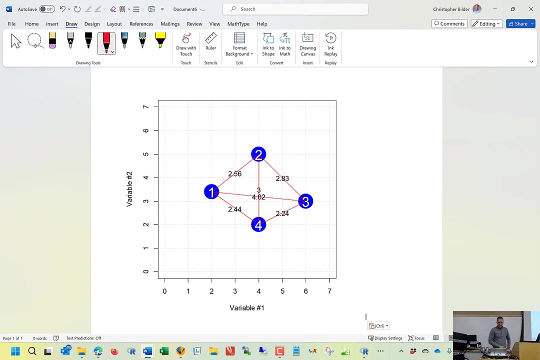 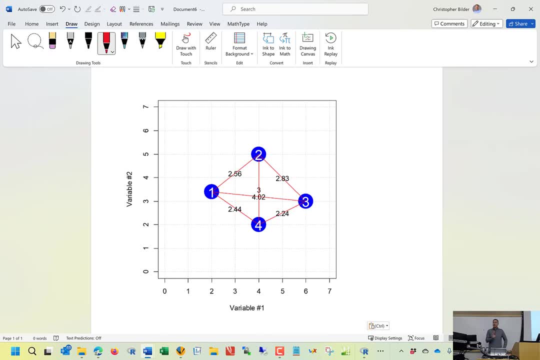 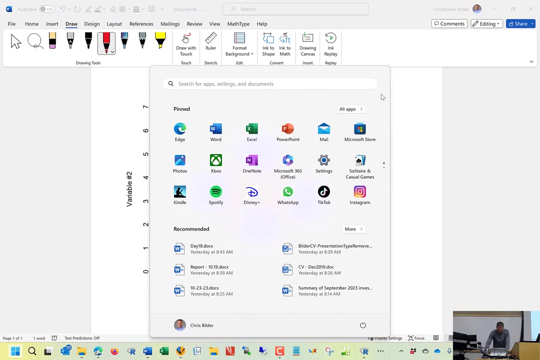 I have the distances between all of the clusters actually in or this diagram. This is the smallest distance, So I'm going to join them together, OK, OK, Oh man, Let's try something else. Let's go to my whiteboard. 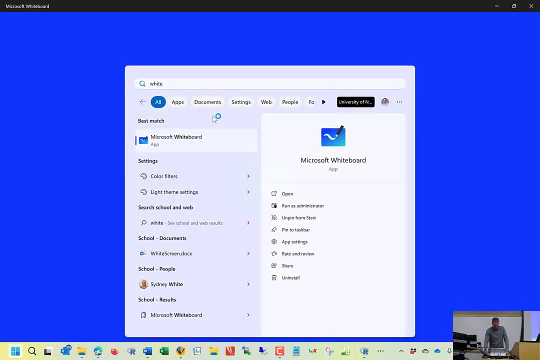 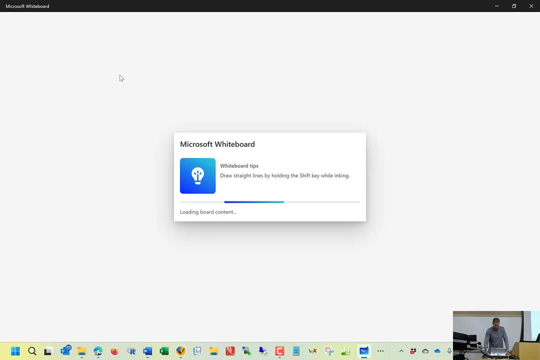 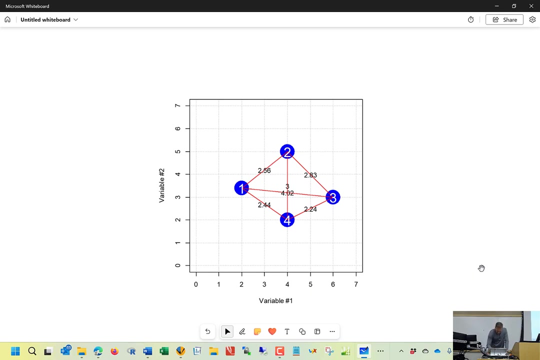 All right. So here we are. Here are my clusters at this stage, Because the cluster with just 1 in it and the cluster that has just 2 in it have just one observation piece. the distance between 1 and 2 is 2.56.. 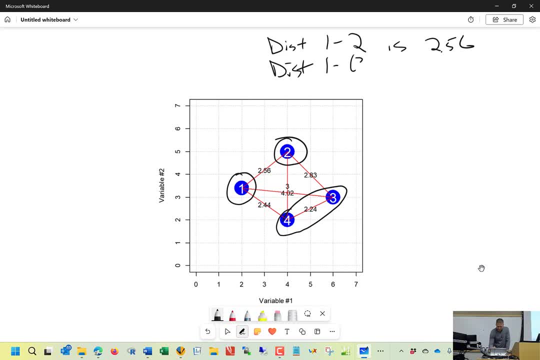 But also I need to define what's the distance between 1 and the cluster that has, let's say, 3 and 4 in it. This is where the name for this neighbor comes into play. I look at the distance between 1 and 3.. 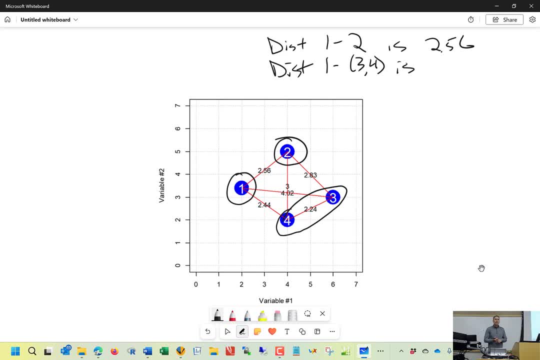 I look at the distance between 1 and 4.. The distance between 1 and 3 is the largest, So I'm going to define the distance between the cluster that has just observation 1 in it and the cluster that has observations 3 and 4 in it. 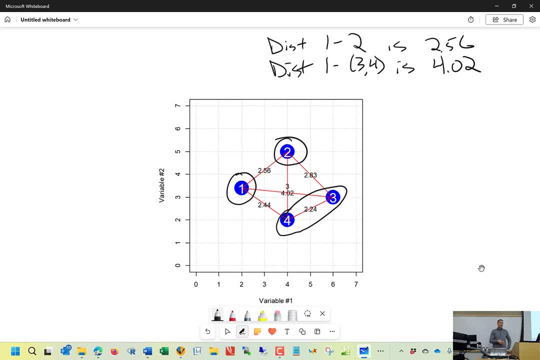 3 and 4 in it has 4.02.. Where the nearest neighbor, I would define that distance to be 2.44.. Now the distance of, let's say, 2 to the cluster that has 3 and 4 in it is 3.. 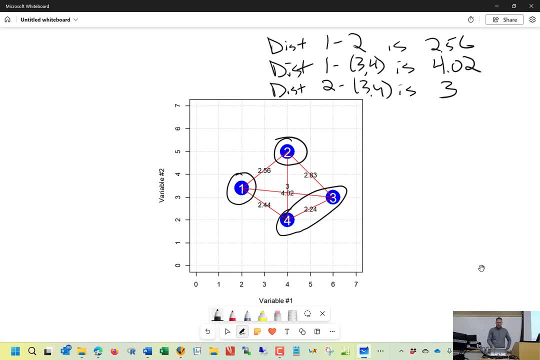 So the distance between 2 and 3 is 2.83.. The distance between 2 and 4 is 3.. So that distance is 3. Because I'm using the furthest neighbor method, So I have 3 distances here. 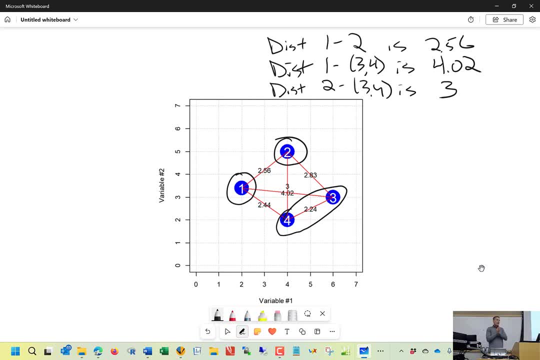 And I need to decide well, what's going to now be joined together To make that decision. I still look at, well, what's the smallest of those distances? That smallest one is 2.56.. So now I don't use whiteboard that often. 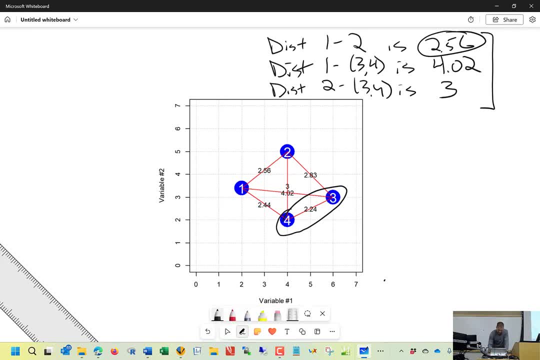 So sorry, Take a little bit longer than what I would like. So now I have those two clusters. So next I'm going to define the distance between 2 and 4 in it. So now, of course, the next what would happen is the cluster with 1 and 2 in it is going to be joined with 3 and 4.. 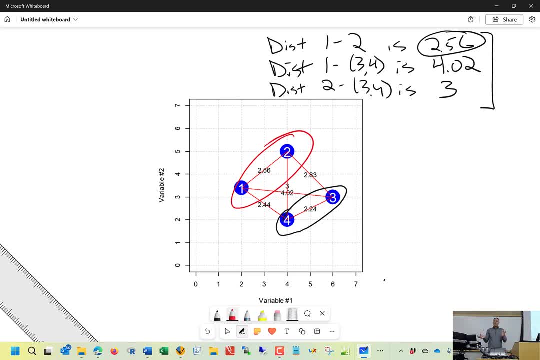 But my question to you is: what is the distance between the cluster that has 1 and 2 in it and the cluster that has 3 and 4 in it? Is that 3?? What I'm looking at, an actual numerical value for what is the distance between 4.02.. 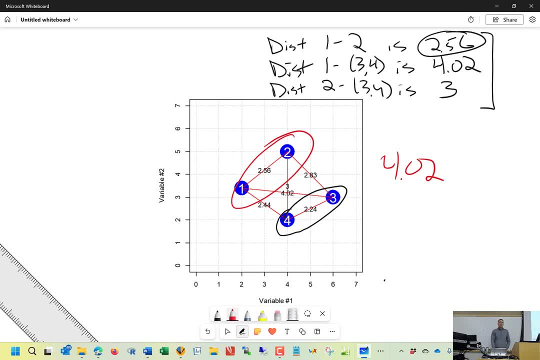 That's the distance. Okay, Because again we're looking at what's the furthest neighbor of this cluster that has 1 and 2 in it to the cluster that has 3 and 4.. What's the furthest apart? they are. 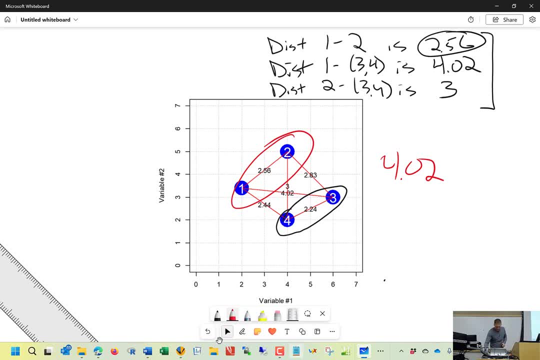 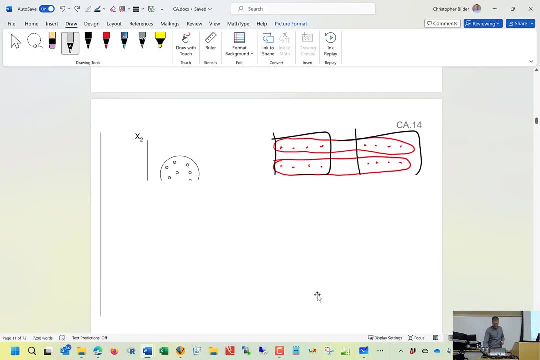 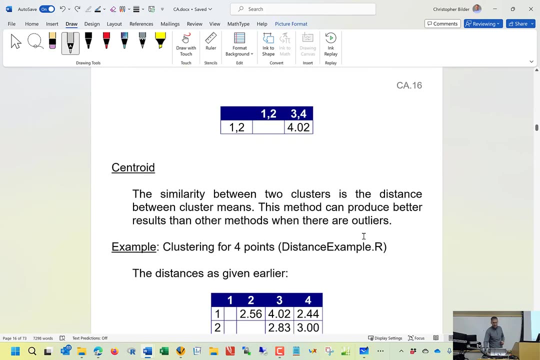 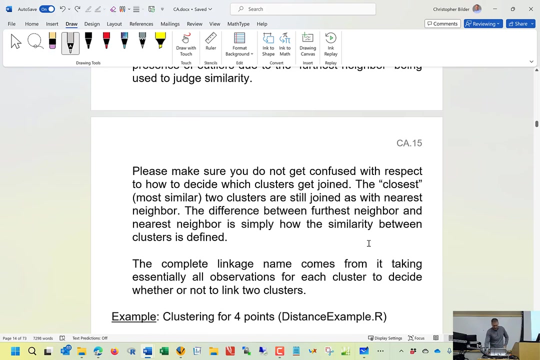 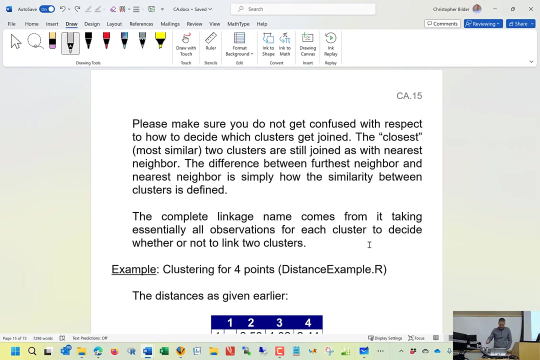 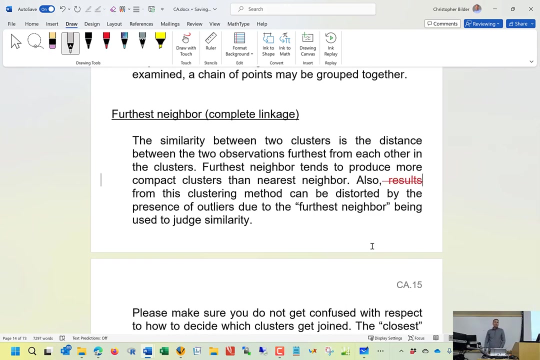 So that's how you make that judgment. Let's see here: Yeah, As you might expect, this method is not perfect. It can be distorted by outliers. So you can imagine: let's say one cluster, Let's actually do a plot here. 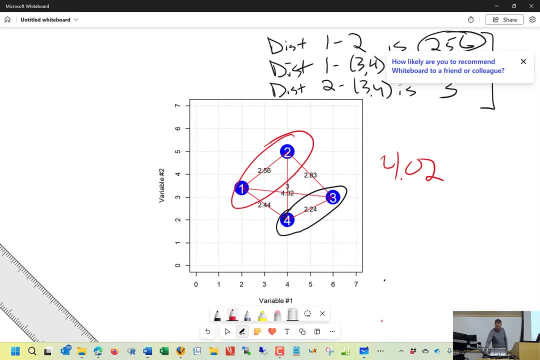 I think the computer is just having some difficulties here. So suppose we have two kind of compact clusters, But then we also have one outlier in one of those clusters And we can see how that's going to distort the distances between these two clusters. 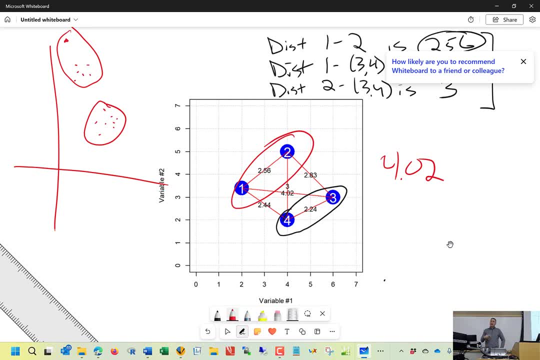 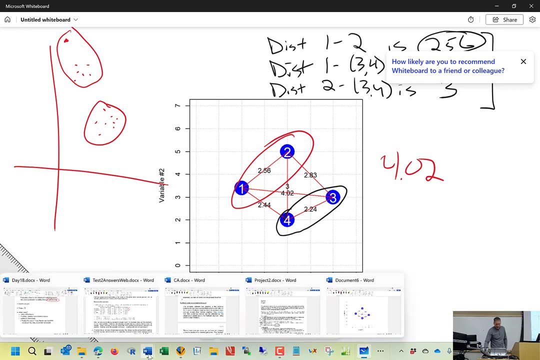 Because they have this one thing that's far apart, And so that can cause them problems about trying to find observations that are similar to one another and put them into nice clusters. So that's why this isn't a perfect method. So you might be thinking: okay, well, we've talked about the furthest neighbor. 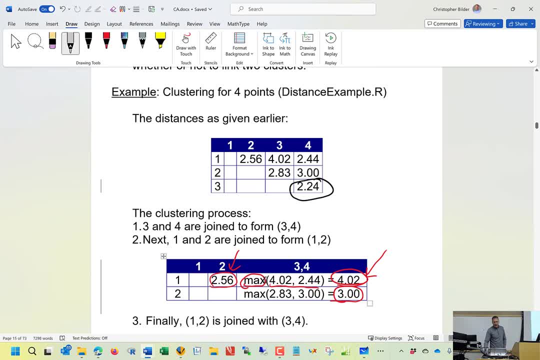 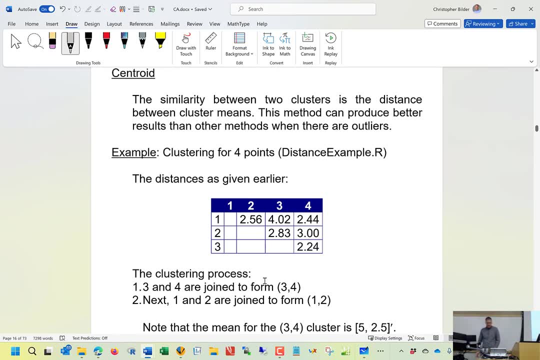 We've talked about the nearest neighbor. Is there something that we could do in between? Yeah, There's something called a centroid method, Where, if I want to find the distance between two clusters, I simply find the mean value for a particular cluster. 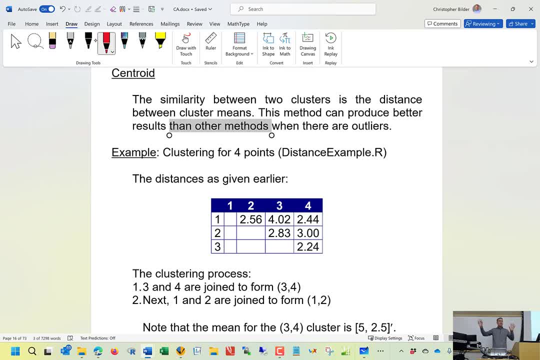 then find the mean value for another particular cluster. The distance between those two clusters then is the Euclidean distance between the two cluster means, And so you think of a mean as being in the middle. So that's why I say it's kind of in the middle between furthest and nearest. 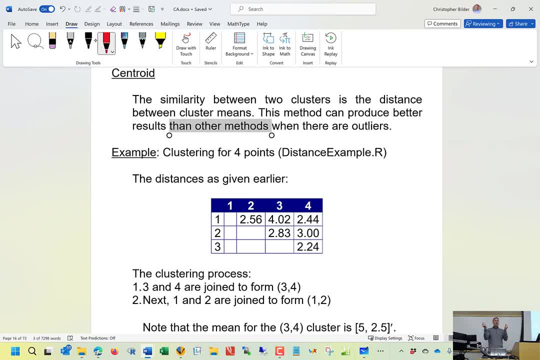 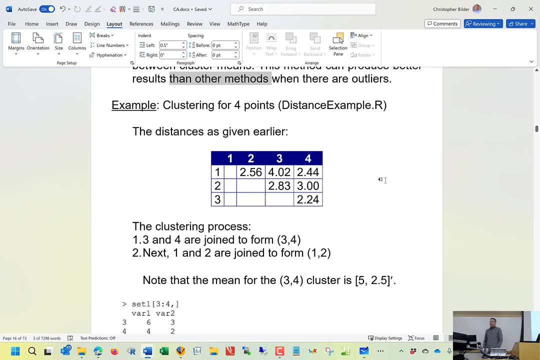 We're looking at the distance between the two cluster means to make a judgment of, or then to find then the distance between the two clusters. So let's take a look at an example of this. Here are the distances that we have for that four observation example again. 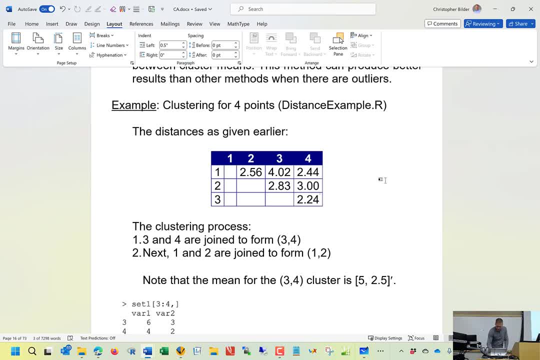 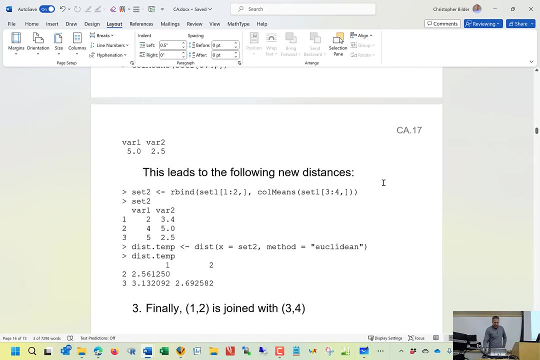 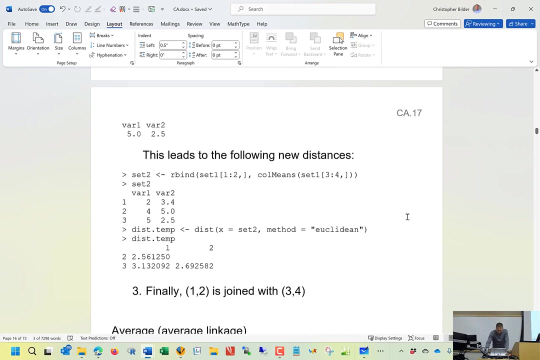 Once again, we're trying to find what's the smallest distance. That distance is 2.24, so observations three and four are going to be joined together. Now I need to figure out. I don't know why I didn't put it on a table like that. 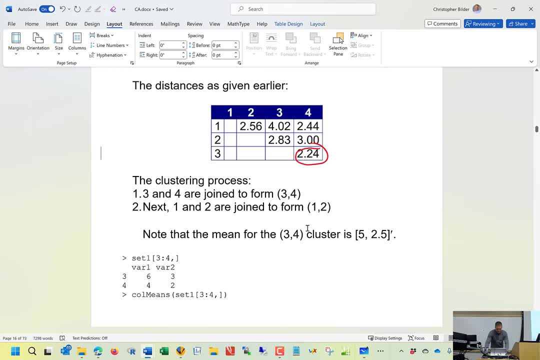 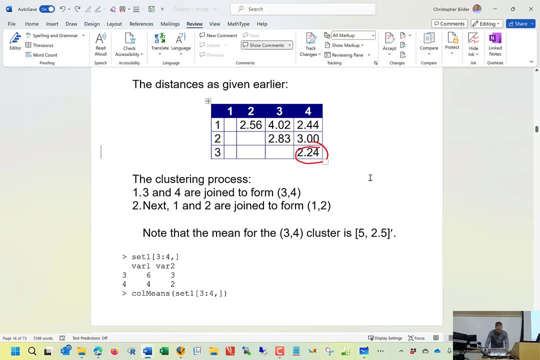 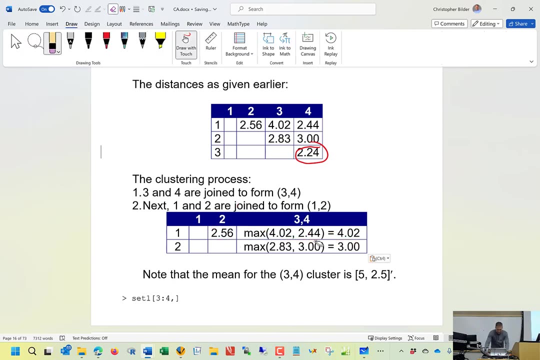 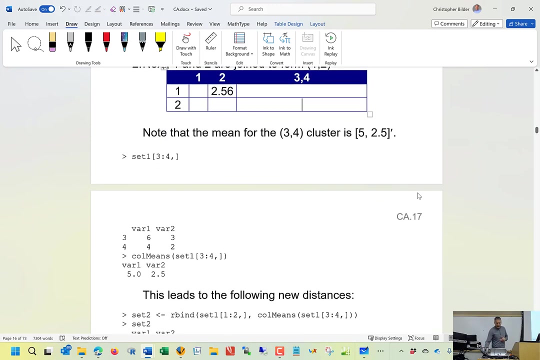 So three and four have been joined together, But now I need to find the distance between the cluster that has just one and then the cluster that has three and four. And so what that means then is I need to find, then, what is the central point of the cluster that has three and four. 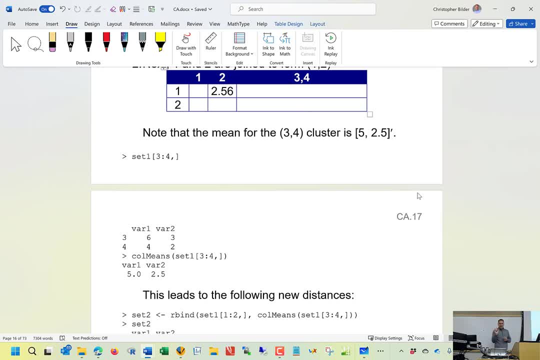 In other words find the mean between observation three and observation four, And so a simple way to do that is that here is observations three and four. I use the call means function To find just now the column means when I just have observation three and four. 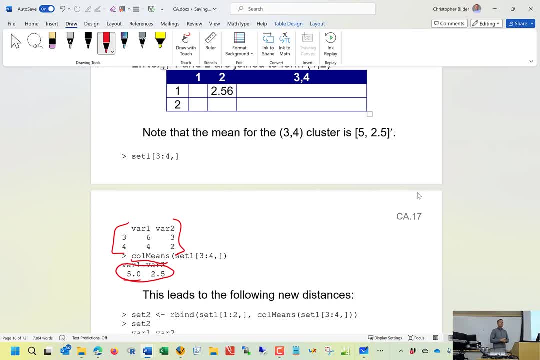 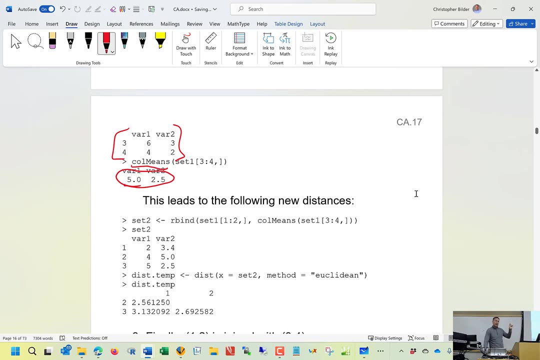 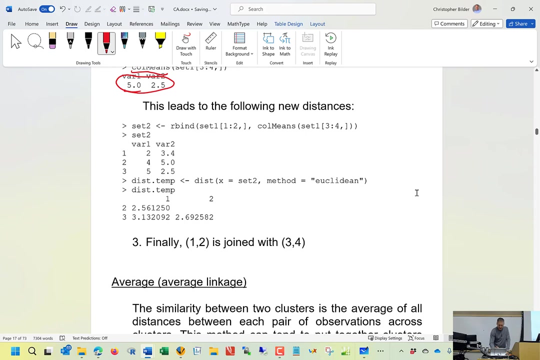 So that mean is five and 2.5.. Okay, So now I need to find well, what's the distance between observation one and something that has five for variable one and 2.5 for variable two. And so one quick little way that I did this was: 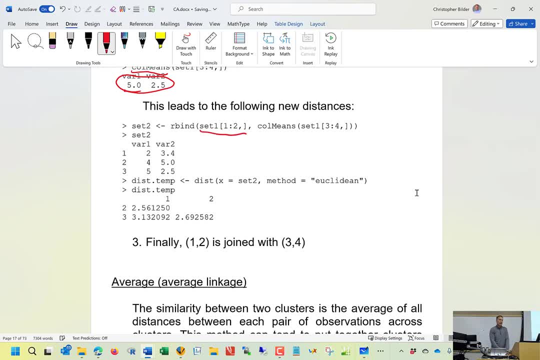 I took my first two observations that are in set one and then I combine it with those column, means that we just found, And so that now I have, let's say, a new little data frame that has all the the values that I want to find, the distances between 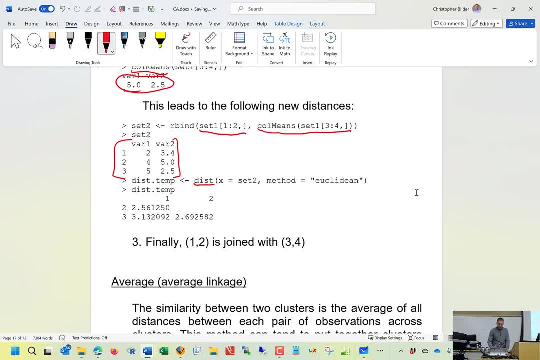 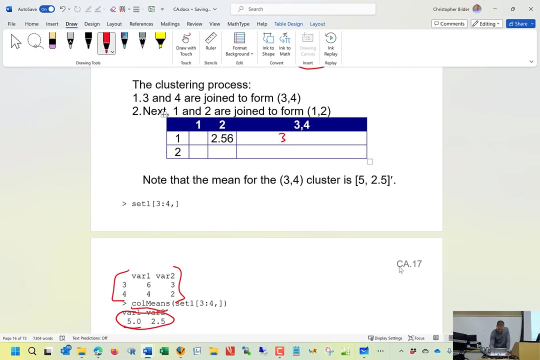 So I can put this back into dist and this is what I get. So the distance between- let's see now- one and the cluster that has three and four in it is 3.13.. The distance between observation two and the cluster that has three and four in it. 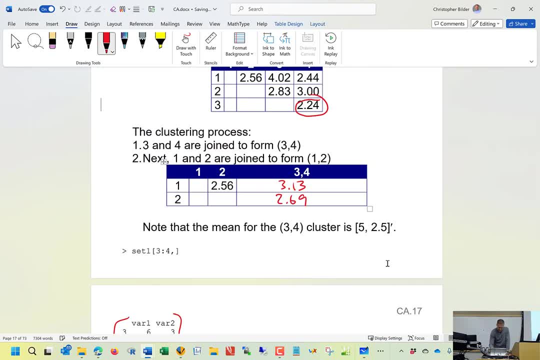 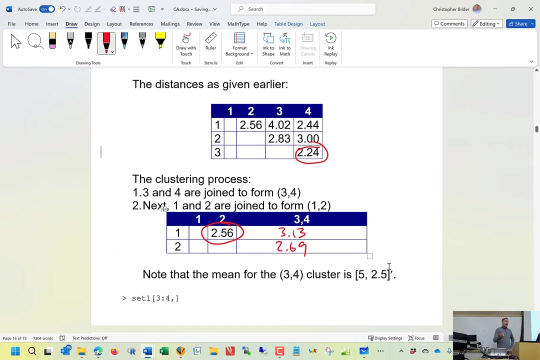 is 2.69.. I look at all those distances. I find the one that's the smallest. It's the 2.56.. So observation one and observation two are going to be joined now to a new cluster. So I have one more stage. 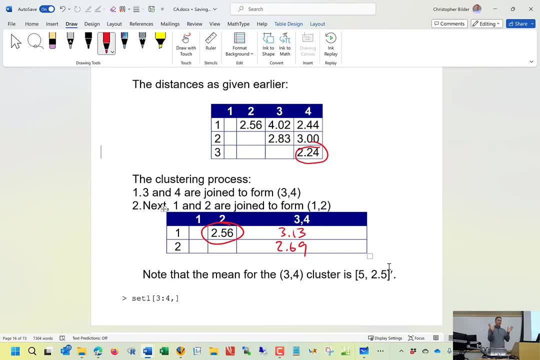 Of course, the cluster with one and two in it is going to be joined with the cluster that has three and four in it. How do I find the distance, though, between those two clusters? I find the mean for the cluster that has observation one and two in it. 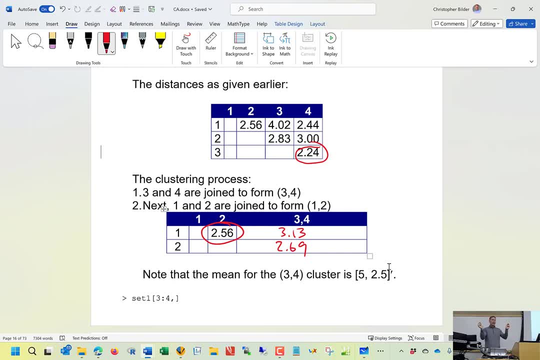 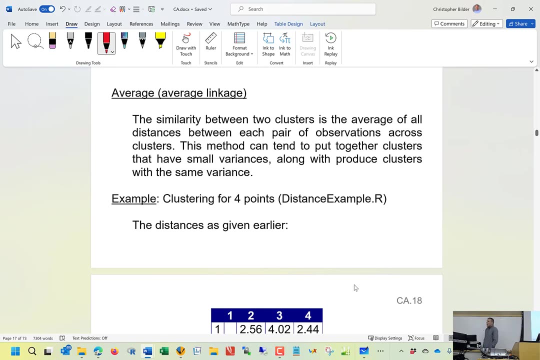 I find the mean that has the cluster, that has three and four in it, And I just simply find the Euclidean distance between those two. That's how you do it, Okay, So that's one way to think about being in between furthest neighbor. 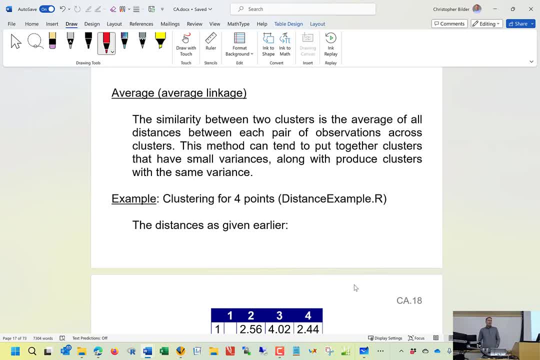 and nearest neighbor. Here's another way We can use what's called the average method. Now note: we just found some averages, So you have to be very careful about these names and what they actually represent. This is a different way of finding averages. now. 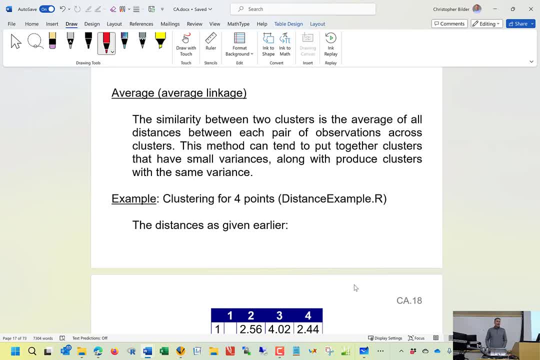 What we could do instead in this particular case is how about we look at all the distance between, let's say, this cluster and this cluster? Look at all those distances and find the average distance. So maybe I have a total of ten different distances between these two. 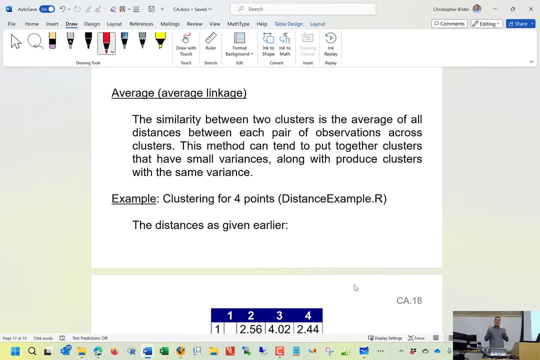 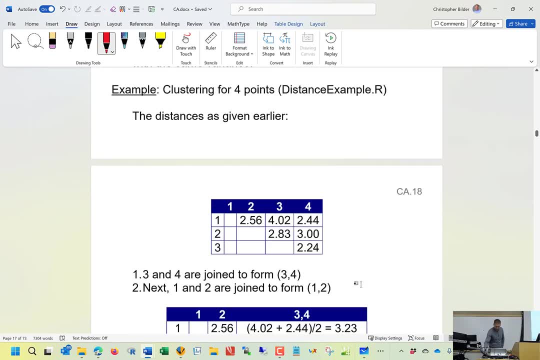 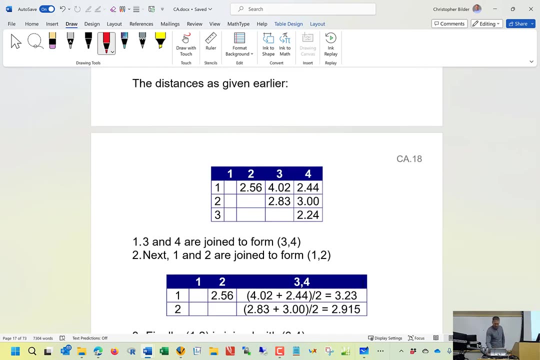 Just find the average of those distances And that's going to be now the distance between this cluster and that cluster. So let's go through the steps. So again, I start off with this table. here, Observation three and four join together because it's the smallest distance. 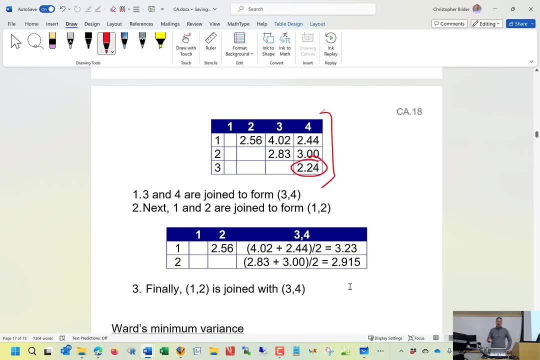 Now to decide what I'm going to join next. distance between one and two does not change The distance between observation one, and the cluster has three and four in it. Well, what I do is I find the distance between one and three, I find the distance between: 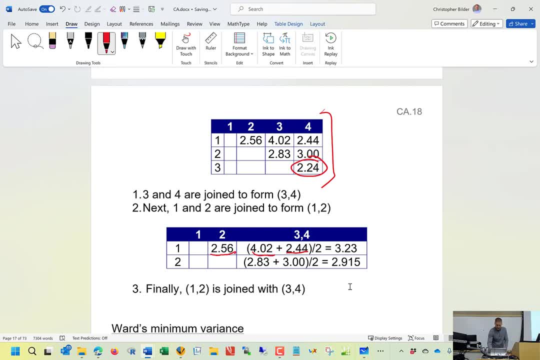 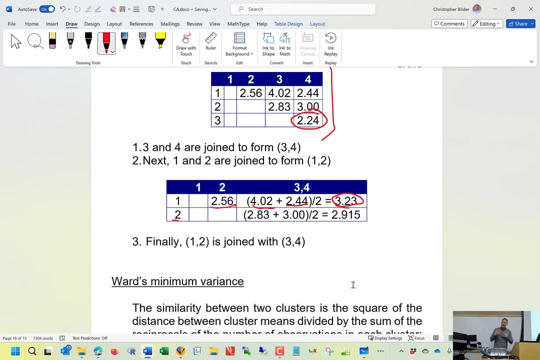 one and four. The average distance then is 3.23.. In a similar manner, I find the same way of finding the distance between two, and the cluster has three and four in it, And I get 2.915.. Again, the smallest distance here is 2.56.. 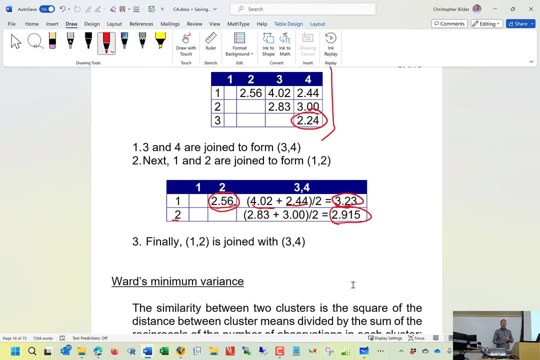 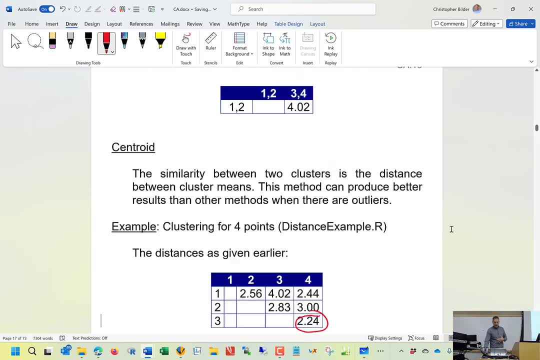 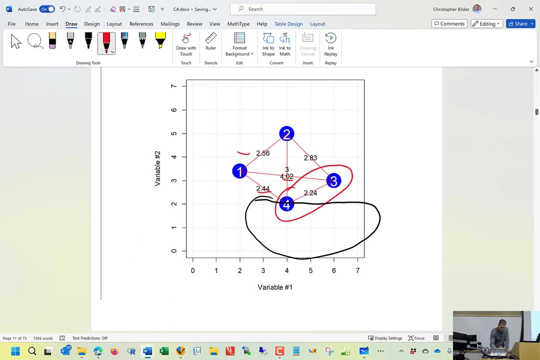 So I'm going to join cluster one and two together. In the end, I'm going to have a cluster with one and two. I'm going to have a cluster with three and four. What's the actual distance then between these two clusters? 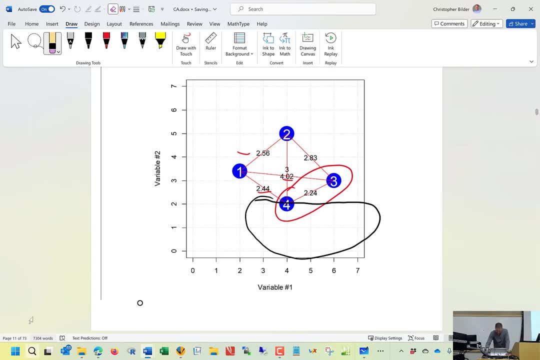 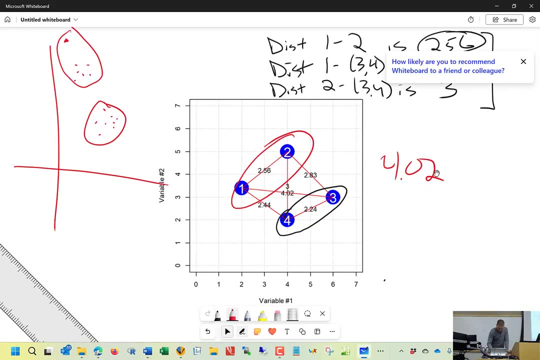 I'm going to come back up to my ah. I'm going to come back to the whiteboard. That's not working. Let me get an eraser. So I need to. so this is the two clusters I have And I need to find now the distance. 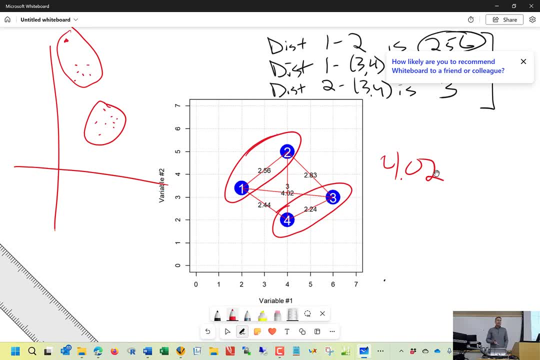 between these two clusters. What would I need to do? The average distance, but basically all the numbers that you see on here for all these distances. well, let's well, let me put it this way- I'm going to highlight the distances that I would use. 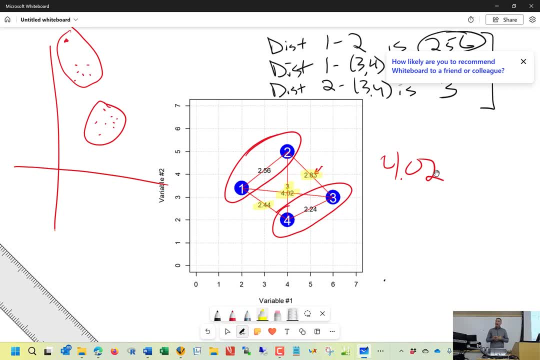 to find that distance. So I would take the average of those highlighted yellow numbers. I would not take the the distance between one and two because that's already one cluster. I would not take the distance between three and four on this average because it's already one cluster. 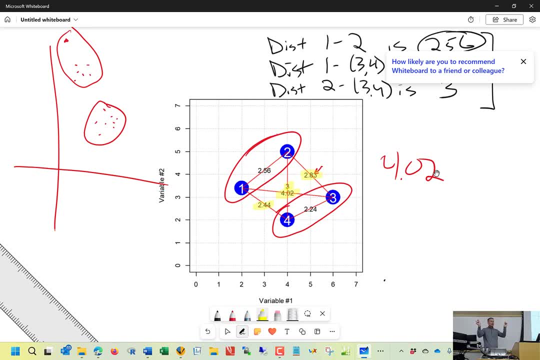 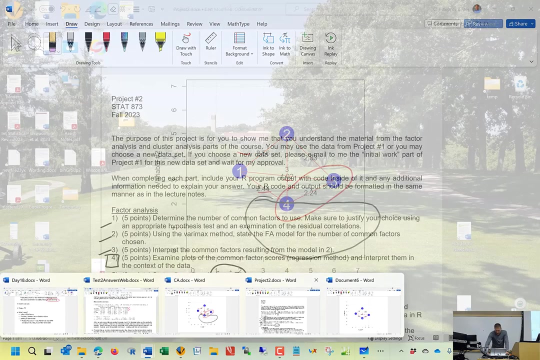 It's all the distances between the observations in the two clusters. Those are the ones that are average. So the average of that would be my distance between the two clusters. Any questions Now, overall, using the average method, using the centroid method, 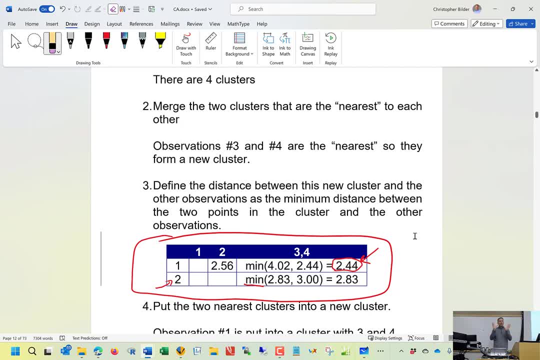 you can often have more, let's say, compact clusters than you know what we saw with the single link with the nearest neighbor, single linkage. You know you have these elongated clusters. You know obviously outliers are not going to be. 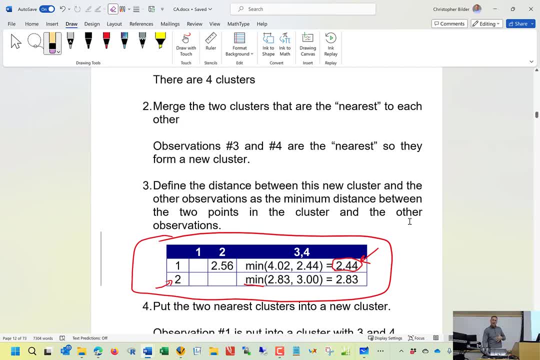 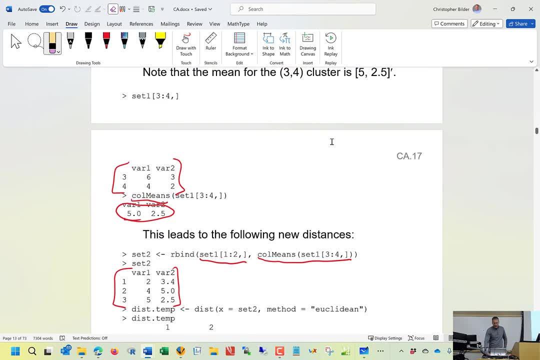 playing as much of a role, so you're not going to have the problems that the furthest neighbor can have. And so those are some advantages of using the average method, the centroid method. But you might be thinking, well, why don't we just use those then? 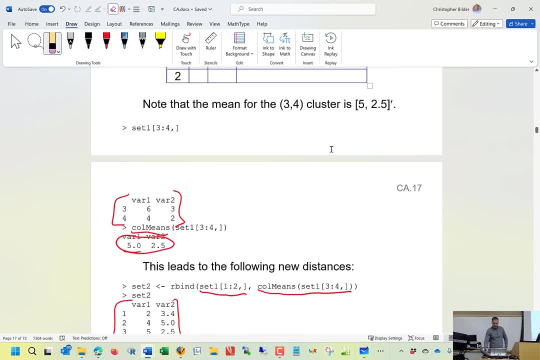 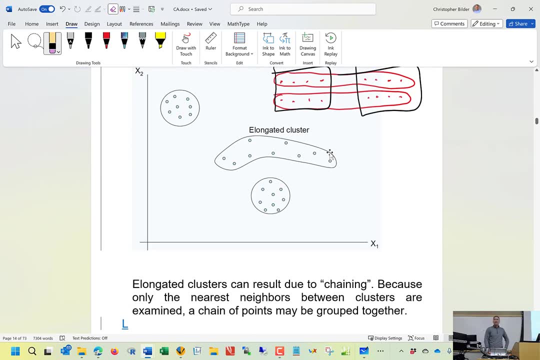 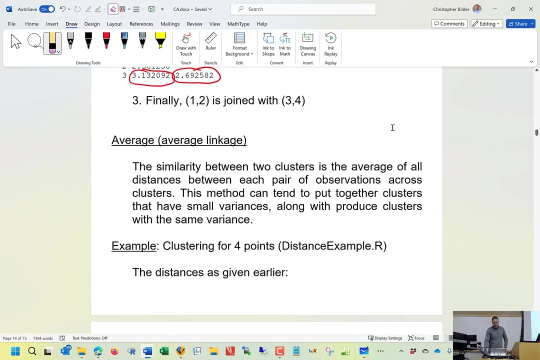 since you just talked about averages, Well, maybe there might be times where you want something like, something like that, Okay, And the average method and centroid method might not work as well in those situations. So what ends up happening in practice? what you typically do. 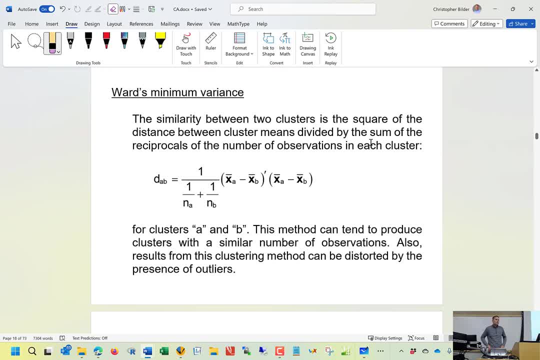 is you use more than one clustering method and then using some tools. well then, you're going to use some tools to make a judgment of do these clusters make sense? So just to give you an idea of what we will do, is that we'll use 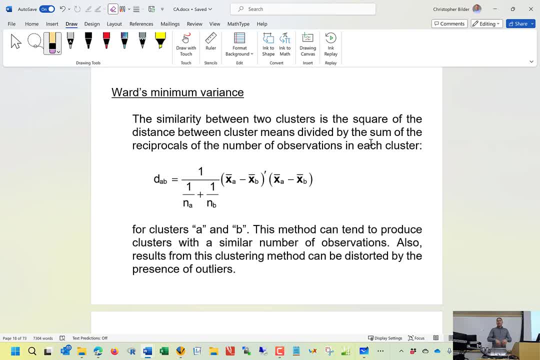 principal component analysis to you know, find, you know, some principal components that account for a large percentage of the variation of the data plot, the scores, and then also, let's say for the, for the plotting point, have that correspond to the cluster. 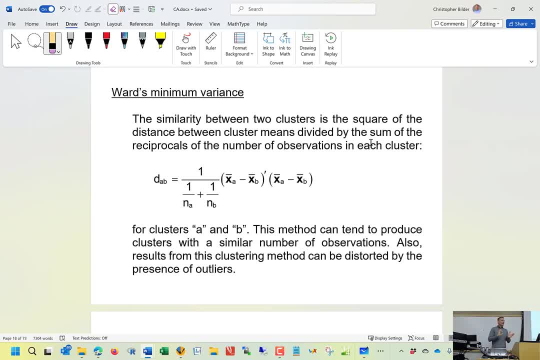 Like, if it's cluster one, is it cluster three, is it cluster five? And look at the principal component you like, think of like a if you have two principal components, think of a scatter plot of the scores And if the observations are nicely grouped, 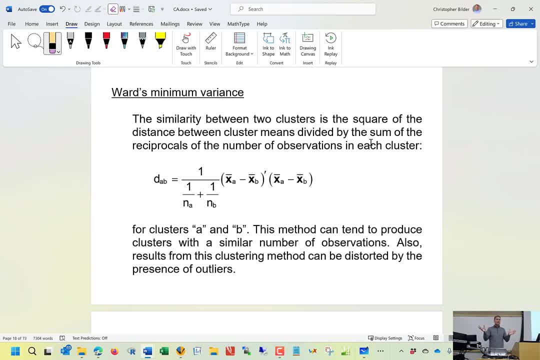 then okay, you're satisfied with that clustering method. If they're not, like you know, if you have, let's say, two observations that are really close to each other on the plot, but yet they're in two different clusters. 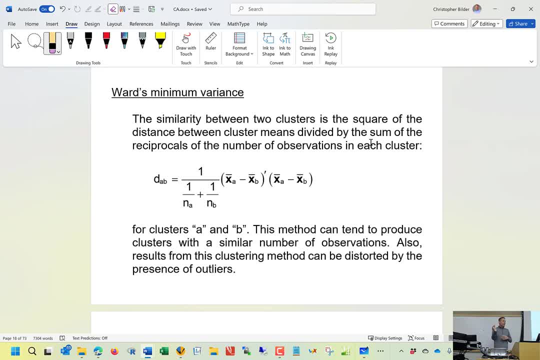 and you might be. then that calls into question: did this clustering method work? well, We'll get to that. Lastly, there's another- sometimes you see this used, I see this used a lot less- Another clustering way of, another way to do agglomerative. 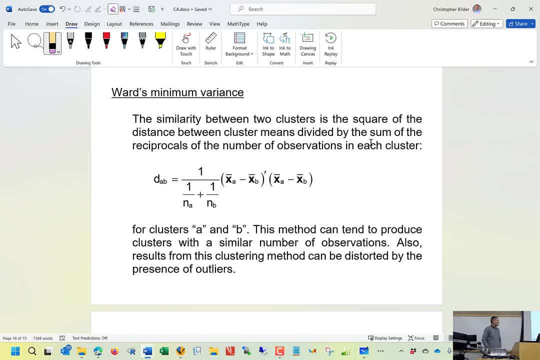 it's called Ward's Minimum Variance, and here you just redefine how you do the distance between the clusters by using this: N sub A is the number of observations in cluster A, N sub B is the number of observations in cluster B, and then we have corresponding cluster means. 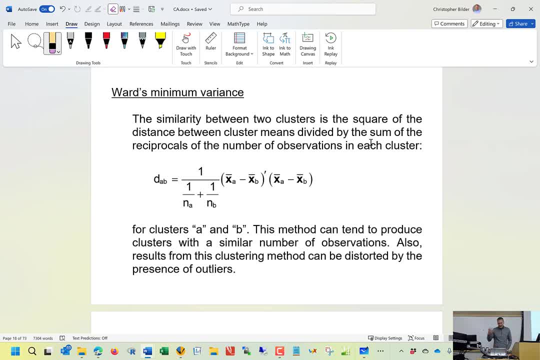 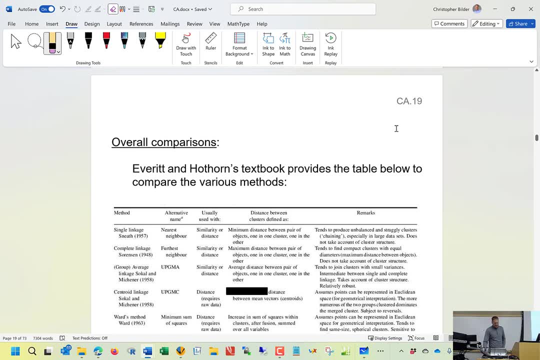 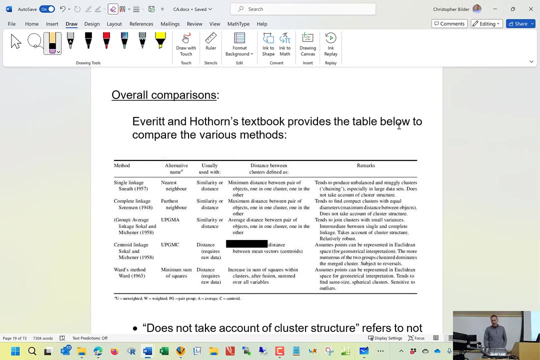 similar to like centroid method and some people will use this. On page 19 of my notes, I just basically took a table that is from one of the recommended books for this course. that talks about a lot of the stuff that I just talked about. 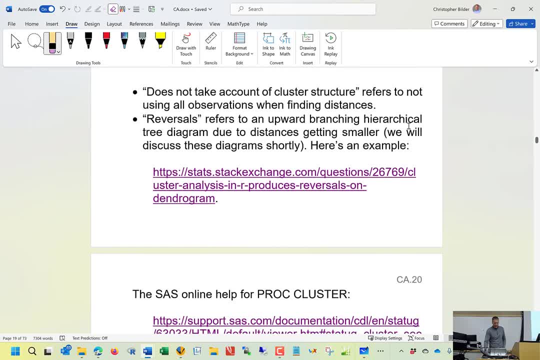 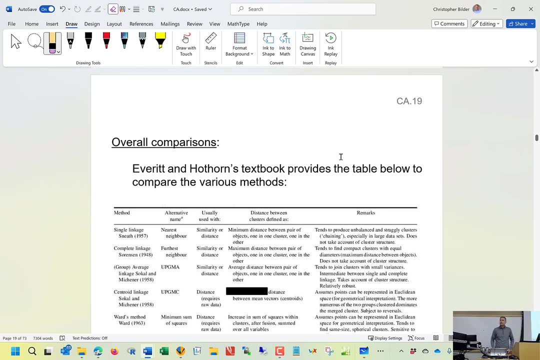 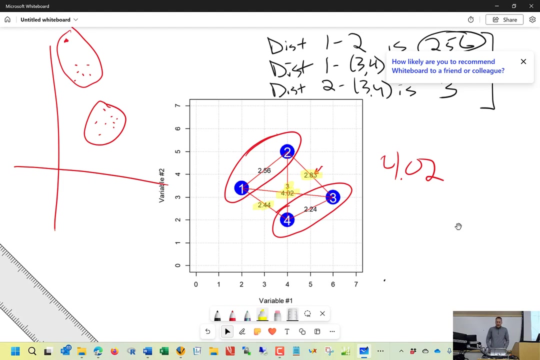 in terms of comparisons amongst the methods. You're welcome to take a look at that. Another question is: you said, finally, we join the two clusters together. Well, I understood that with the averages, we took the averages for like, We took the averages of those yellow. 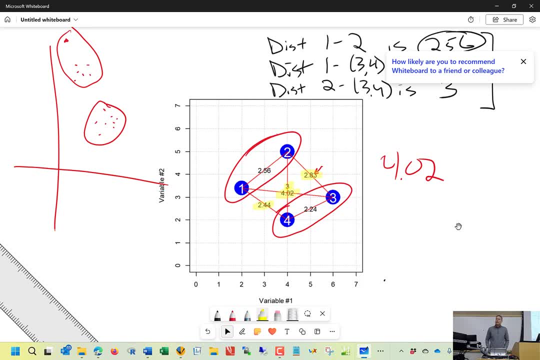 Yes, so now how do we like decide whether to join them or not to join them? because the averages are we going to look at, maybe the smallest averages, or maybe we can decide to separate clusters. Yes, I guess I'd say, stay tuned for that. 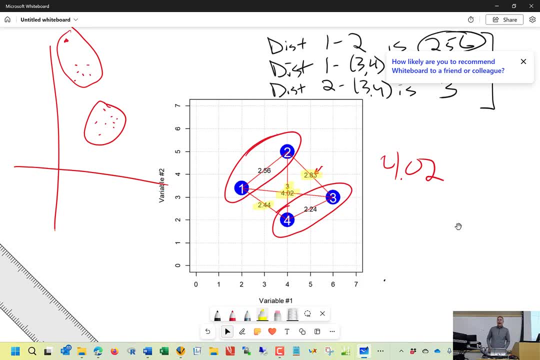 I will talk about how we make that decision. Would we actually want to do it? But the way that these clustering methods will work is that you will go all the way to having just one cluster and then, once we've done it, then we go back and think: 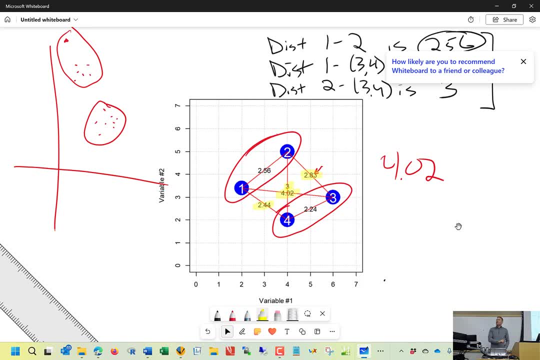 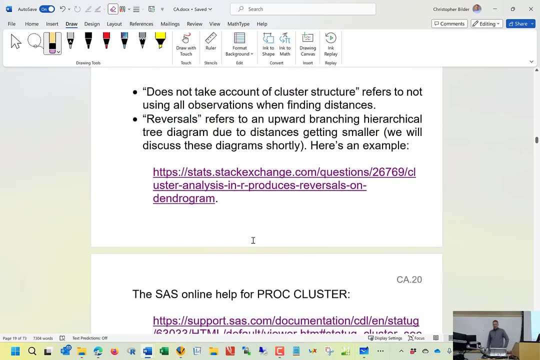 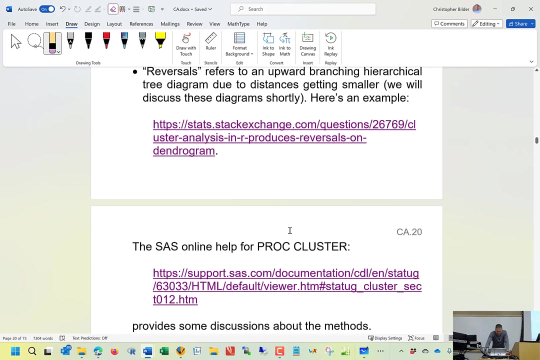 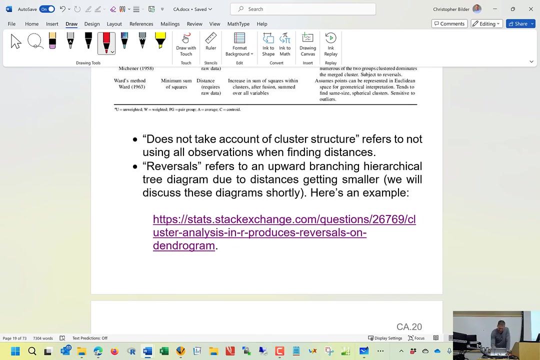 okay, did I really want to go to one? Maybe I should have stuck with two. Okay, so we will get to that. I'm going to get ahead of myself here. I guess I can talk about this here. When we're looking at tables like this, 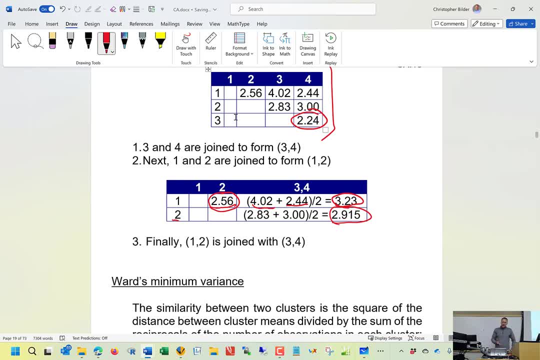 where we have these distances. you would expect that as you go from, In our case, we have four clusters, then we go to three clusters, then we go to two clusters, then we go to one cluster. You would expect that these distances 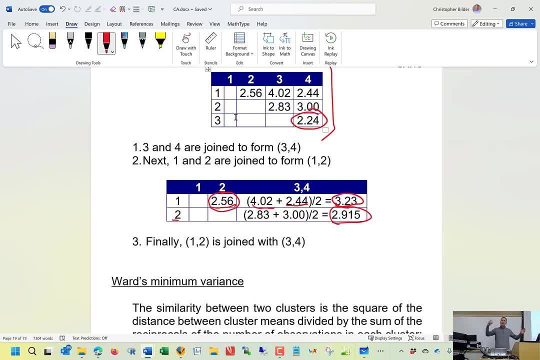 between clusters would increase as you get to a smaller number of clusters. and that makes sense, especially for like single for the nearest neighbor method, because as you're joining clusters now, the observations are going to be farther and farther and farther apart as you continue to. 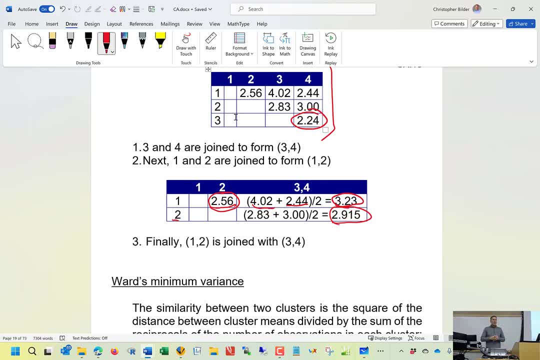 reduce the number of clusters. Some of these methods, though, can have what are called reversals. What that means is that the distances can actually decrease as you go from, let's say, from three to two clusters. Compare that from three. 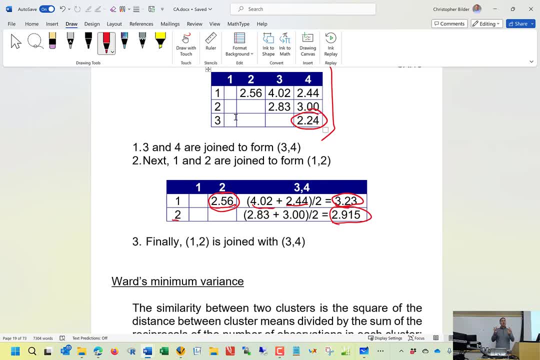 Compare that from two to one. The distance from two to one could be smaller than it is from three to two. That seems counterintuitive, But because of how these distances between these clustering methods, or the distances between clusters, are actually computed for like a centroid and an average. 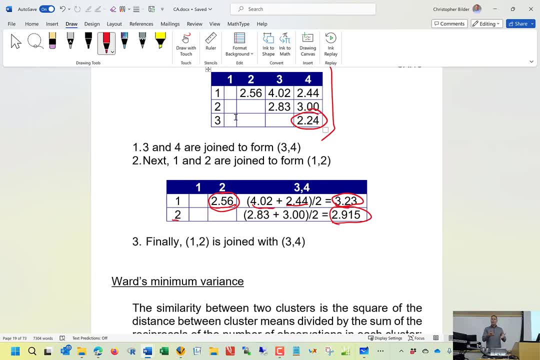 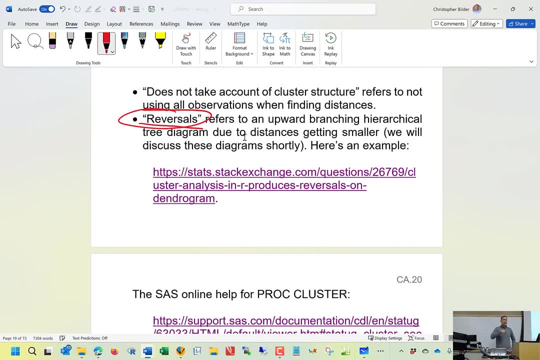 that can actually happen. I'll talk more about that later. As I'm going through my notes here, not actually doing this in a class, it's like, well, maybe I should have held off on that, but we will hopefully come back to that. 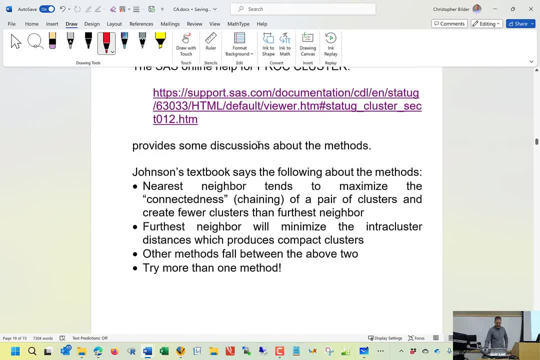 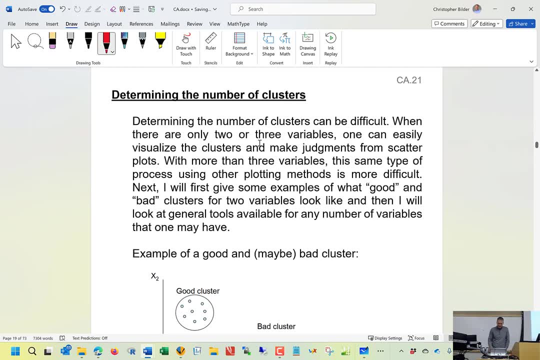 and see a nice plot that shows how that can happen. Okay, So the next part here is determining the number of clusters, And then we'll get to the question. but well, maybe I should just stop at three versus go to two, Going through all these methods. 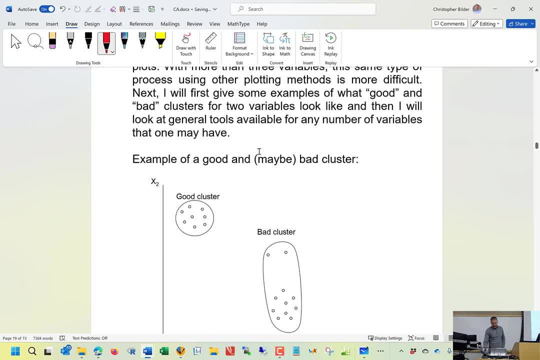 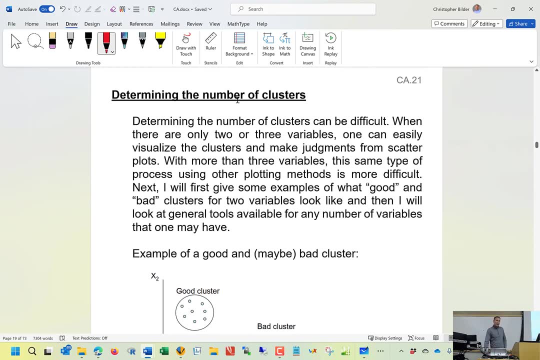 has taken a lot longer than I anticipated, And we're about at the end of class right now. So next time we will talk about how do I decide how many clusters I actually want. So let's take a look at then what's next for our course. 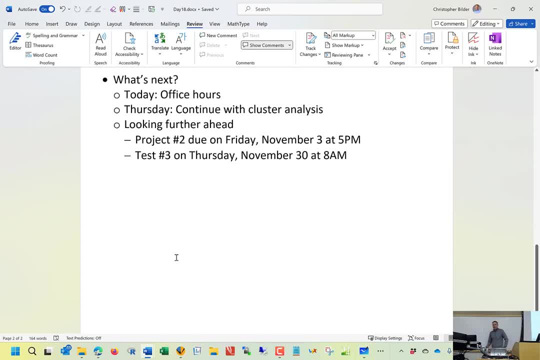 So I have office hours after our class. Thursday we will continue with cluster analysis. Again, project number two has been moved back two days And then, just looking farther ahead, test number three is Thursday, November 3rd. So are there any last questions?